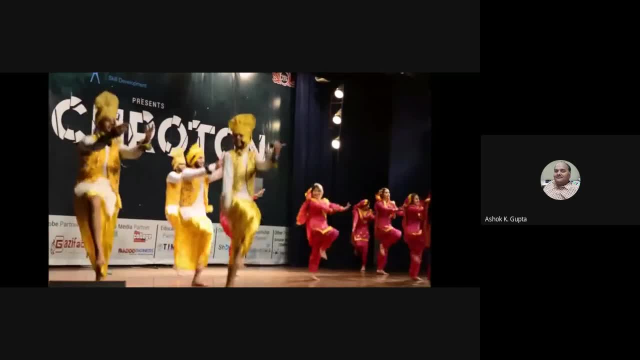 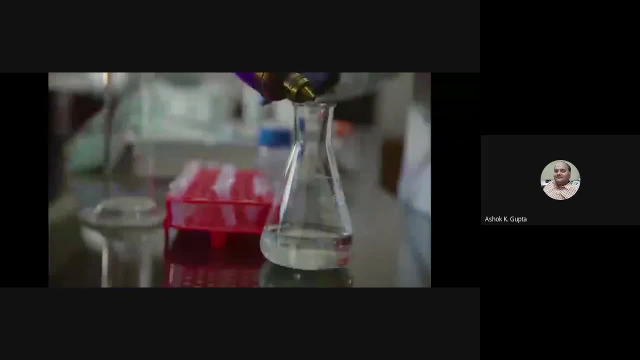 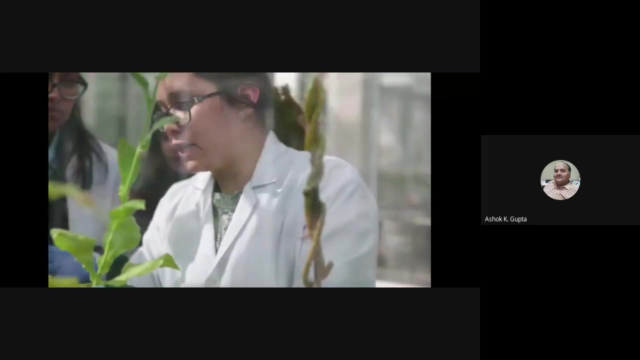 festival called Padukram, literally festival and cultural festival, which further heightens their energy levels. They're also encouraged to develop independence and thought and action, as well as trained to deploy appropriate technology paradigms for given tasks, Explore new horizons and lead teams to solve complex problems With our learner. 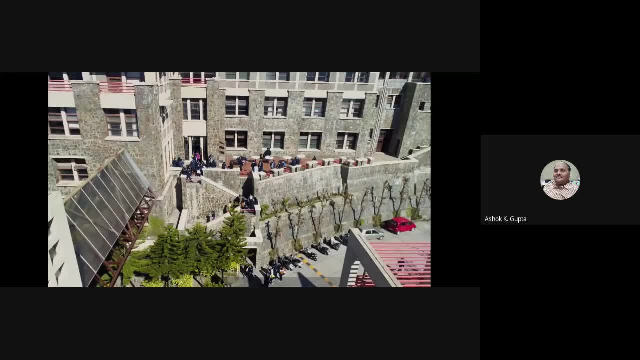 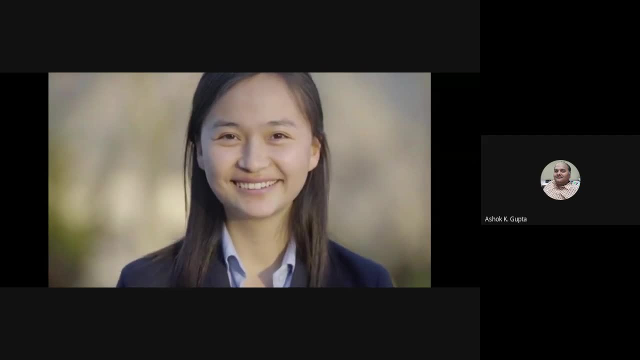 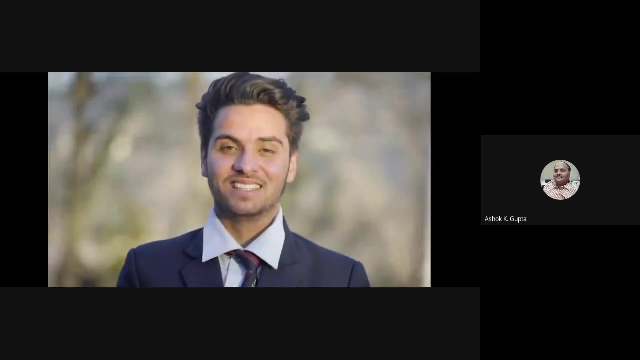 eccentric educational process. students are free to find their own paths and learn their way to limitless opportunities that awaits them. So be a part of JP University of Information Technology Vagnekant in Machu Parish, to be the leaders in innovation, entrepreneurship, creativity and 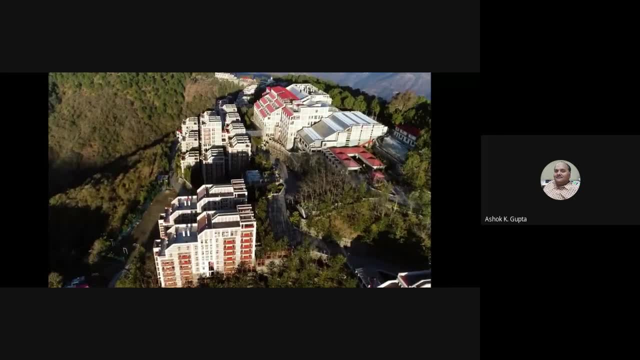 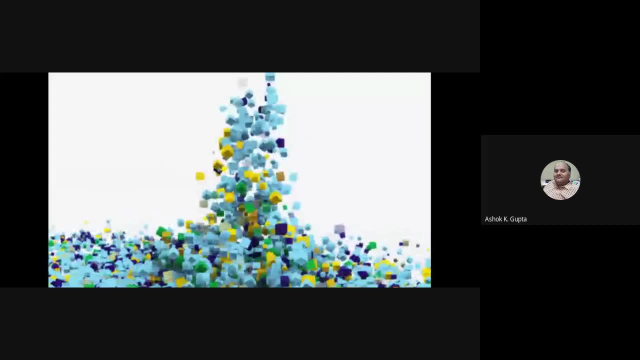 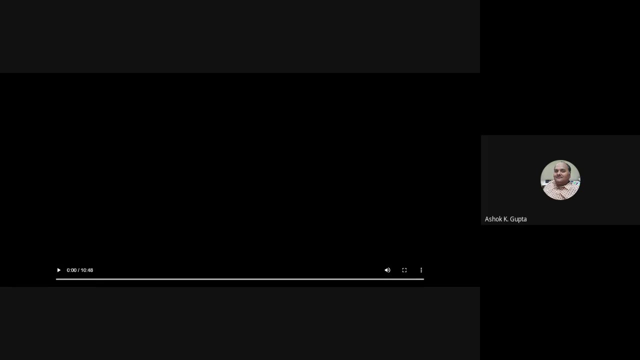 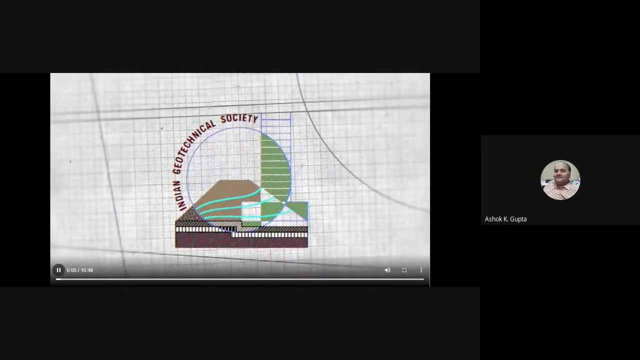 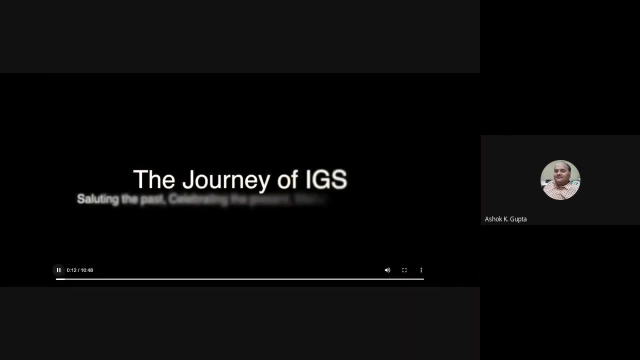 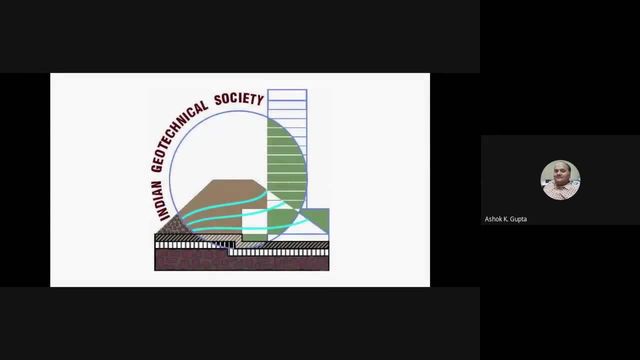 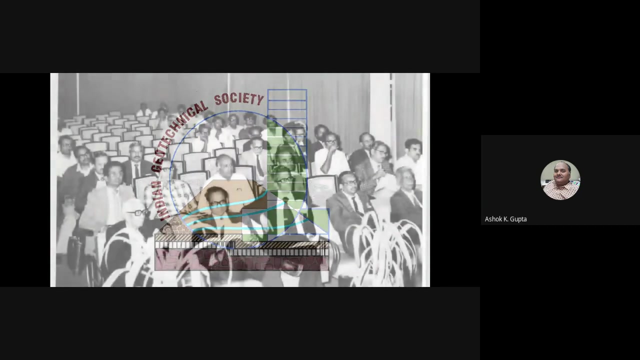 management, Because this is where we engineer lifelong learners. The Indian Geotechnical Society, which was earlier known and founded under the name of the Indian National Society of Soil Mechanics and Foundation Engineering, was established in 1948. This came soon after the second international conference. 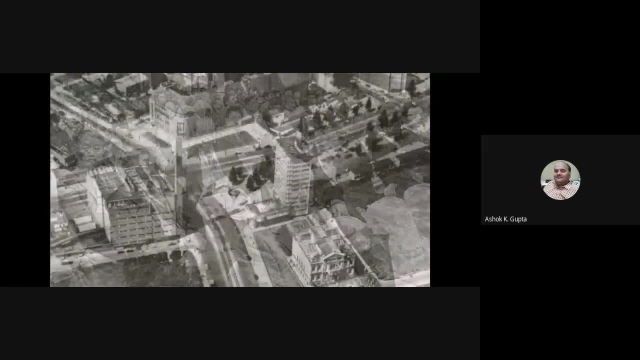 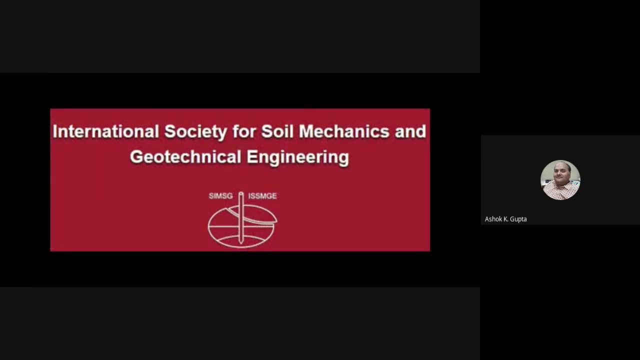 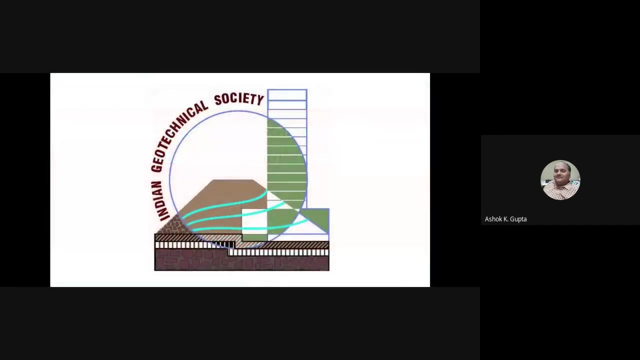 on soil mechanics and foundation engineering held in Rotterdam. The society was affiliated to the International Society in the same year and since then it has strived to fulfill and promote the objectives of the International Society. The name Indian Geotechnical Society was adopted in 1970. 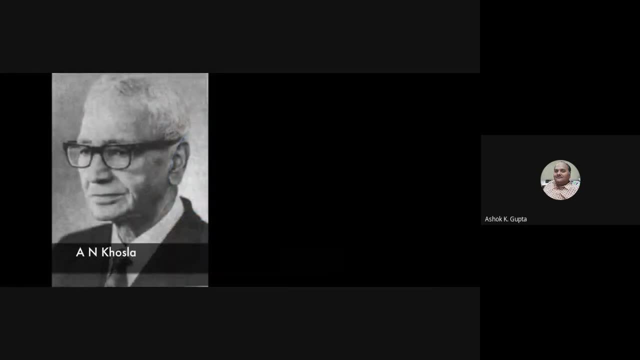 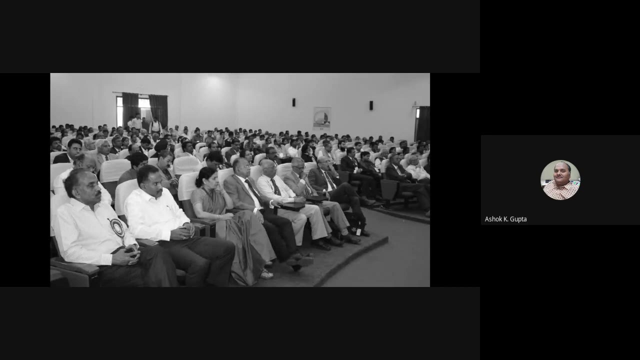 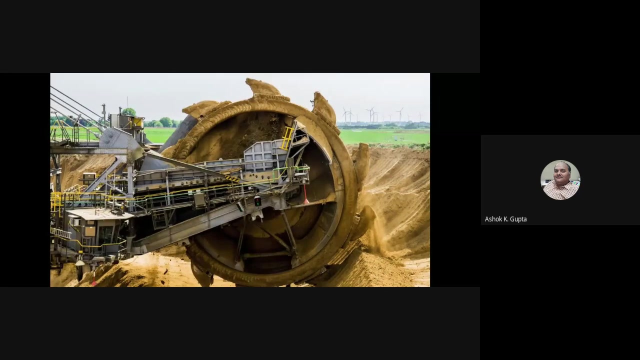 The vision of the founding president, Mr Khosla, and the honorary secretary, Dr N D Gulati, was to build the society, to promote cooperation amongst engineers and scientists for the advancement and dissemination of knowledge in the fields of soil mechanics, foundation engineering. 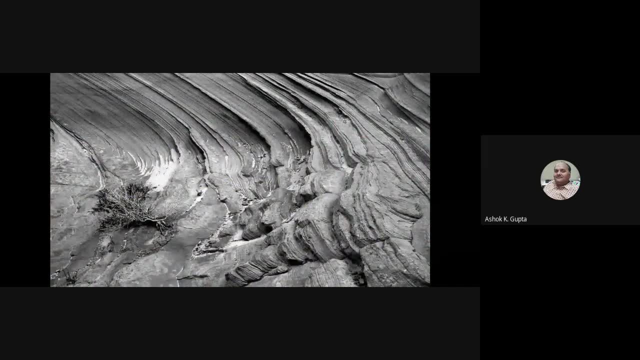 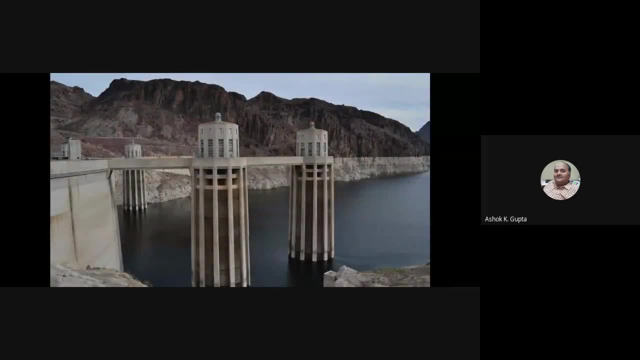 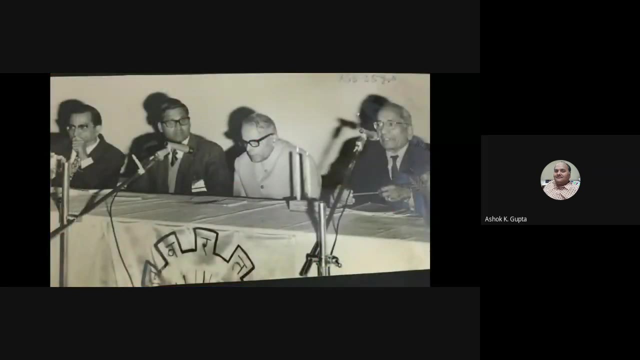 soil, dynamics engineering, geology, rock mechanics, snow and ice mechanics and allied fields and their practical applications. As the geotechnical community started to grow, the International Society decided to have regional conferences for each continent, along with having four yearly international conferences. 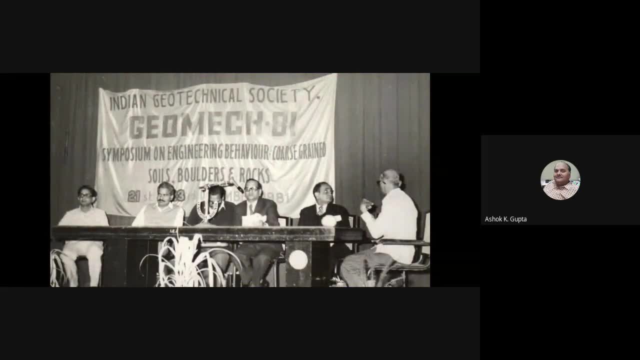 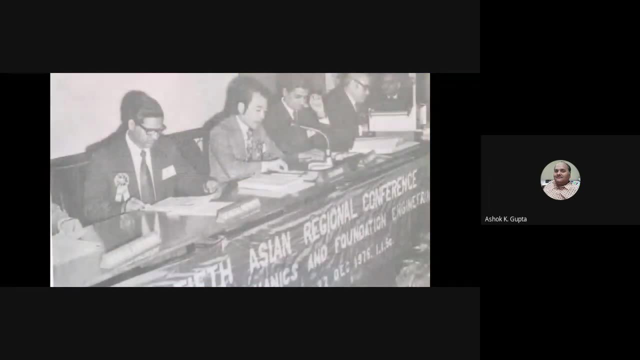 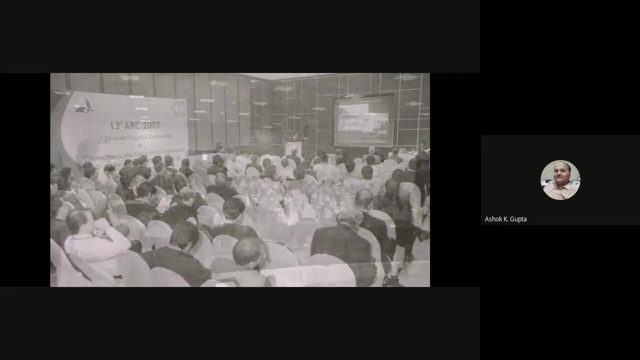 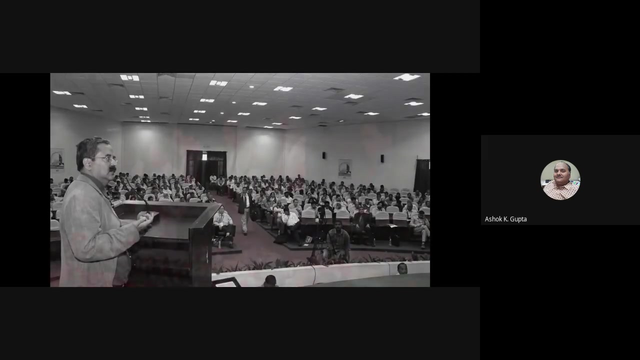 This is when the first Asian Regional Conference was held in 1960 in New Delhi. India also hosted the fifth Asian Regional Conference at Bangalore in 1975 and the thirteenth one at Kolkata in 2007.. IGS has been organizing national conferences annually in different cities since 1961.. 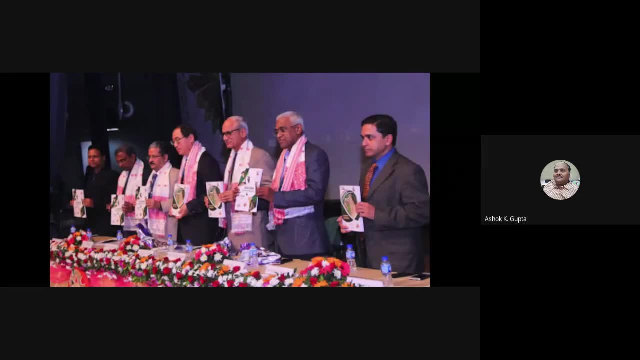 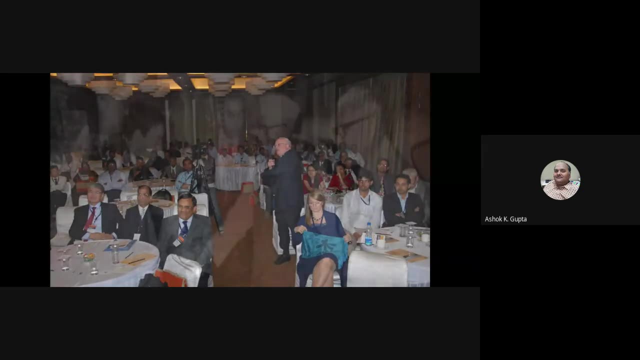 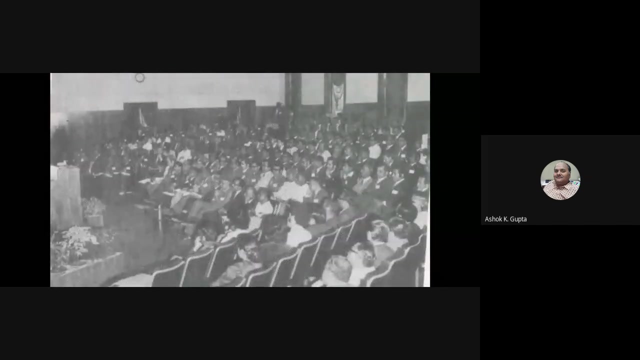 The Silver Jubilee Conference was held at Kurukshetra in 1973.. The 1978 Geocon was a landmark conference held at IIT Delhi, which was inaugurated by the then Prime Minister, Muraji Desai. IGS started the prestigious annual lecture in 1978. 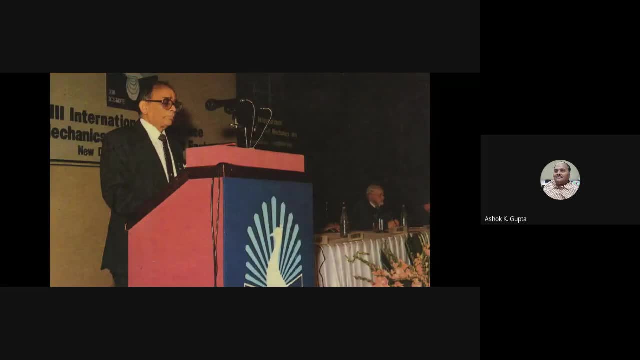 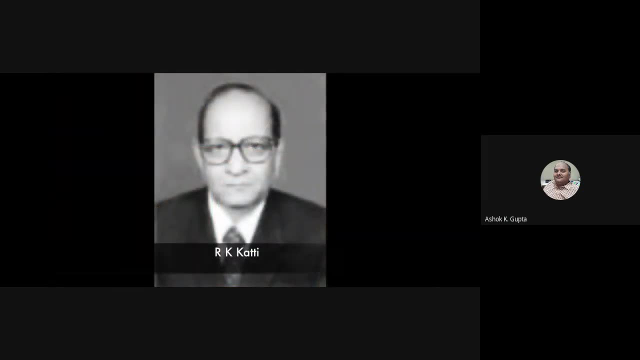 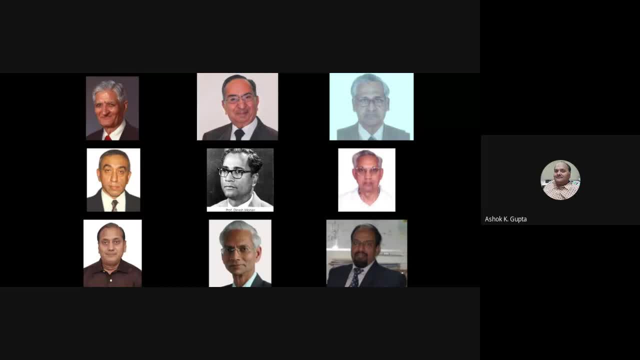 Prof D S Mohan, Prof D S Mohan, Prof D S Mohan, Dr R K Bhandaari, Professor Gopal Ranjan, Dr B G Rao, Dr N V Nayak, Prof G V Rao, Prof A V Shroff and most. 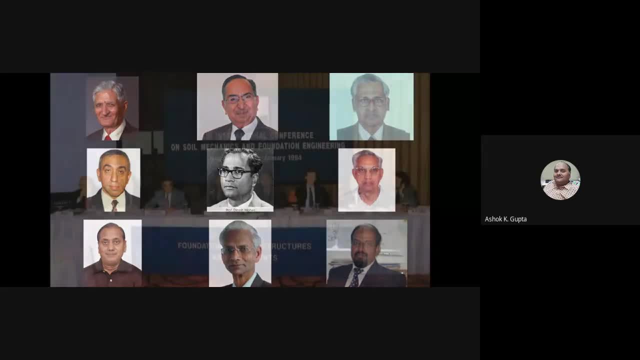 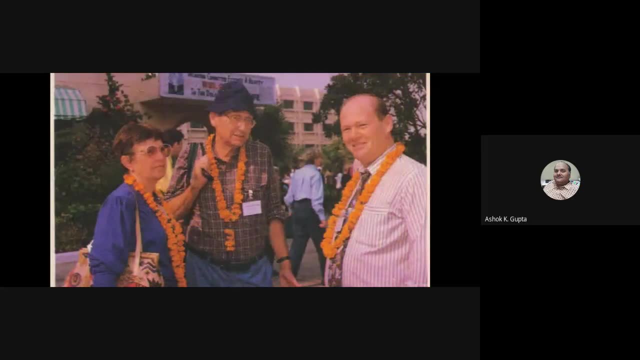 recently, Prof M N Vilatkar IGS made an impressive debut in the international scene in 1994 with the organization of the 13th International Conference on Soil Mechanics and Geo- Kunsttechnische Ausbildung in Geotechn, sutieren. 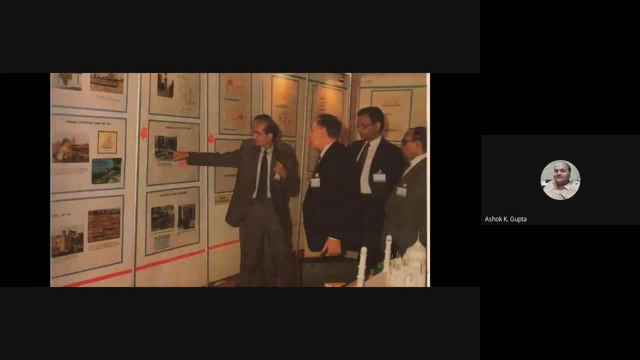 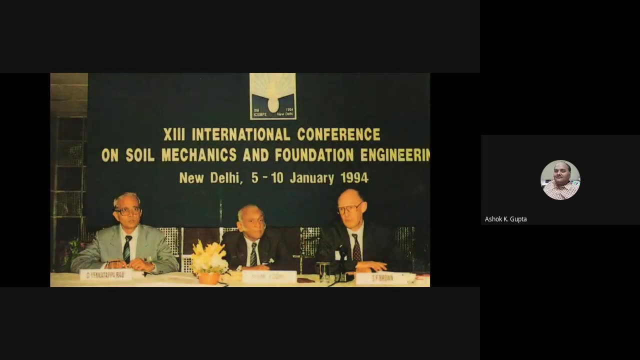 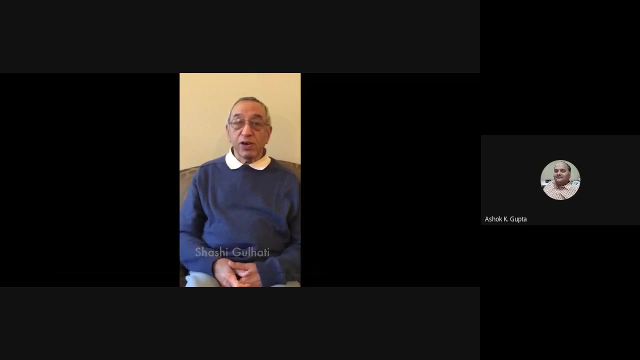 von des cubedischen Feuerwerk und geotechnischer Unterricht inspection- that was a remarkable- was held in New Delhi. This was one of the biggest conferences in the history of the International Society and it firmly put India on the international map. Two dozen years ago, in 1994, the Indian Geotechnical Society organized 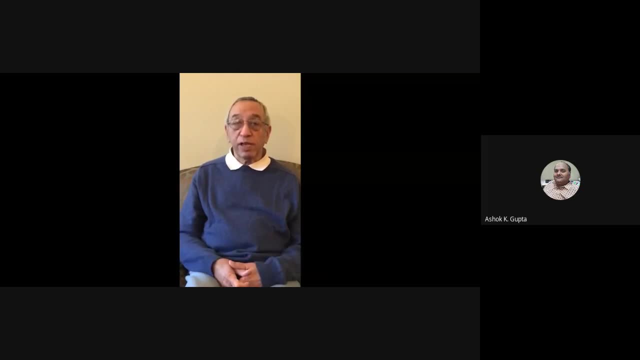 the 13th international conference on soil mechanics and foundation engineering in New Delhi. This conference was a great success. Everything went perfectly as planned: Its technical sessions, its exhibition, its field trips, its delicate interaction, its companions program, its entertainment and. 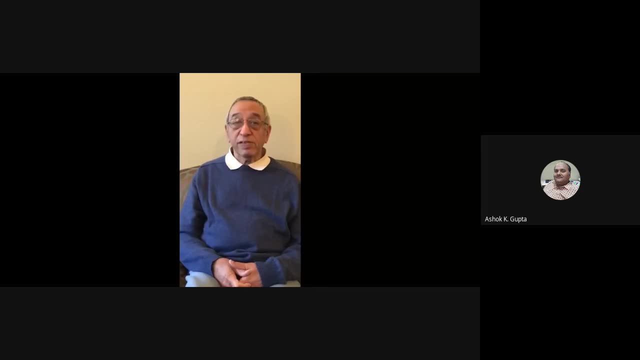 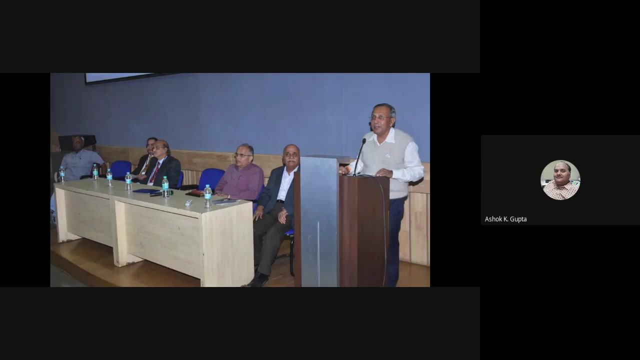 hospitality. Dr Parry, the Secretary General of the International Society, in his concluding remarks branded the conference as the magic carpet conference. The turning point came from the 12th annual research and development conference in New Delhi. This was a regional conference in Singapore which saw more than 20 Indian participants and 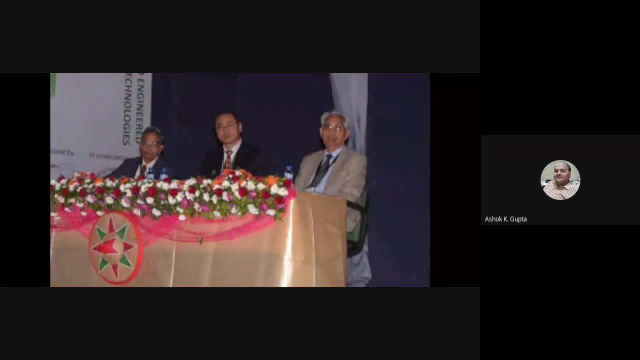 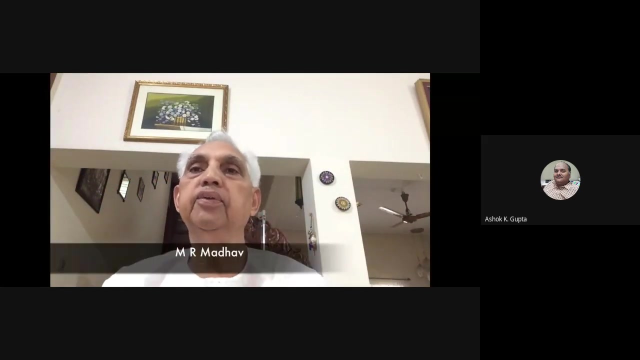 the keynote lecture by Professor Madhav. We were successful in winning the next ARC at Kolkata and also Professor Madhav as vice-presidentship for Asia for the term 2005 to 2009.. The major visible contributions from Indian Geotechnical Society: 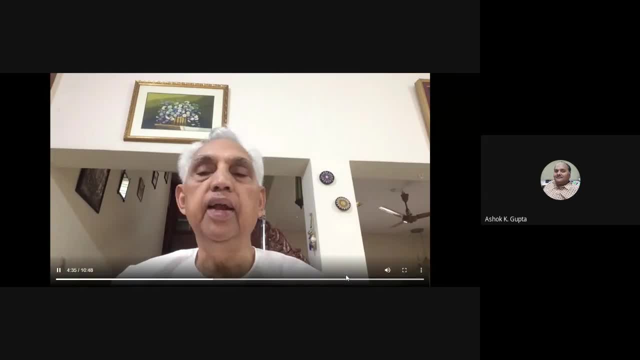 have been in the latest 21st century. A large contingent had been presented in 2017, but has not been told how it was in 2010.. In 2013,, the Singapore Asian Regional Conference followed by election of Professor Madhav as the next vice president. 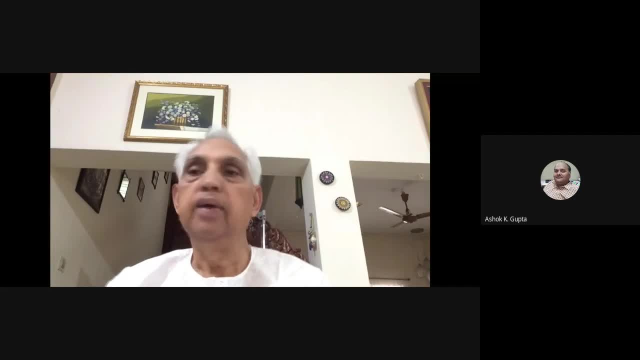 for the term 2005 to 2009.. Several of our members of the IADIS have been members of the Technical Committee. The most recent achievement of our Society has been the keynote lecture, or keynote lecture, given by Professor Madhav. We were looking forward to its arrival First. 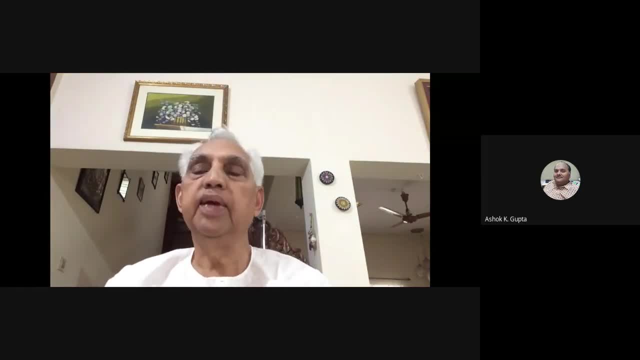 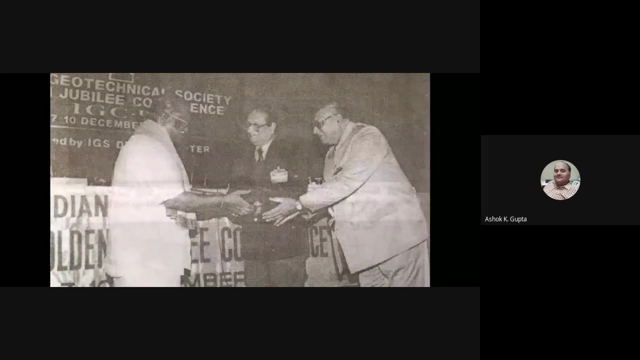 was a Babu at the Seoul International Conference. With the kind of enthusiasm and activities of the Indian Geological Society and its members, I look forward to a much more greater role for IGS in the international community. The Golden Jubilee Conference was held in 1998 at Delhi. IGC has hosted the council. 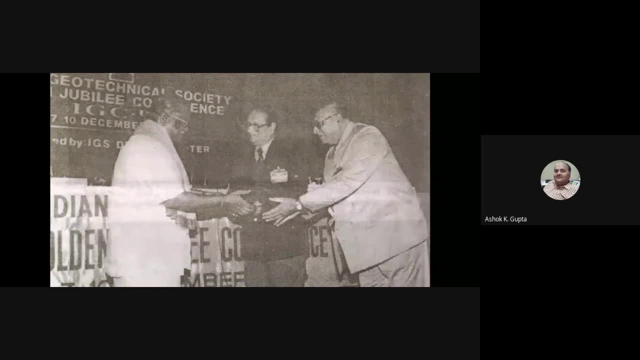 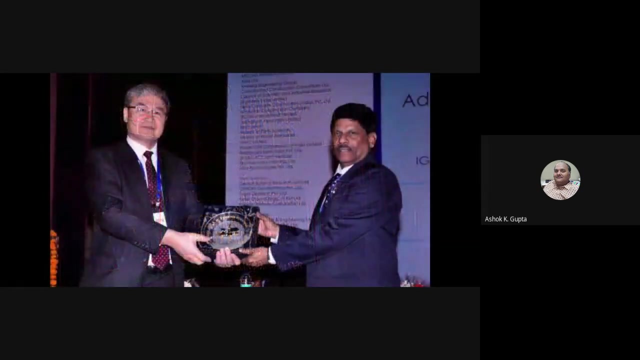 meeting of ISS MGE at Bangalore and the 6th Asian Young Geotechnical Engineers Conference very successfully. thanks to great efforts by Professor Sitaram, Professor Srinivas Murthy and the team, IGS was successful in bidding for the 6th International Conference on Environmental. 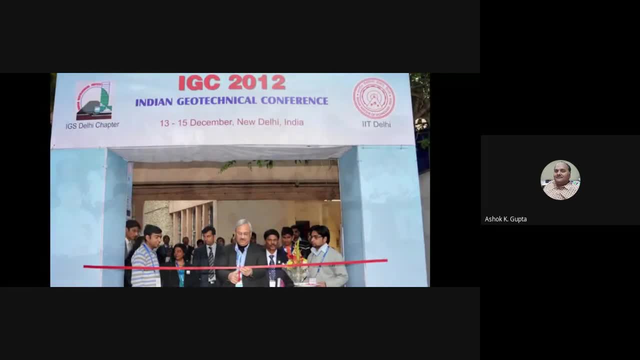 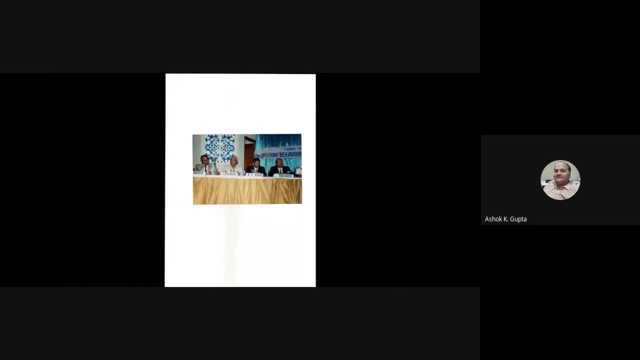 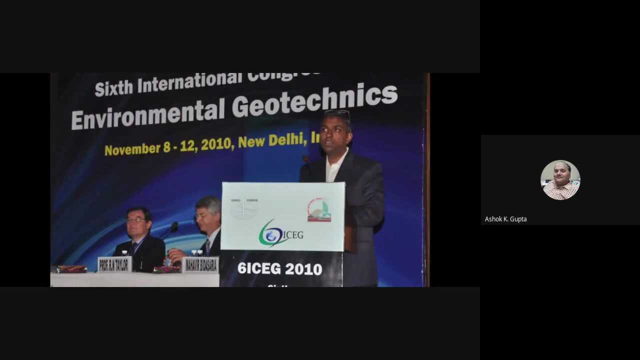 Geotechniques to Delhi in 2010,, which was a great success with, due to Professor Manoj Dutta's great efforts, The international community has become aware of our true potential, with several of our members becoming active in several technical committees of ISS, MGE. 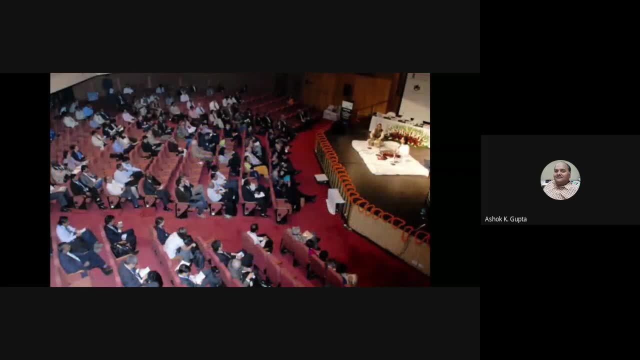 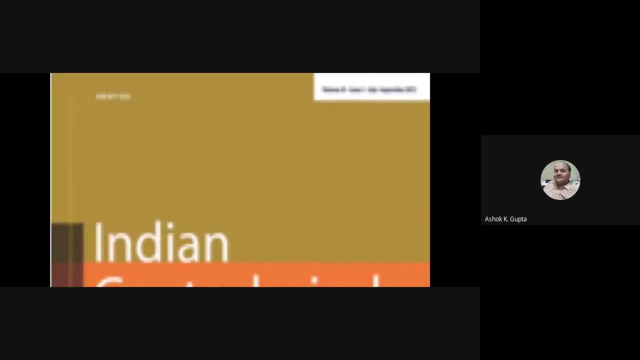 IGS has a full-fledged office in New Delhi catering to the needs of its members. IGS publishes a quarterly journal since 1962. It is now accessible online to all. Since 2012,, the journal is being published by Springer for qualitative improvement and. 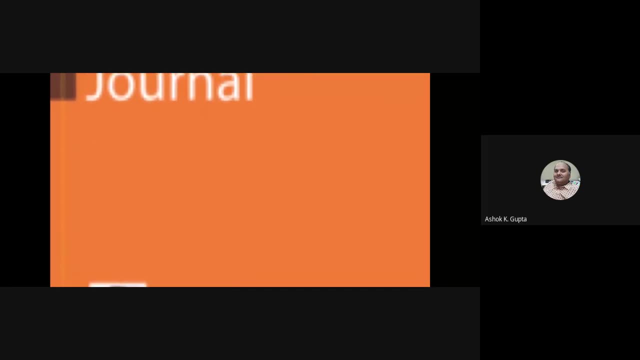 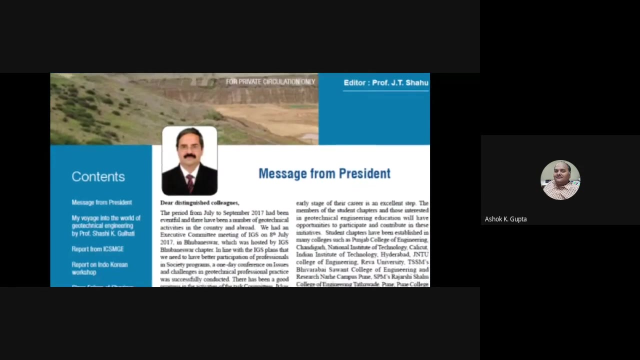 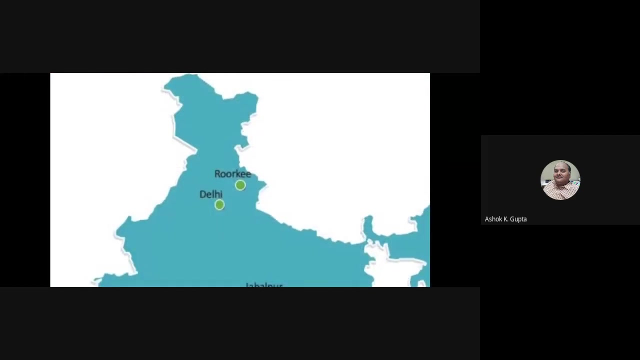 international reach. It has wide circulation and is retrieved internationally. IGS also publishes a quarterly newsletter to keep its members abreast of all geotechnical events. IGS operates through its local chapters. IGS is the largest geotechnical agency in India. 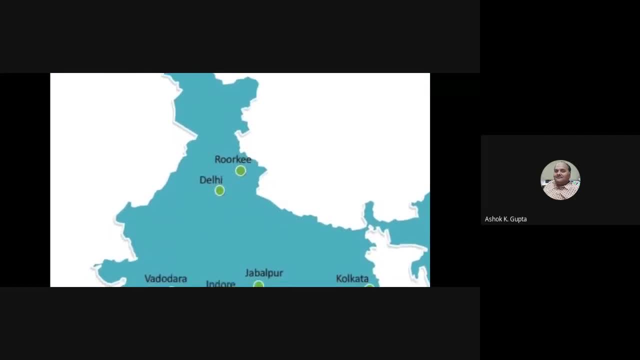 IGS is the largest geotechnical agency in India. IGS has over 100 members that keeps its flag high in different cities of India. IGS has over 100 members that keeps its flag high in different cities of India. IGS is the largest geotechnical agency in India. 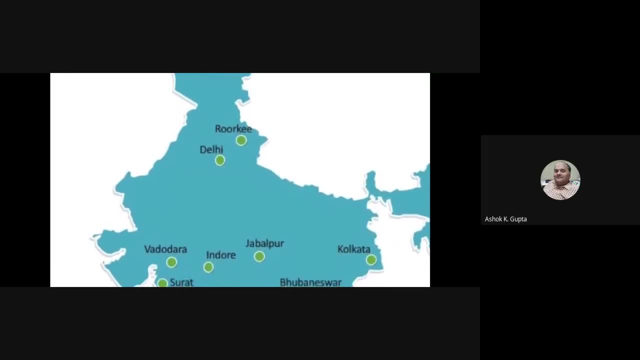 IGS is the largest geotechnical agency in India. IGS has over 100 members that keeps its flag high in different cities of India. With 44 active chapters, IGS has spread its reach to every part of the country. Some of the active local chapters include Delhi, Rootki, Mumbai, Indore, Pune, Goa, Surat. 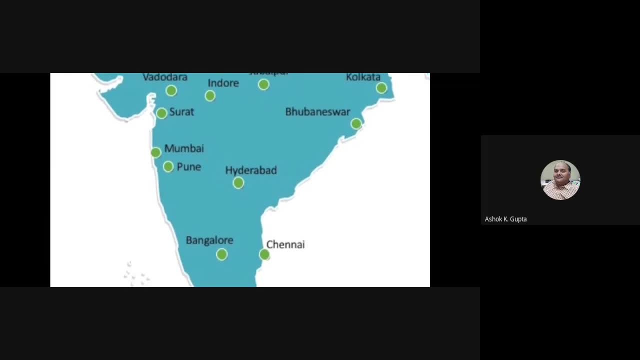 Bangalore, Chennai, Kolkata, Guwahati and several others. To encourage the chapters, an annual best-selling journal is being published. IGS is the largest geotechnical agency in India. annual best chapter award was instituted in 1995. the delhi chapter has won this award- a record. 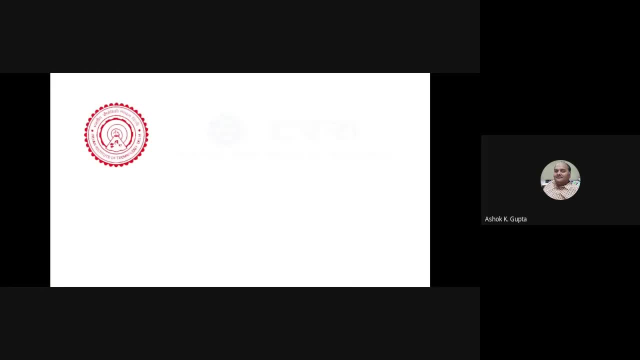 five times. the geotechnical industry in india is incomplete without its partnerships with geologists, earth retention system contractors, consultants and public sector organizations. institutions like the iits cs, mrs crri cbri, provide industry- academia interactions so that the benefits of research reaches the industry and the industry can input to the academia what the 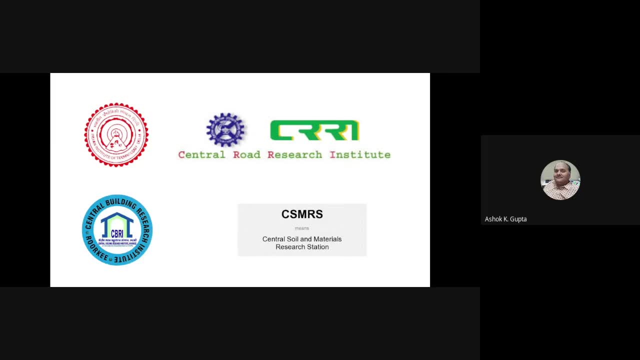 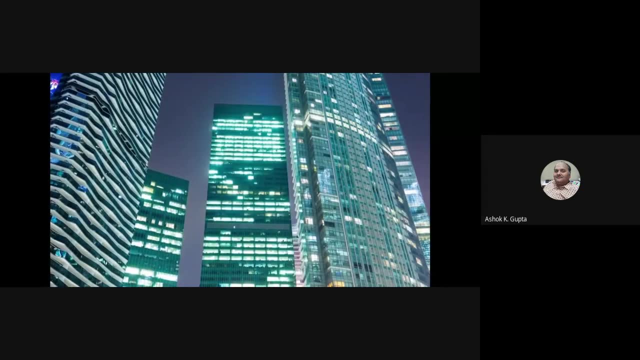 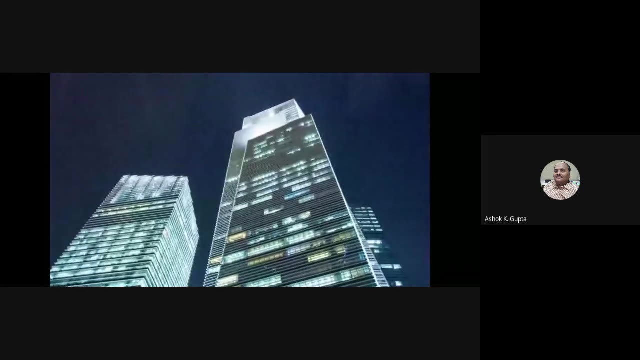 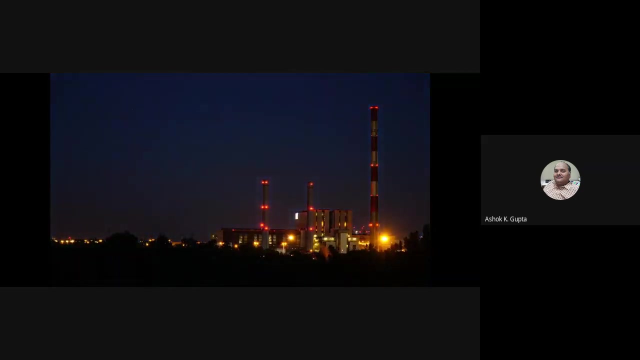 trust of the research should be. this helps in directly applying the findings of the research on the ground for real implementation. with the growing demand for land, we have skyscrapers sprouting up in every big and small city in india. as industries grow, demand for power and power plants also increases, connecting the industries through bridges. 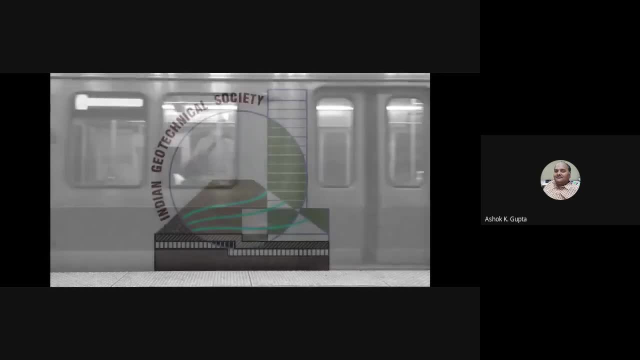 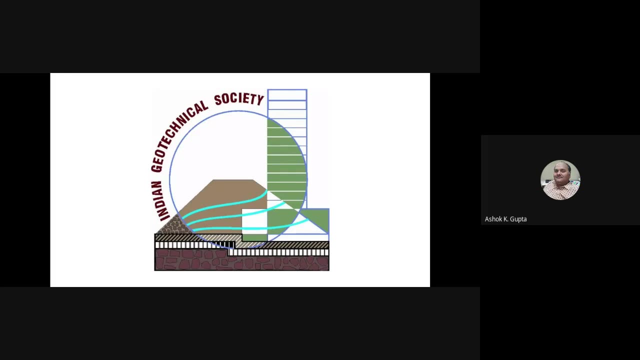 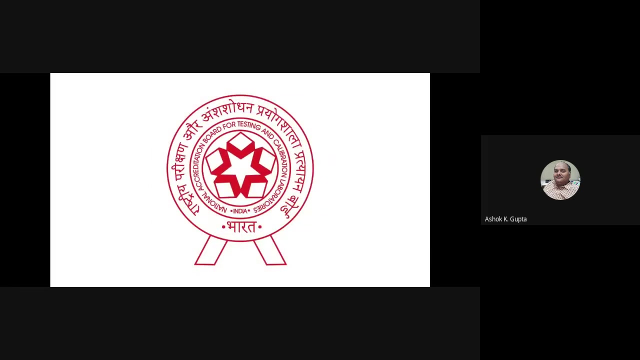 highways, railways and metros. the indian geotechnical landscape only shows a promising future. this also means that there is a demand for quality work, as the margin for error is nil. today, ig s is working towards setting up a joint assessment for testing soils, along with the national 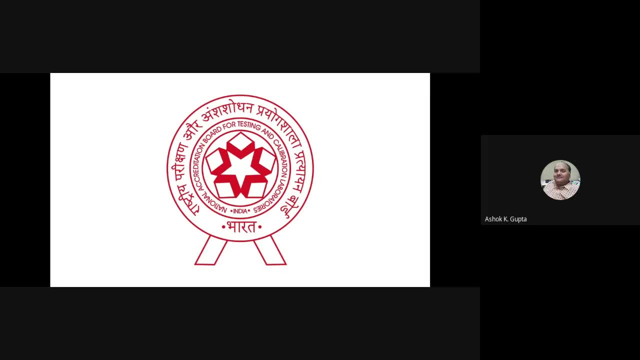 accreditation board for laboratories, the nabl, to match the quality of testing with the international standards. igs is also working with the bureau of indian standards to prepare indian standard codes in several aspects of foundation design and field and laboratory testing. many of our members serve in these committees. 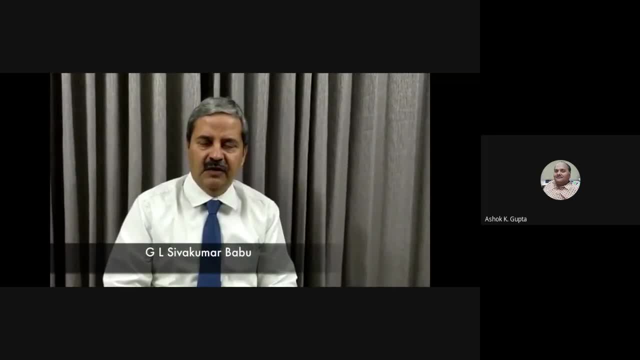 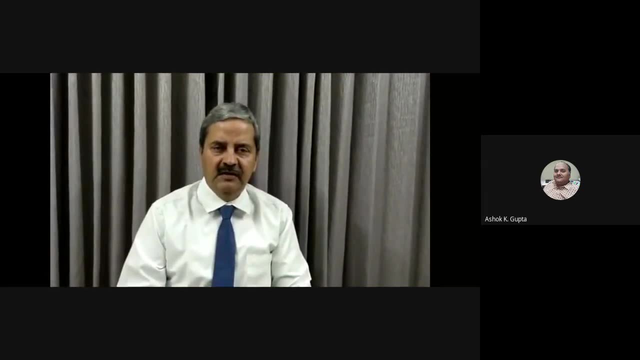 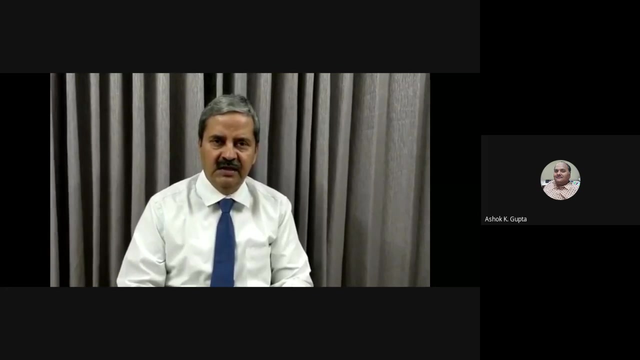 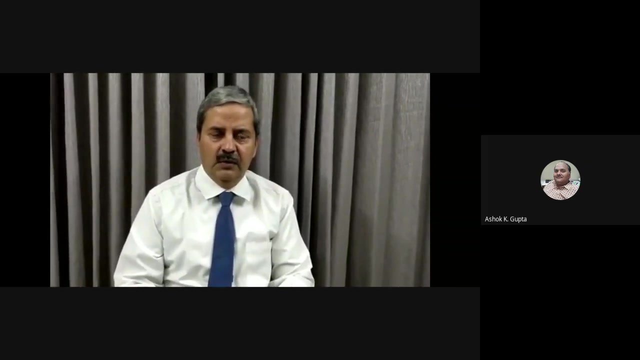 the future is very bright and full of optimism. a number of initiatives have been taken up: promotion of student chapters in various colleges and institutes to sensitize the students about the importance of geotechnical engineering in their curriculum and the practice. creation of number of professional groups to make them aware of the future challenges and opportunities in the. 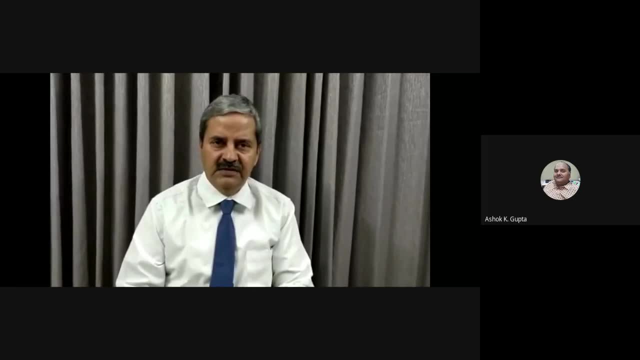 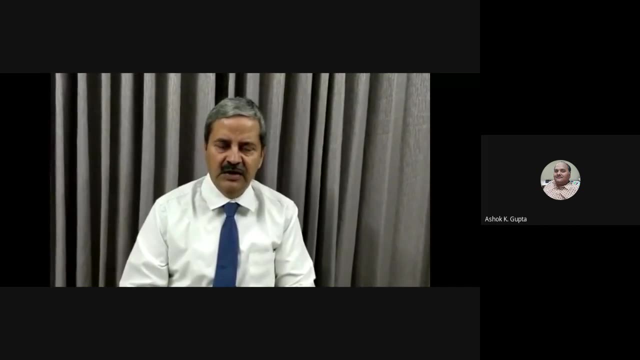 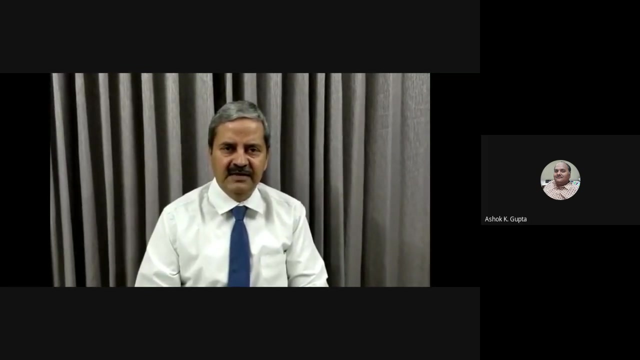 geotechnical engineering. a number of initiatives, such as interactions with other professional groups that are overlapping with geotechnical practice, are also initiated. it's hoped that with all these initiatives and further initiatives that one can have at igs level, there could be better geotechnics in the country which ultimately to 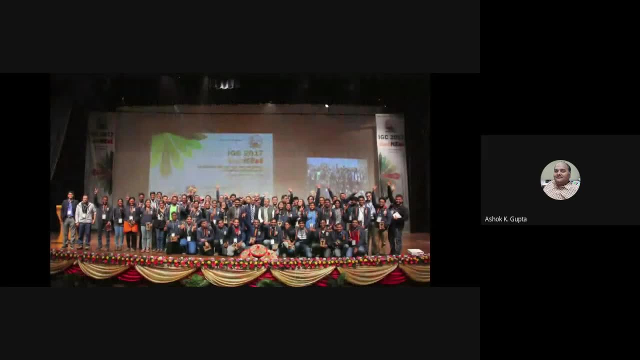 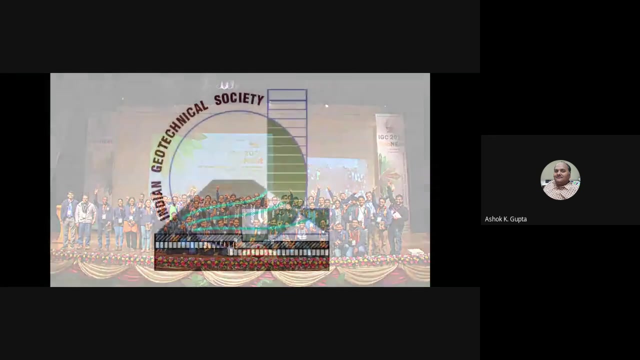 better, cleaner, sustainable societies. the future of geotechnical engineering lies in the hands of students. recognizing this, igs has set up student chapters in some cities. several more in the offering as we celebrate the 70th year of the indian geotechnical society: the possibilities. 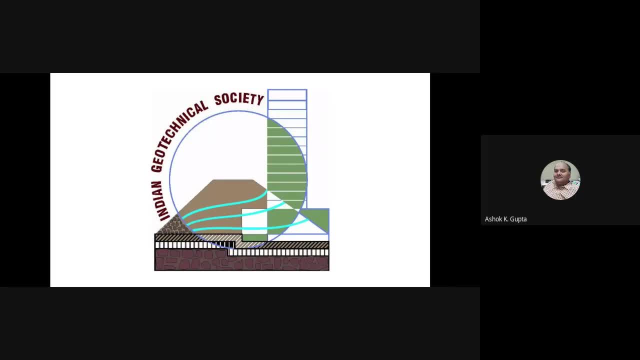 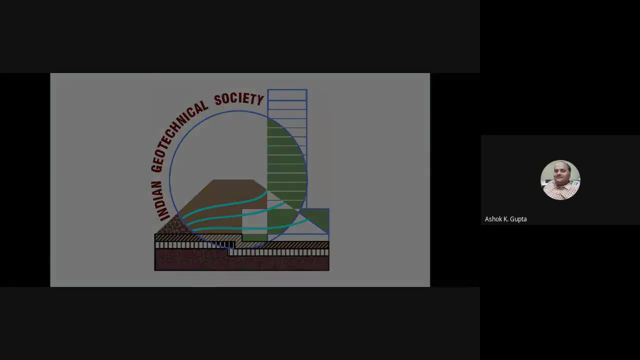 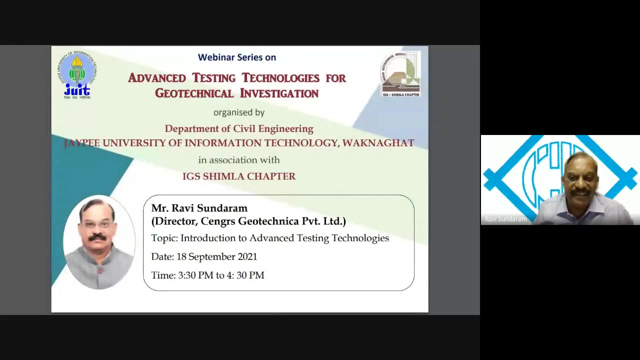 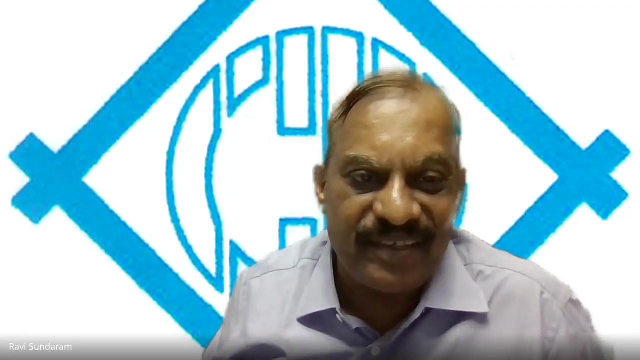 that we look forward to are limitless. here's to saluting the past, celebrating the present and welcoming the future. this video was. this video was actually made in 2018 to celebrate 70 years of igs. of course, now igs is 73 years old and in two years, we'll be celebrating the. 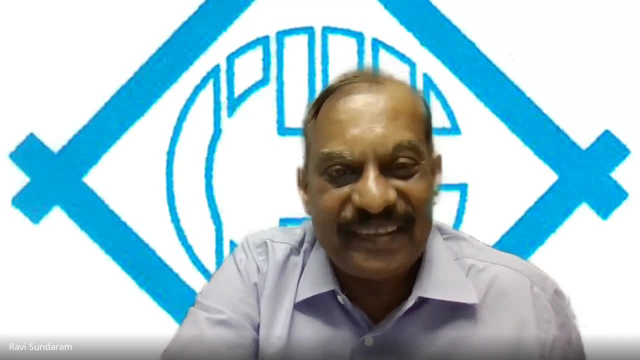 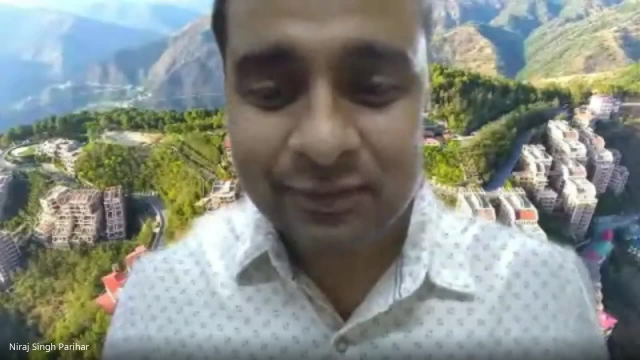 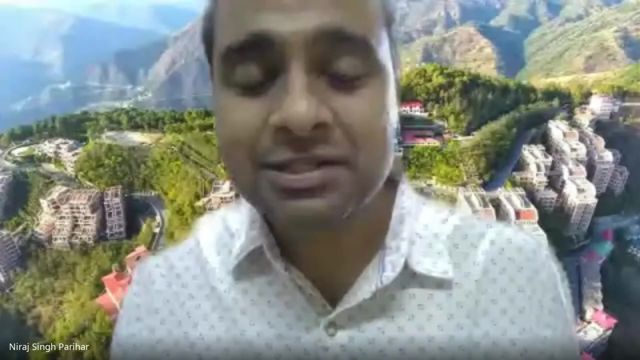 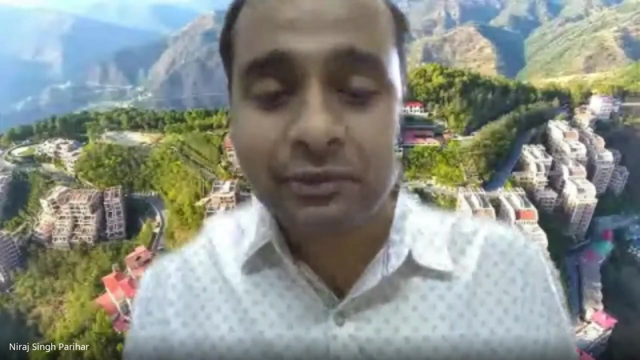 platinum jubilee, so that will be a big event which we all look forward to. yes, definitely so. thank you everyone for the for being a patient listener. it's really because of those great people and the work of those great people- whether accommodations, researchers or industry, people who are made reach the ideas to this heights, and we are really thankful to igs. 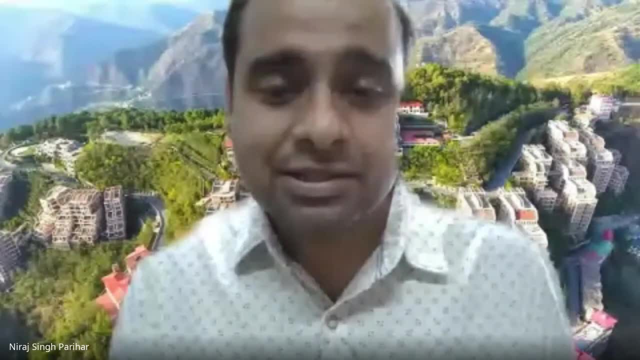 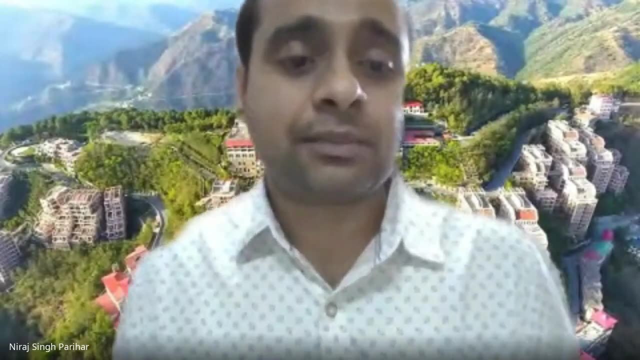 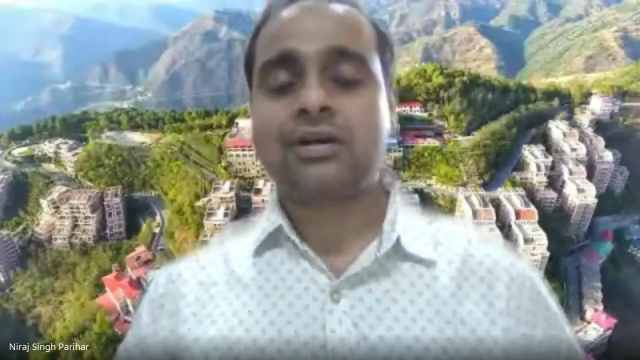 for providing this great platform where we can readily share our knowledge with each other so easily. so with this note uh, we will further progress onto the inauguration ceremony of the event. so first of all, i would like to invite and welcome professor dr ashish kumar rohila, uh hod of civil engineering department and one of the initial joining. 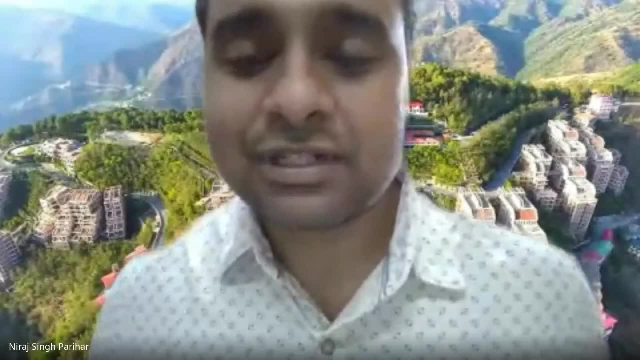 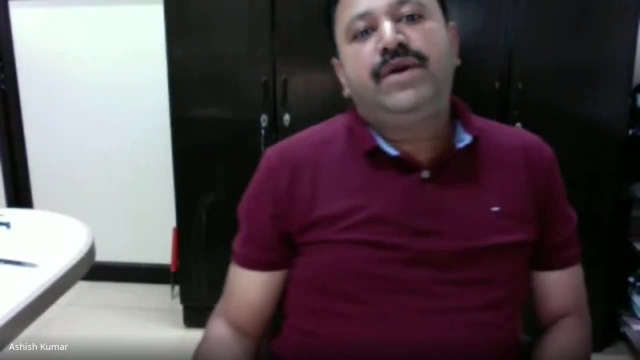 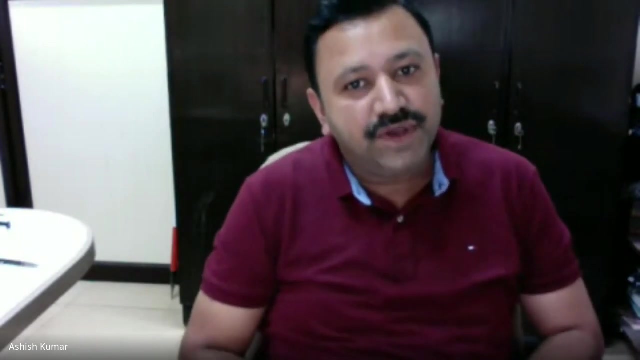 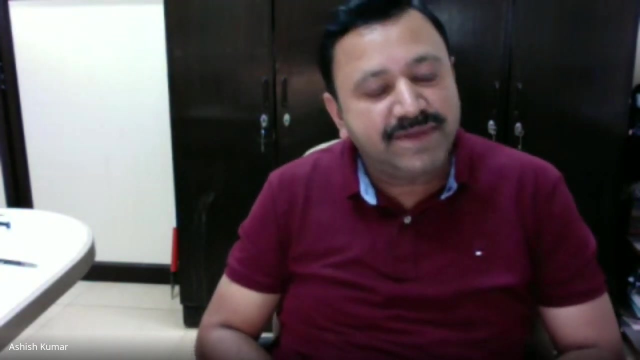 members of igs shimla chapter to kindly share few words with us. thanks, neeraj, for giving me opportunity to talk something about the geotechnical engineering. good afternoon to all of you and, on behalf of department of civil engineering, i warmly welcome all of you in this webinar series. 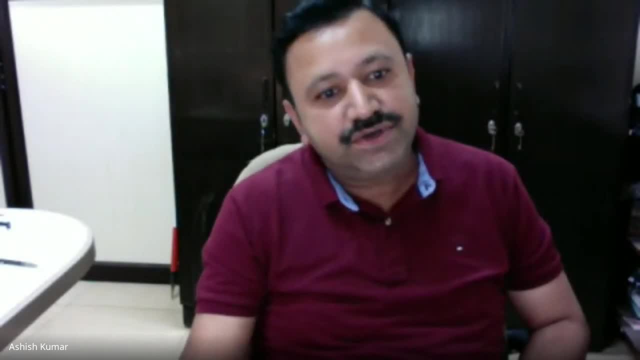 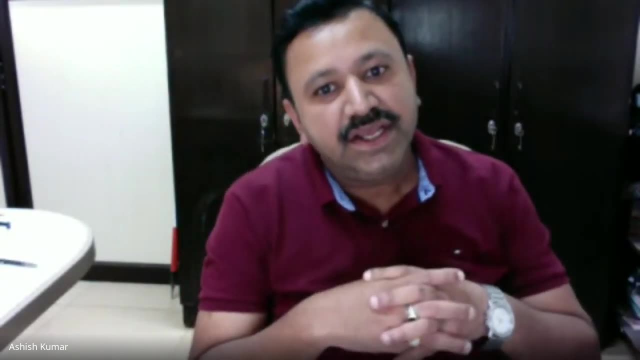 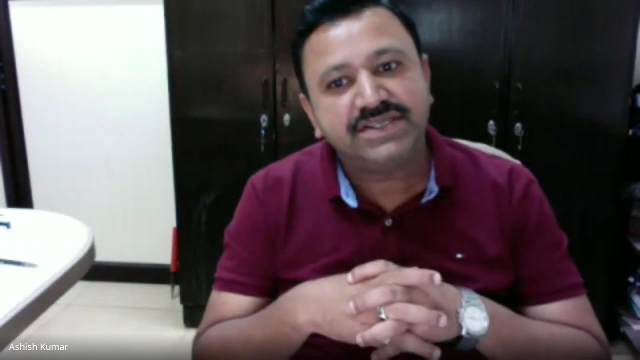 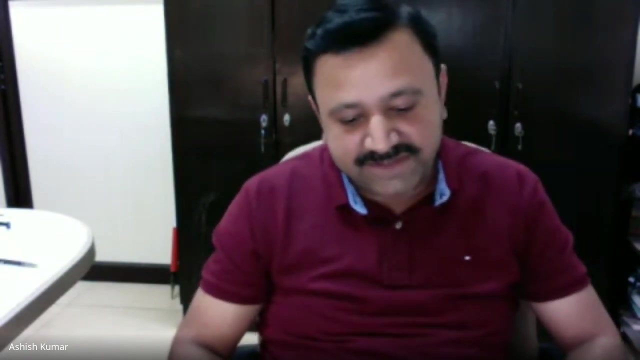 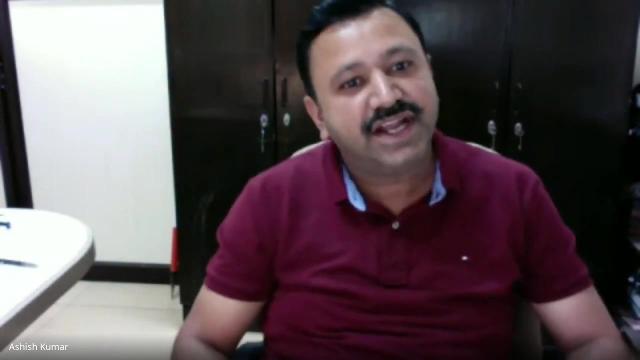 advanced testing technologies for geotechnical investigations that is jointly organized by department of civil engineering and indian geotechnical society. we are grateful to our speakers of the sessions, presently mr ravi sundaramji, director of synergy. synergy centers geotechnical private limited. we are thankful to you, sir, that. 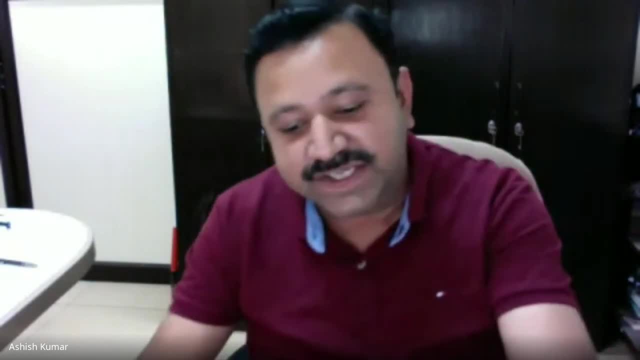 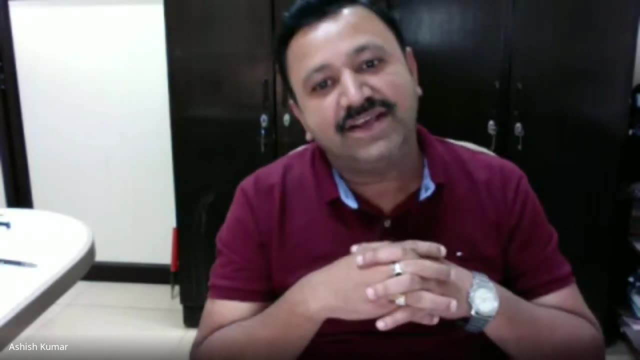 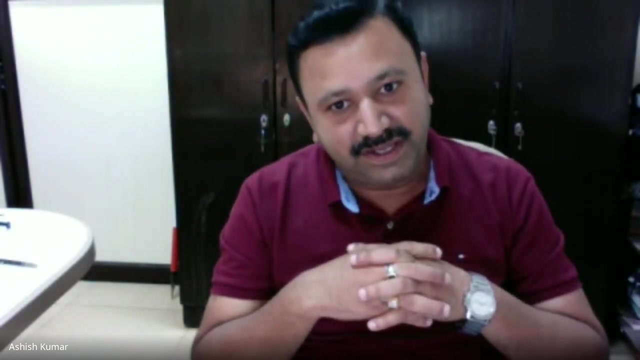 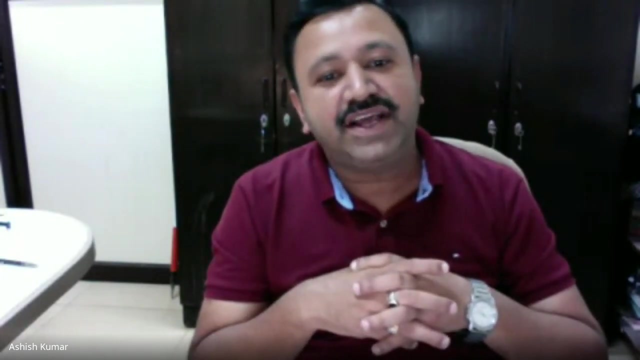 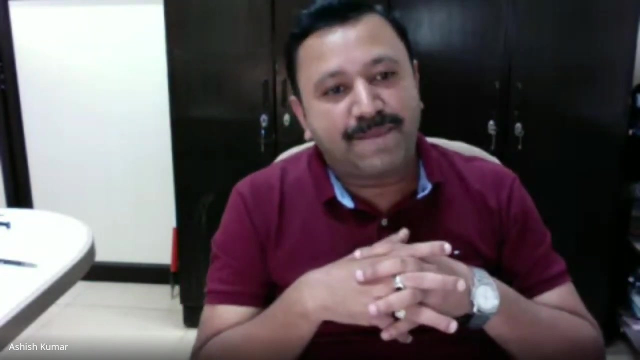 you have here for sharing your words and what you have done in this field. so i believe that we all will get benefited with your clients words and what expert things you have done in the field of geotechnical engineering so well. a geotechnical vast area and needs no introduction and, as we have also seen, that 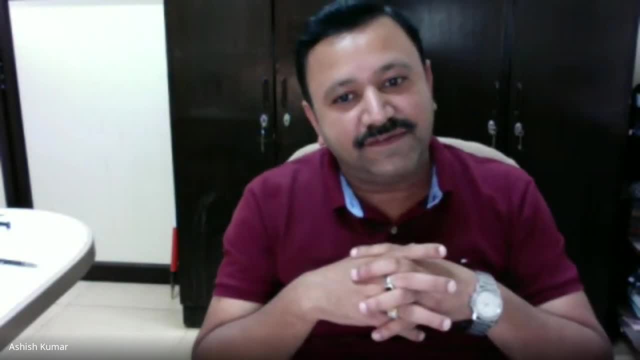 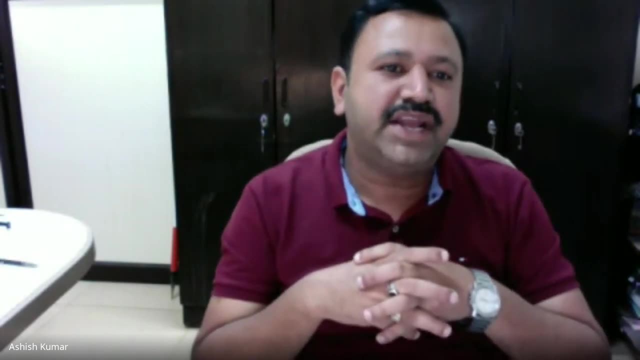 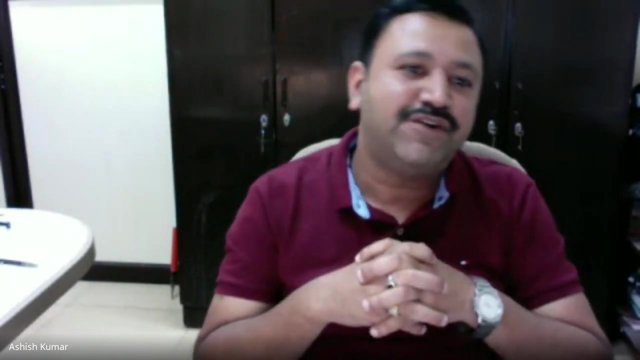 indian geotechnical society has done a lot of work in last 70 years and that is very great. and we all know that a geotechnical engineer is basically a bone. we see that every structure we create needs a foundation like so we see that that a geotechnical 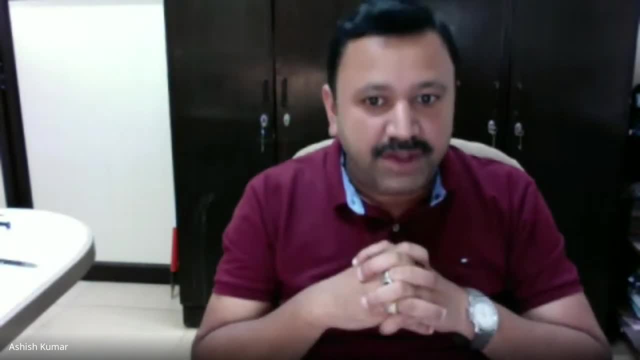 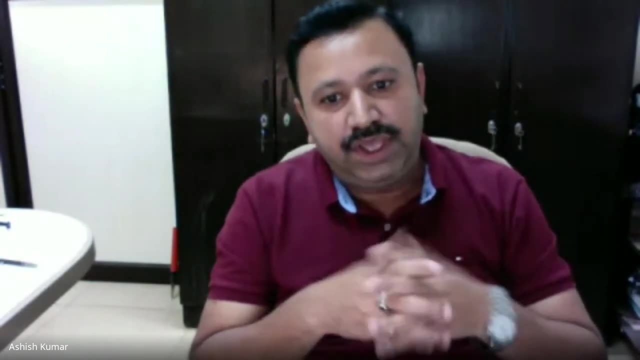 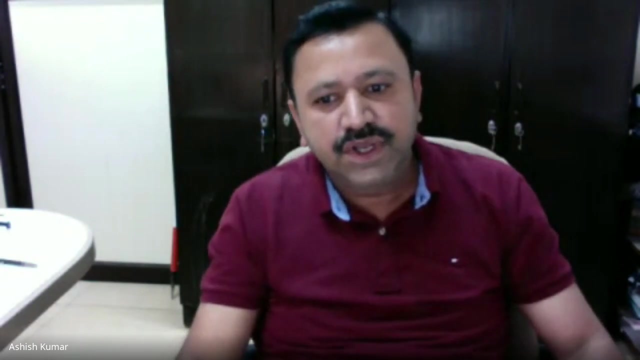 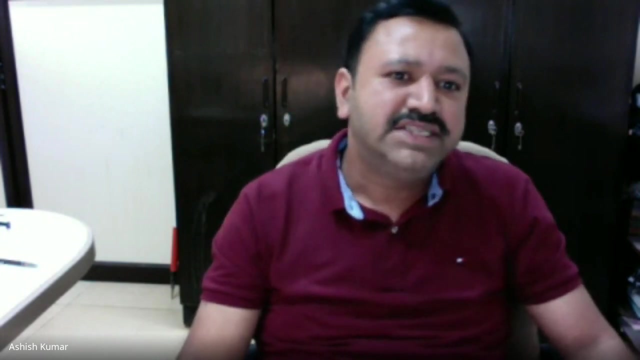 engineering is basically a foundation of any engineering is a foundation of any structure, so is involved from the start, from the conception of any idea of the structure. and if we see that a geotechnical engineers is involved basically in investigations of the subsurface conditions and materials, like what is the soil, what is the rock strata, and then 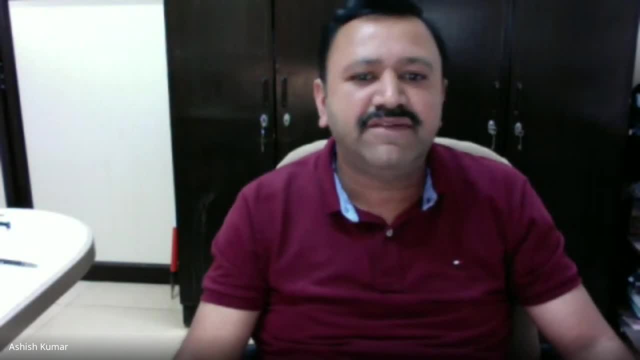 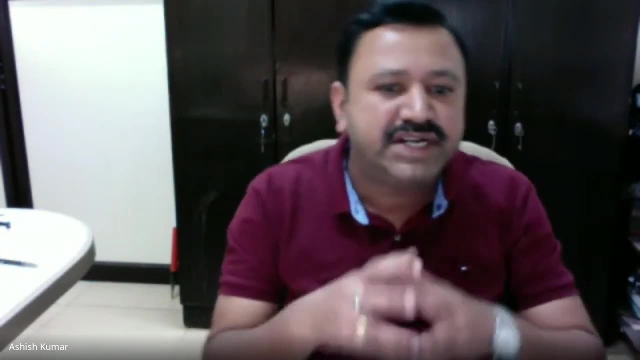 finally, how we can design our structures like retaining structures. we are working for the dams and then we are working for the tunnels, and nowadays we can see that highway structures are going on and then we are working for the tunnels and then we are working for the tunnels. 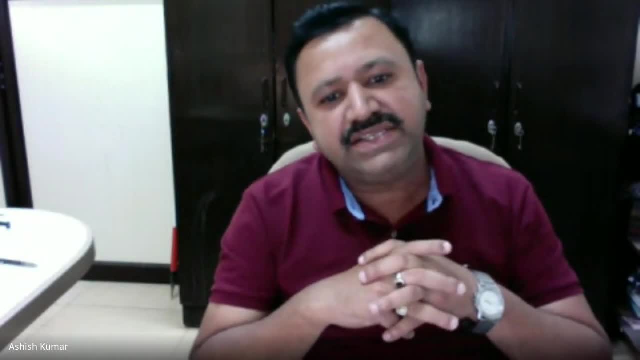 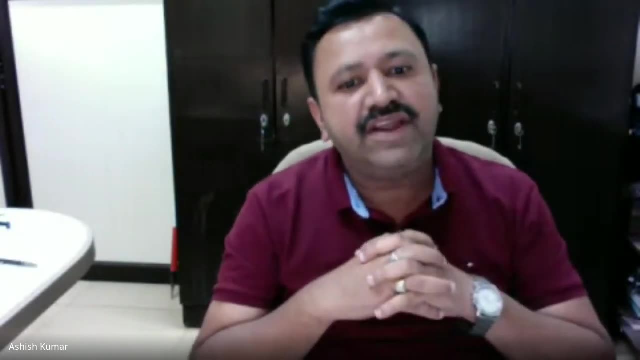 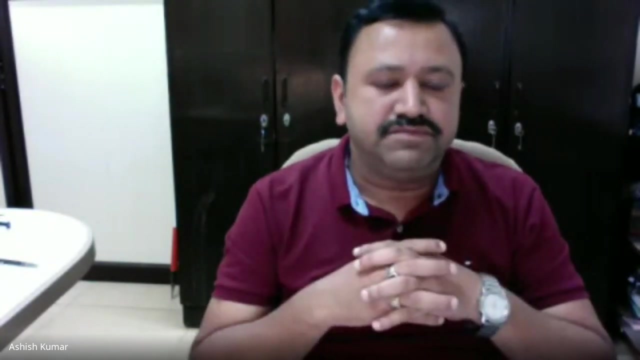 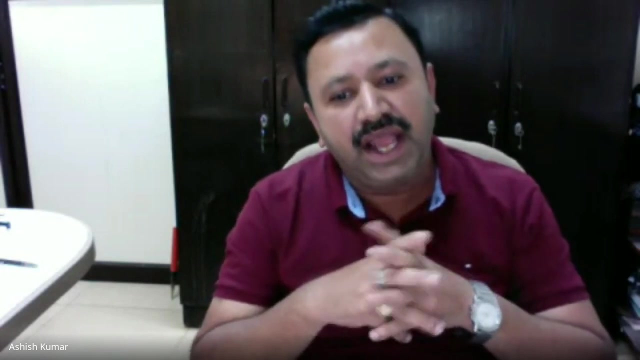 for in a big way and we are designing the numbers of tunnels. so, in this way, what we see, that uh role of a geotechnical engineer is very, very much important and, as such, as our, we have an era of the instrumentation and the automation, and that's what we see, that our techniques for the 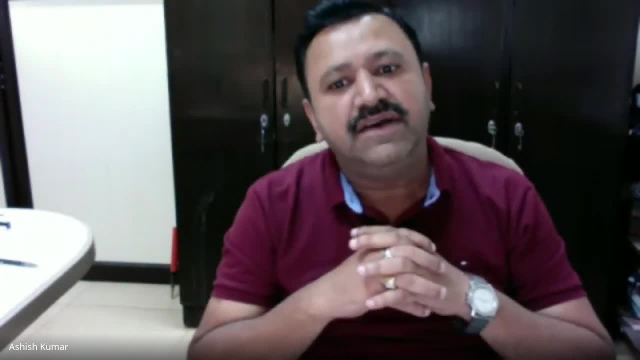 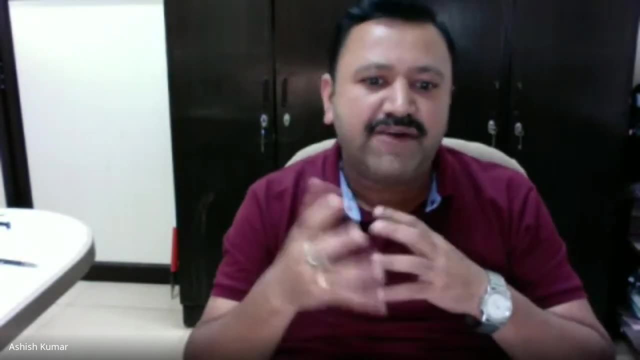 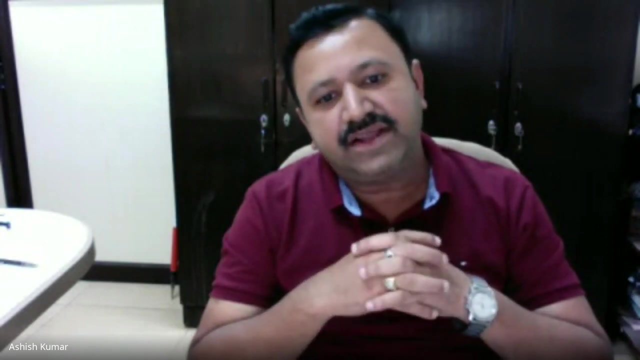 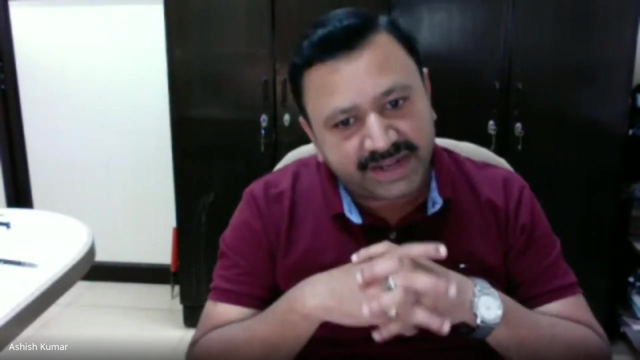 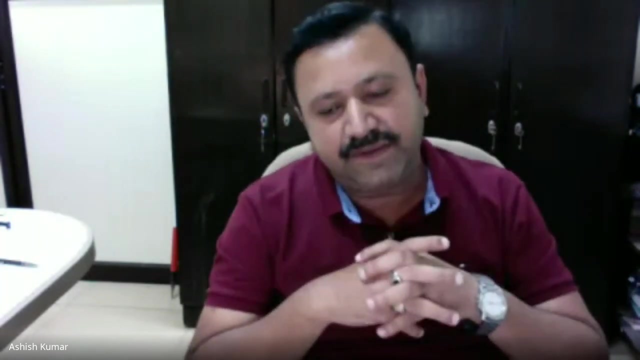 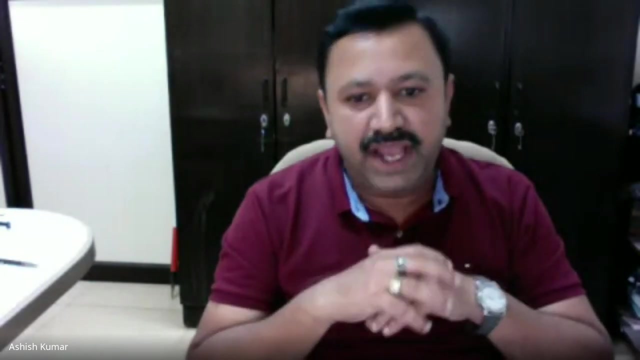 experimentation and finding the various physical or chemical parameters of the subsurfaces. that have boosted refinement, the use of artificial intelligence and machine learning in order to find out the various parameters. so that is very, really good thing that we are. we, as a civil engineer, are also working and also 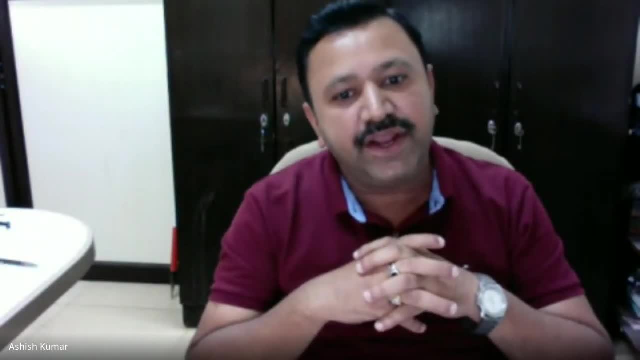 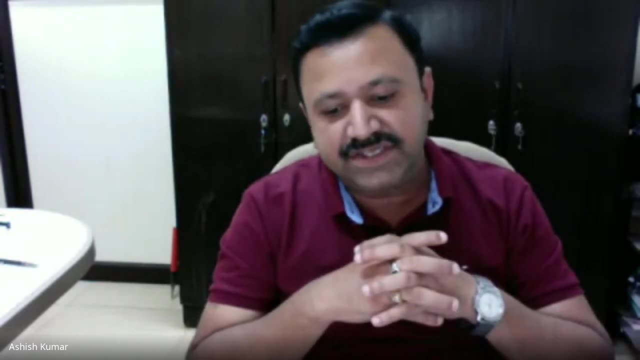 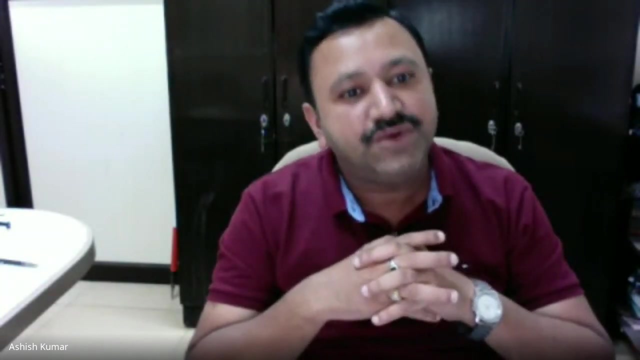 popping up with our new, latest technologies and we are incorporating all these things so that what we have with us- that, mr ravi sundranji, that is giving us the idea about what advanced testing technologies we are using in presently in the field, and i hope that our listeners and 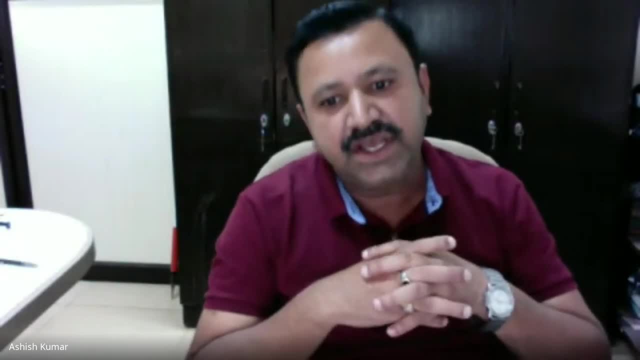 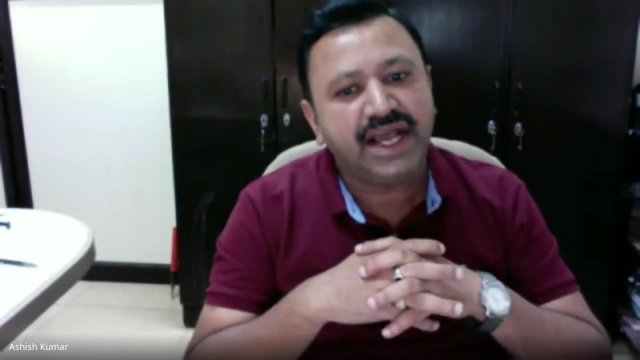 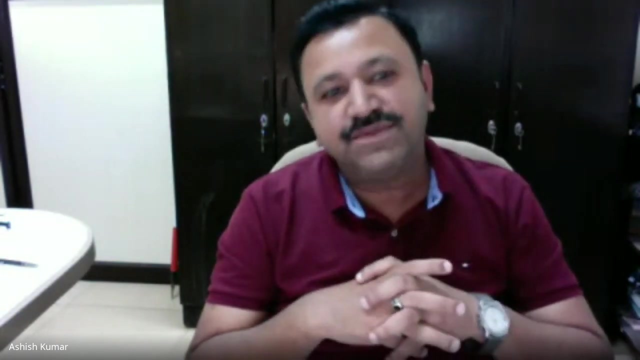 whether it is from the industry, whether it is from the academics, whether it is the students, they will all get benefit from his expertise in that area. so with this verse i will not take so much time, because already we are running, we are also consumed: 30 minutes. so thanks, and i hope that. 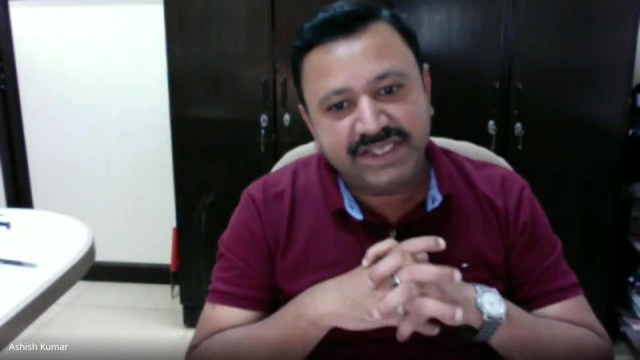 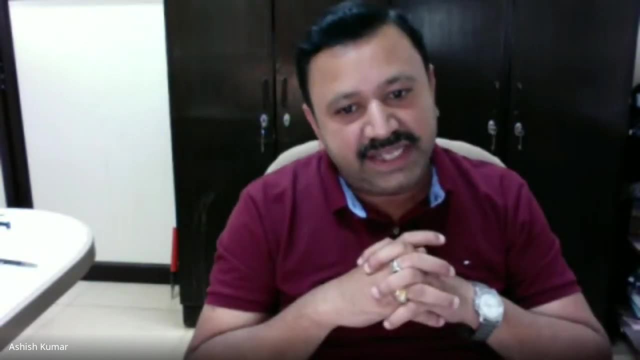 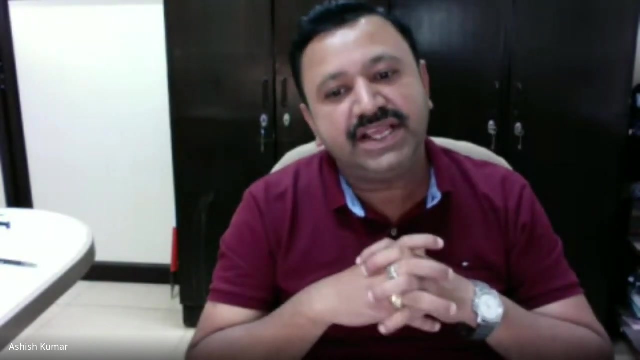 our you listeners will get benefited with this and uh. lastly, i am thankful to our vice chancellor, professor arke sharmaji, and our professor, dr ashok kumar gupta. he was, he is presently dean academic and research and he also, uh, good geotechnical experts and he is also having a 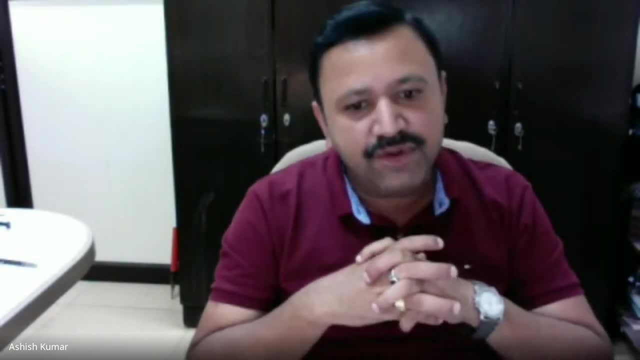 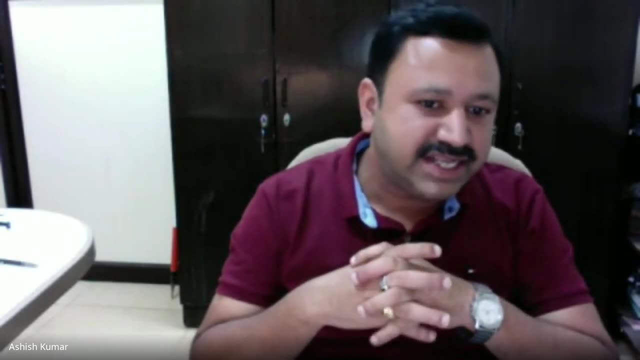 vast experience in that area. i am thankful to both of them that they have uh provided me with this opportunity and i hope that we will get benefited with this, and i hope this is some opportunity to conduct this webinar session. and, lastly, uh, Mr neerajulseen parihar and. 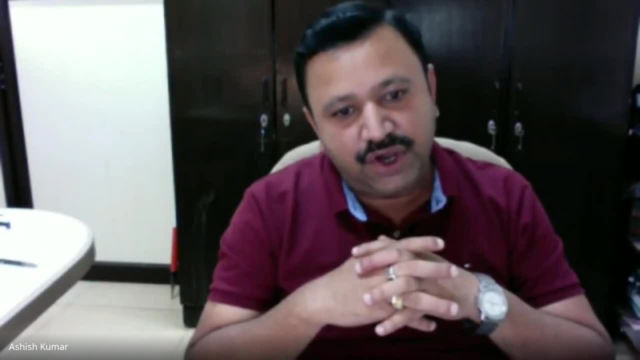 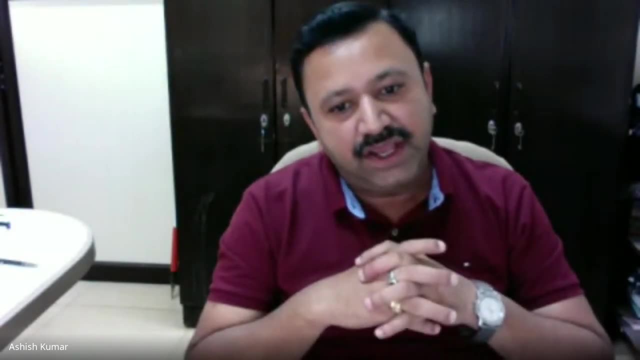 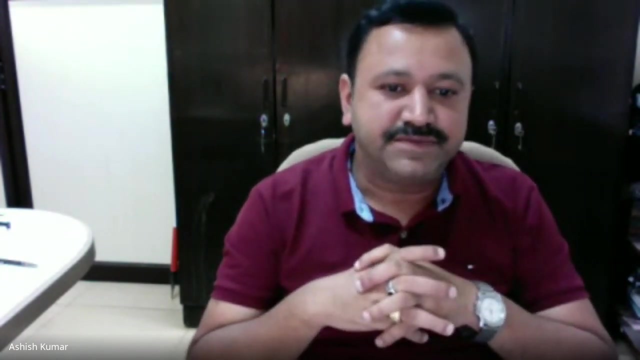 Rohan singhal. they have done a good job in order to organize this event of this webinar session. so with this course, i uh handover the session to neeraj again to kindly continue this. hence. thank you, sir. thank you for your nice vows, appreciation with this. next, i would like to 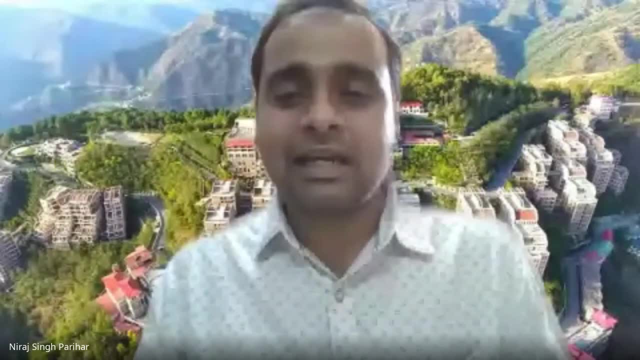 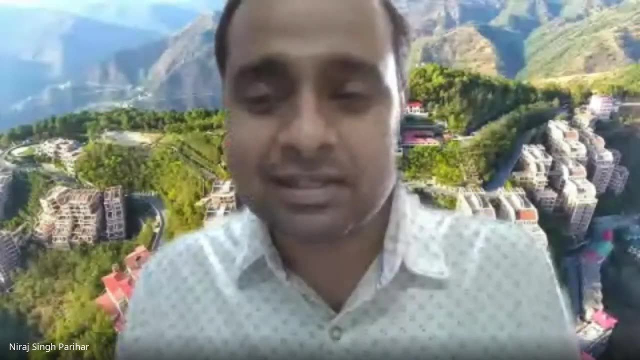 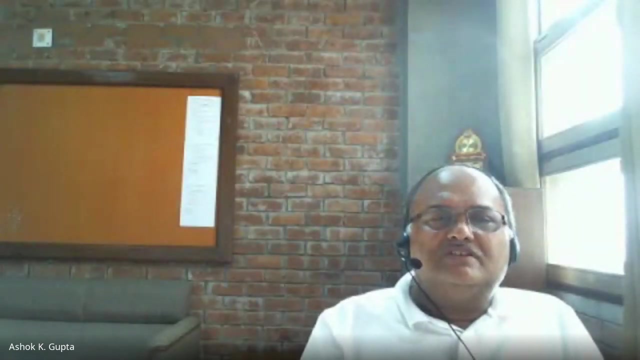 invite and welcome Professor Dr Ashok Kumar Gupta, Dean academic and research JYT and chairman of IEA Shimla chapter, to kindly share few words of wisdom and also declare this event as open. over to you. sir. Honorable Ravi Sundaram ji, Director from Sanger Geotechnical Limited, New. 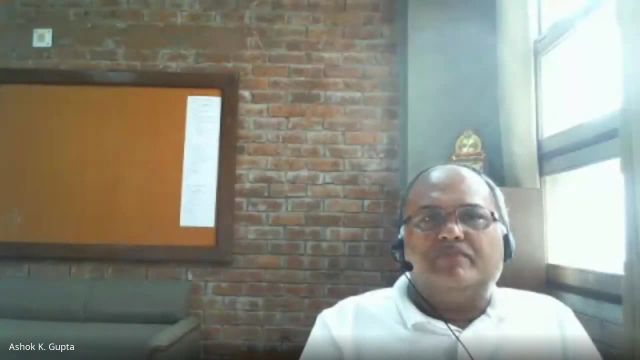 Delhi, our HOD in Civil Engineering Department, Professor Ashish Kumar, the man behind this, the two person behind this workshop, Mr Neeraj and Rohan Singhal- actually they did a lot of work- all the participants here, my dear friends. actually, for any event of this size, I should thank the people who will. 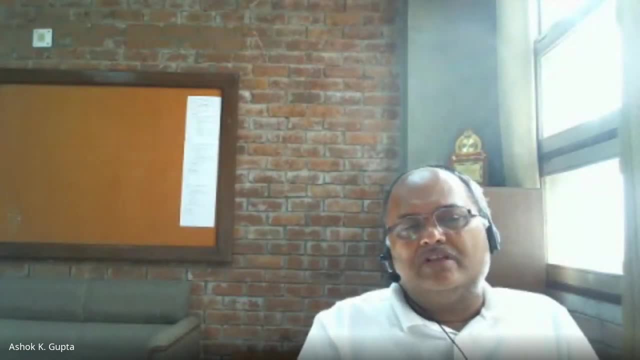 going to our who's over. I the responsible for doing all this. actually, I should thank civil department that he helped us in the civil engineering department, that he helped us in the civil engineering department. JYT Vaknagar that he has taken up this. call that, okay, we help. IGS- Shimla chapter. 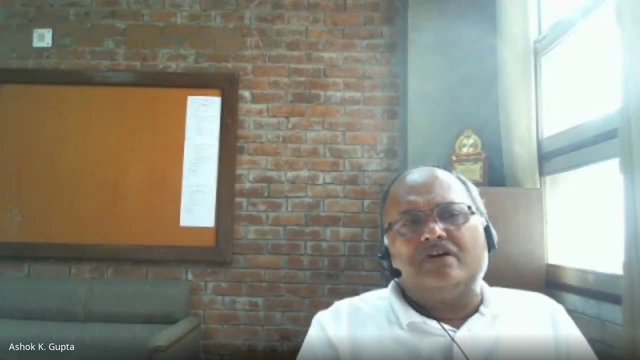 to this and to this activity and, as he did, a lot of help in this case. I also thank Rohan Singhal and Neeraj and they took up the challenge and they do all the work. actually, all the behind-the-scenes work is done by these. 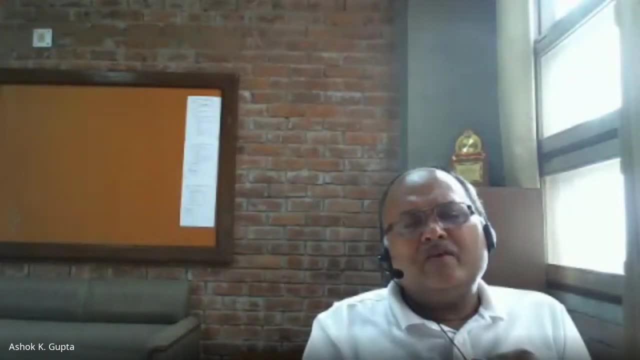 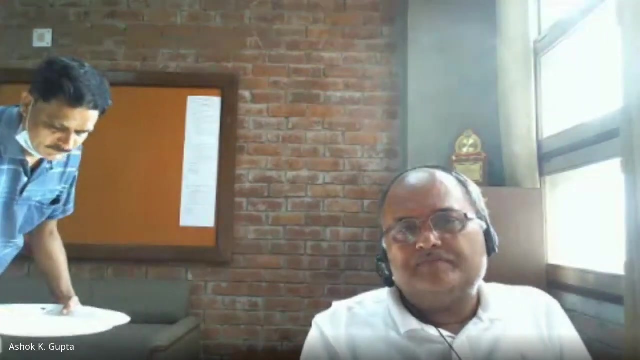 two gentlemen, so I am thankful to them and, with the permission of all present here- all the participants and Ravi Sundaram ji- I declared the this event open. let God help us that this event go through very well and I am hopeful that it will be a successful grant. thank you so much. thank you, sir. 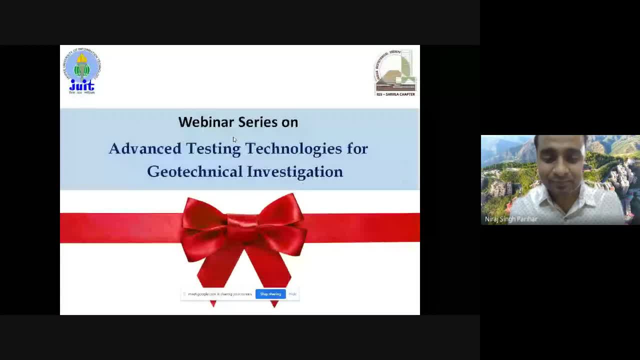 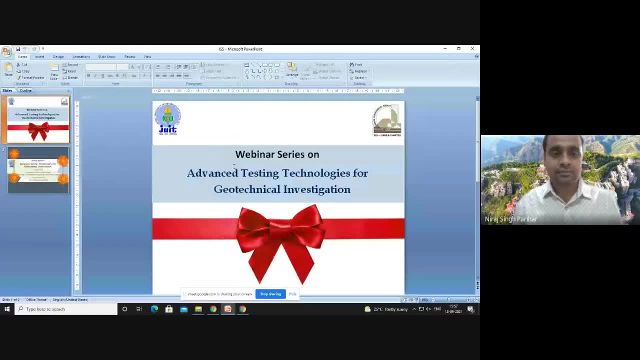 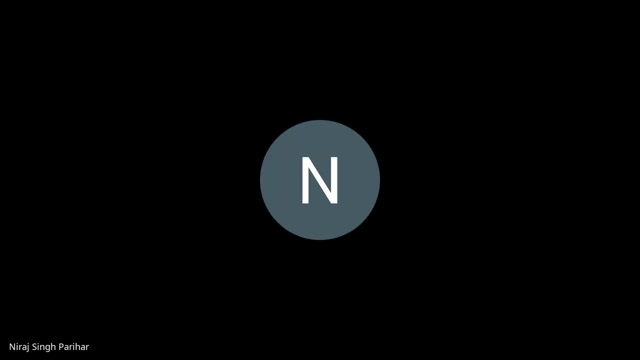 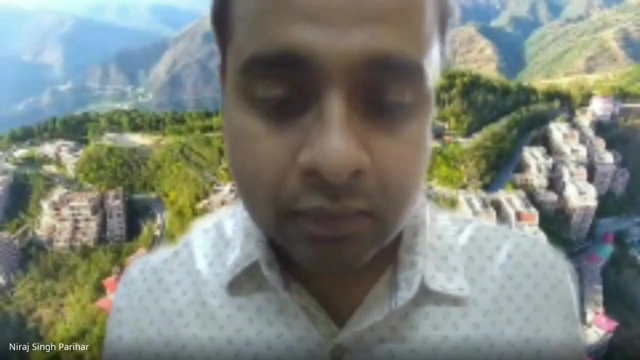 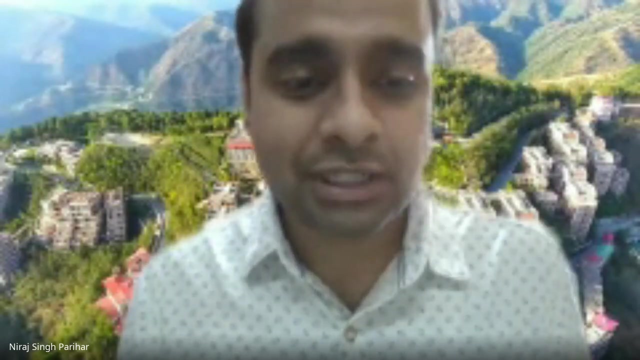 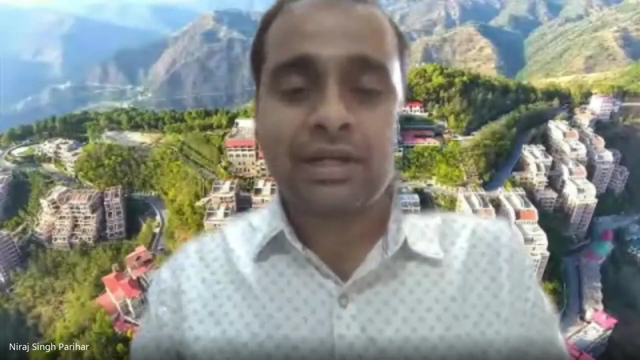 thank you very much, you so. thank you, sir. now the event is open to everyone and we will be proceeding through the next round, that is, the lecture session round. so now, on the behalf of the entire JYT community, civil engineering department, JYT and IGS, 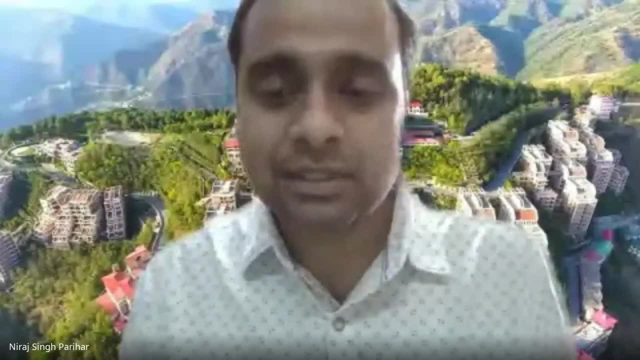 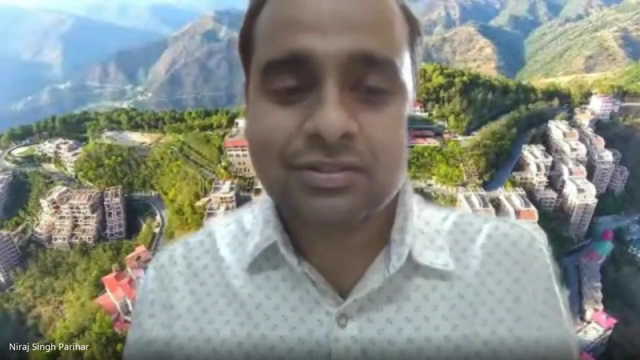 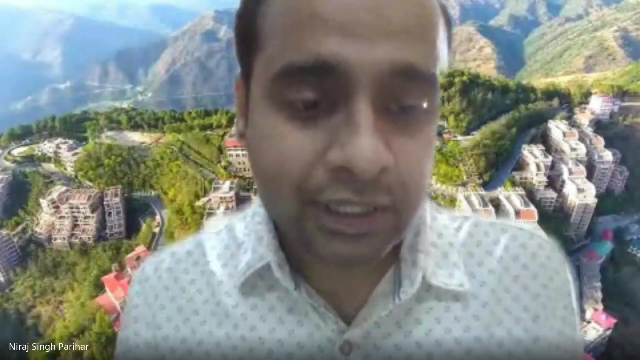 Shimla chapter, we would like to welcome our geotechnical experts speaker of the day, mr Ravi Sundaram ji. welcome to you, sir, and it's a proud moment for all of us to have you here on this platform of IGS Shimla chapter. now giving a brief introduction about him, mr Ravi. 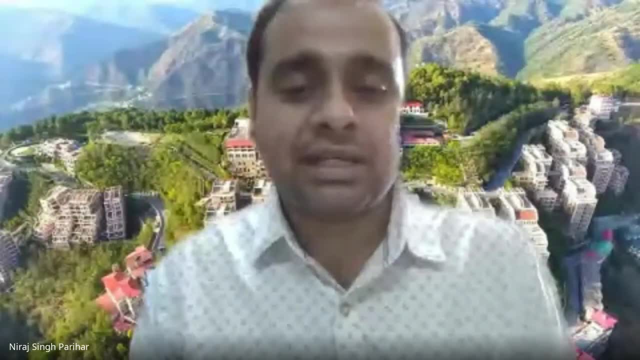 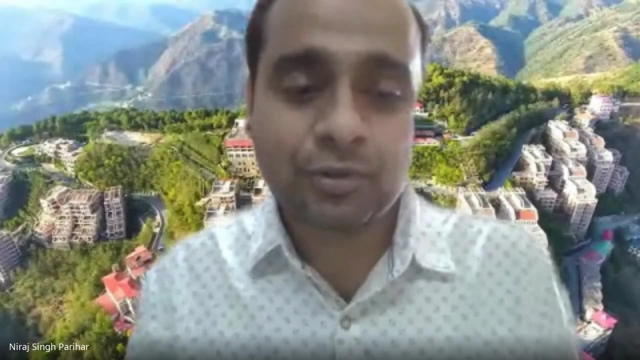 Sundaram ji, BTech in civil engineering 1978 and M tech in soil mechanics and foundation engineering in 1980 from IT Delhi, is a person of high repute both in the field of industry and academia. he's currently the founding director of singers geotechnical department in India and he is the founder of the project. in the field of industry and academia, he's currently the founding director of singers geotechnical. 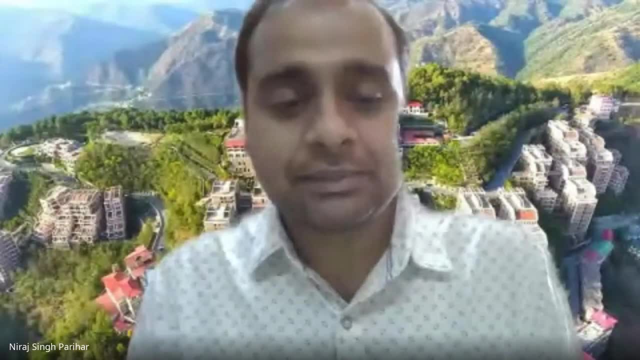 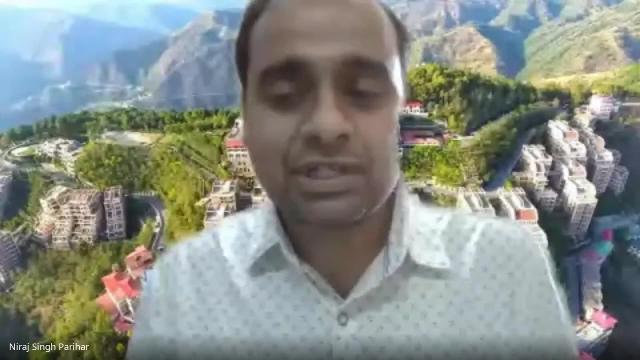 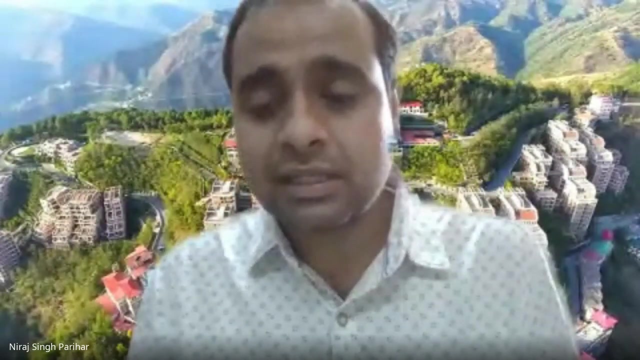 Private Limited and also the fellow of Indian Geotechnical Society. Starting his career with McKellan Engineers USA and working at various official locations in Saudi Arabia, Qatar and UK, Mr Ravi Sundaram became the founder director of Singers Geotechnical Private Limited, which was established in 1990 by IIT Delhi. 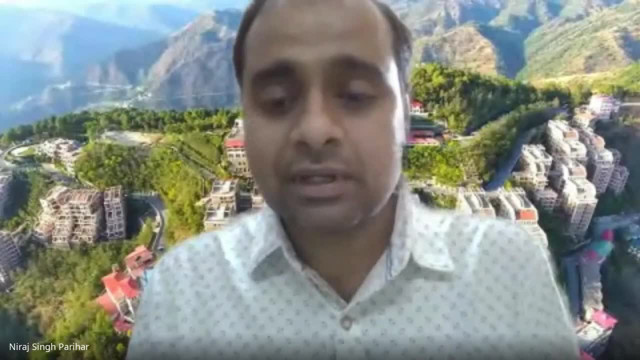 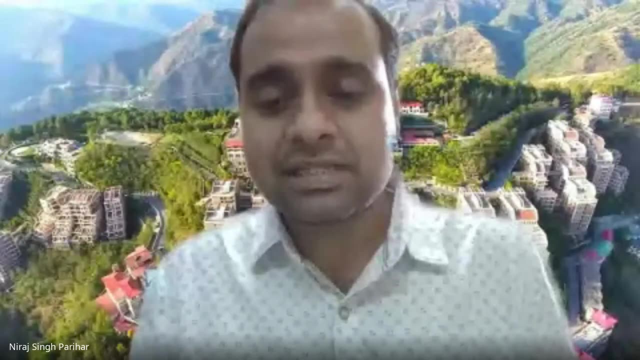 graduates. Now this is one of the leading geotechnical private organization in India as well as abroad. Mr Ravi Ji directs the company's geotechnical consultancy services, as well as the geotechnical construction activities. His expertise includes geotechnical investigations, geophysical surveys. 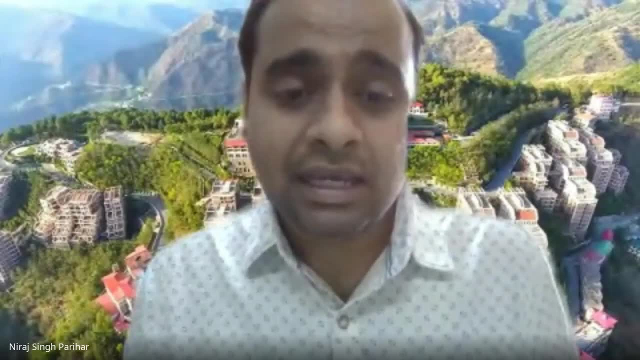 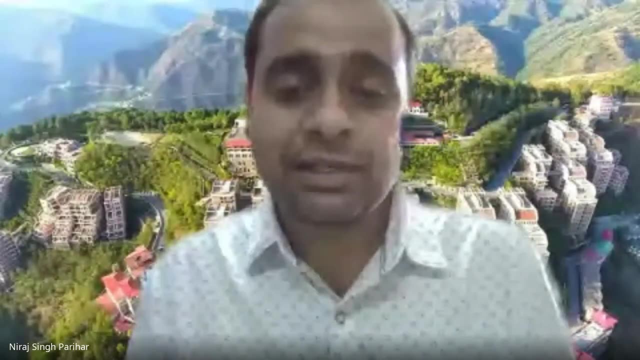 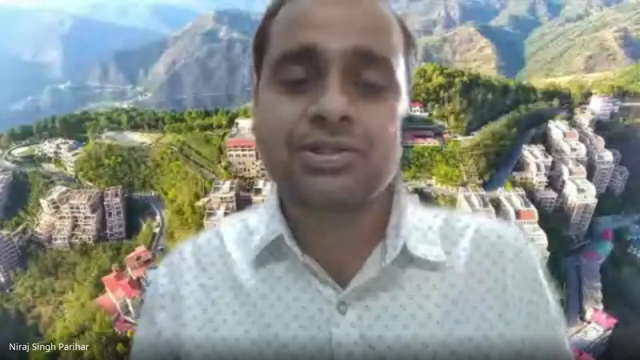 ground improvement and groundwater studies. He has been actively involved in developing the engineering solutions to problems of foundations under artisan conditions, collapsible dune sands, soft place, expensive soils and many more. His special interest lies including the geotechnical solutions for foundations for tall buildings, thermal and solar power plants. 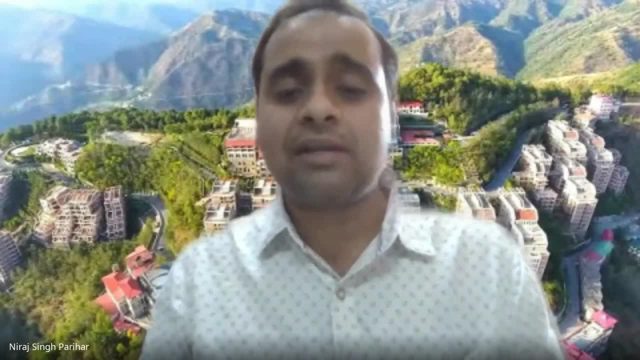 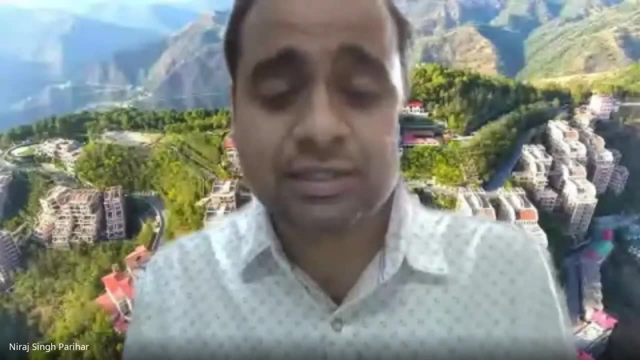 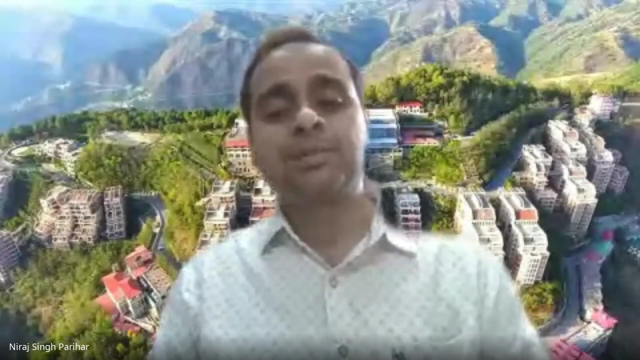 and bridge foundations, besides testing of pile foundations and strengthening of weak and distressed foundations. Now, above all, the industrial experience he has, he has also significantly contributed in the field of academics and research, where he has published more than 70 quality research papers reflecting his true experience in geotechnical practice. He has strived to 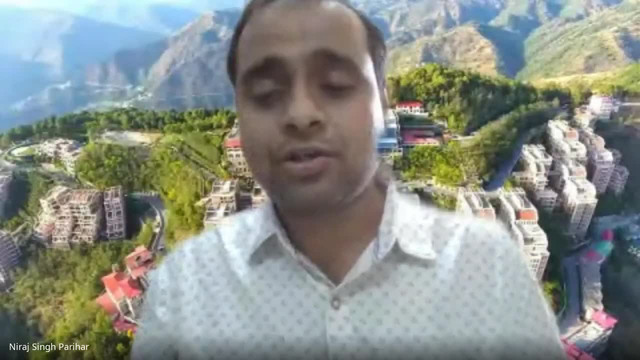 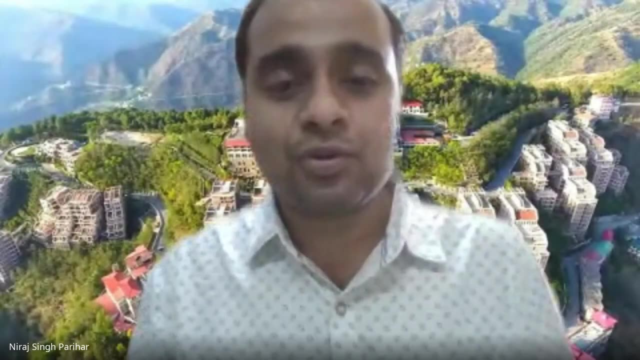 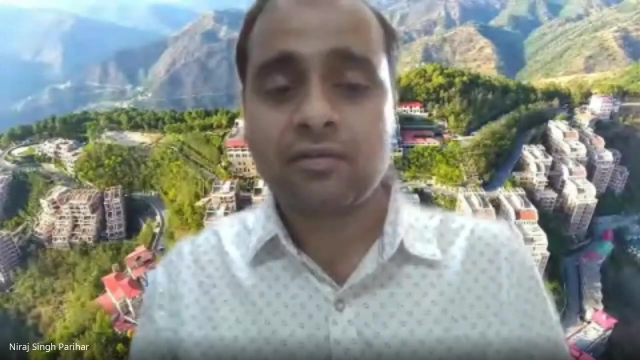 integrate the field experience with the academic research in order to build responsive to complex geotechnical challenges faced in India. He is also the co-author and co-reader of two very renowned books. One is Geotechnics for Transportation Infrastructure, published by Springer Nature in 2019 from Singapore. 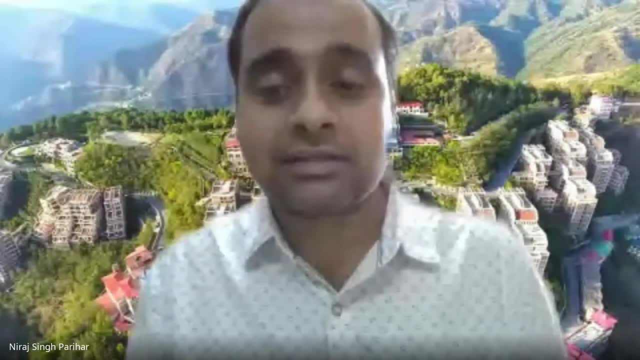 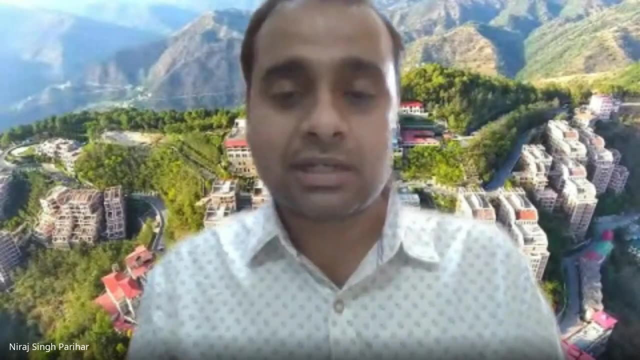 and another one is Retrieving the Lost Paradise, Celebrating the Earth Day, published by Northern Book Center, Delhi in 2001.. Talking about his achievements, Mr Ravi Sundaram Ji has a number of accomplishments and awards to his name, To name a few. Mr Ravi Sundaram Ji has a number of accomplishments and awards to his name, To name a few. 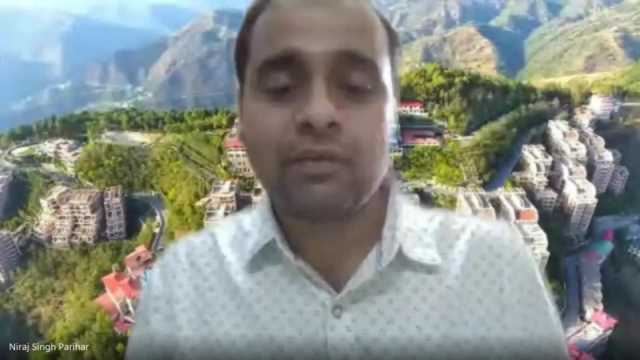 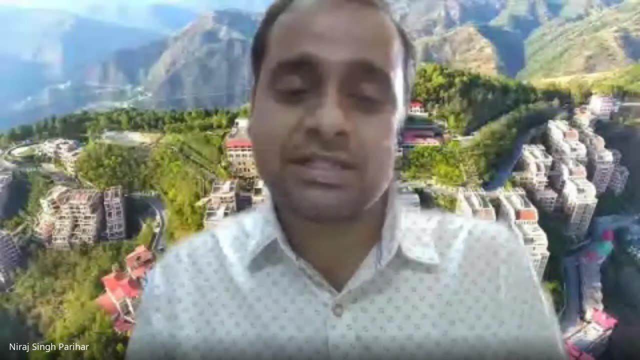 he received Professor Dinesh Mohan Memorial Award in 2017 and 18 by IGS for excellence in professional practice. He also delivered the prestigious 6th Mahadev lecture in honor of Professor Mahadev in 2017 on geotechnical. 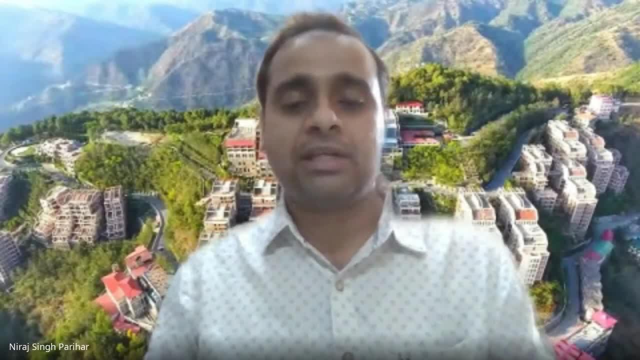 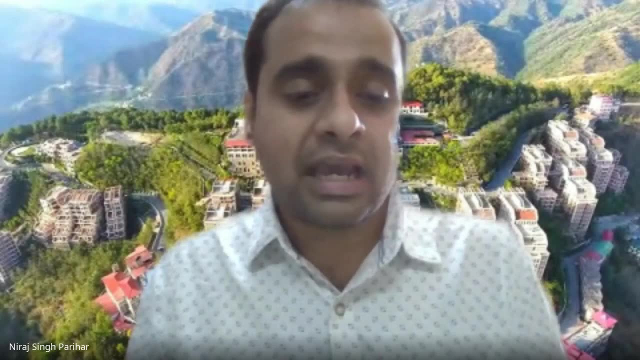 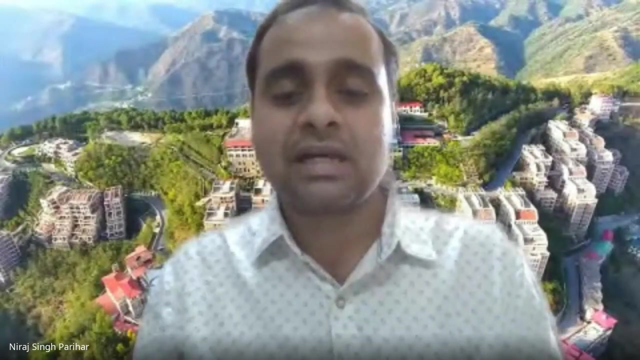 investigations in difficult soil conditions in Indian experiences. He also received the IGS Delhi Chapter Lifetime Achievement Award in 2012 and he is the active member of both BIS and IRC Corps of Economics. He has a number of achievements and committees. he is also the member on transportation, geotechnics, ISSM, GE and 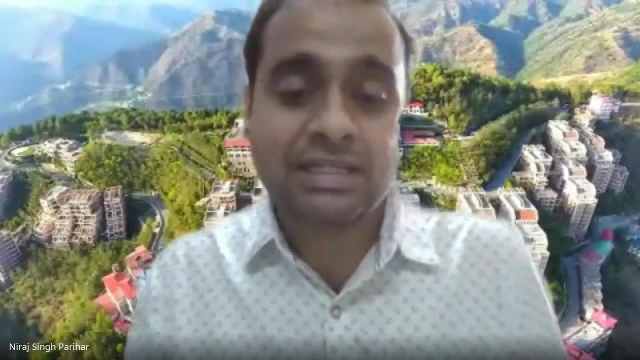 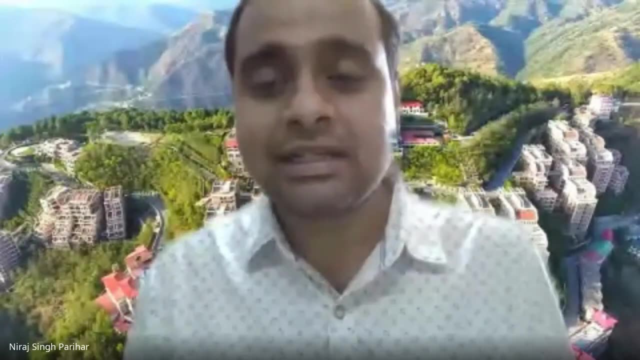 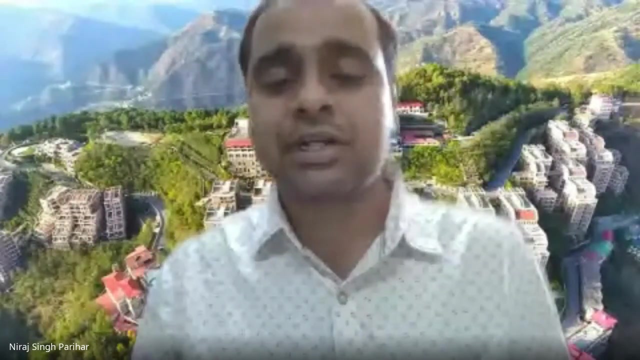 also working as executive committee member of ideas main body at present. so, with this note, I would like to invite mr Ravi Sundam sir to kindly take the main stage and request him to proceed with the first lecture of this geotechnical webinar series: advanced texting technologies for geotechnical 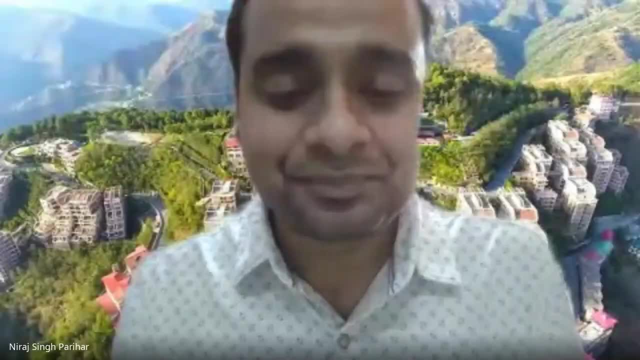 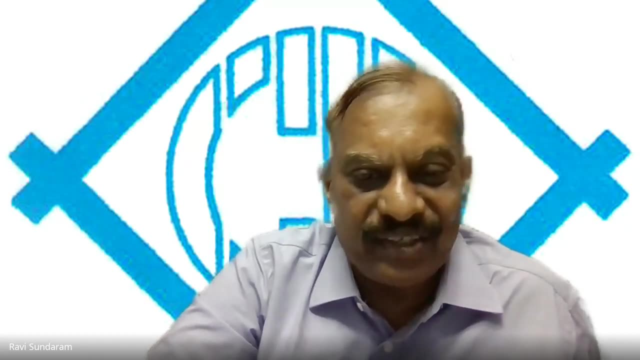 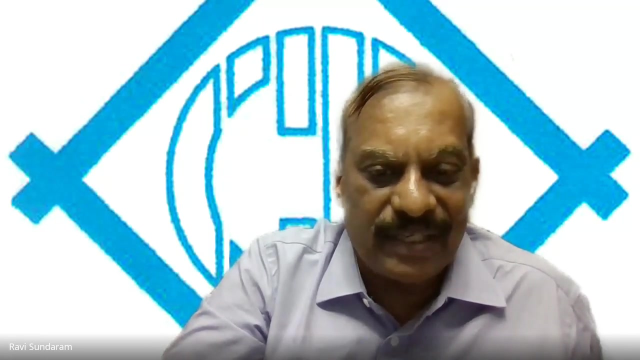 investigation over to you, sir. thank you, dr Parrihar. really grateful to you for that introduction. at the outset I would like to thank ideas, Shimla chapter and J UIT for inviting me Senja's to organize this event. a series of seven lectures is. five lectures is something which you know. 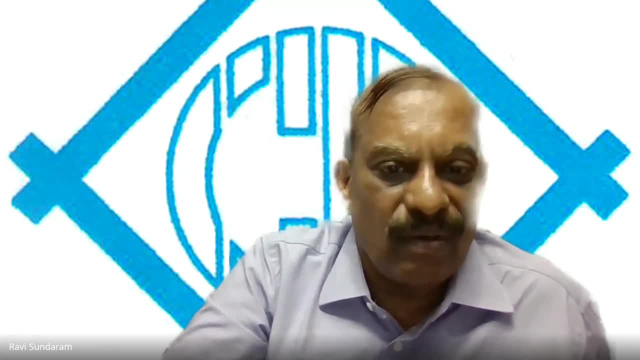 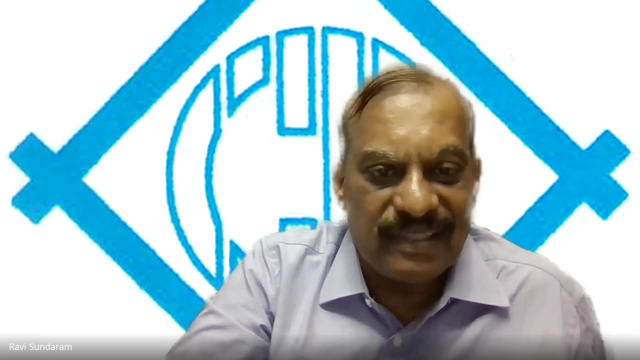 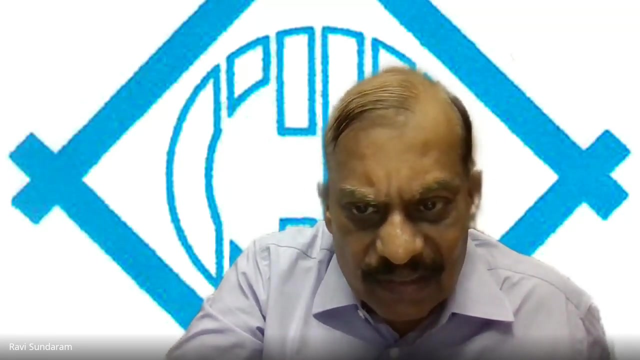 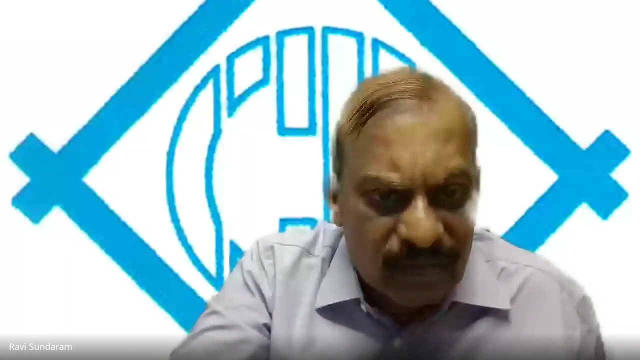 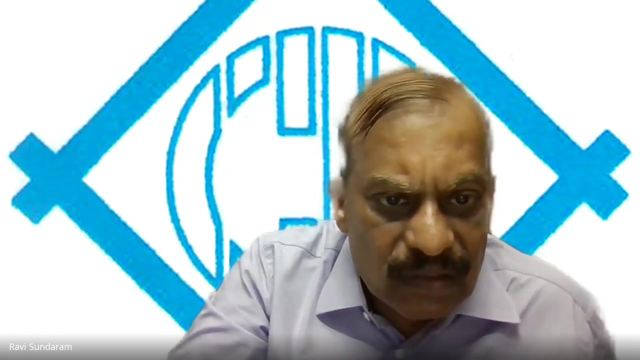 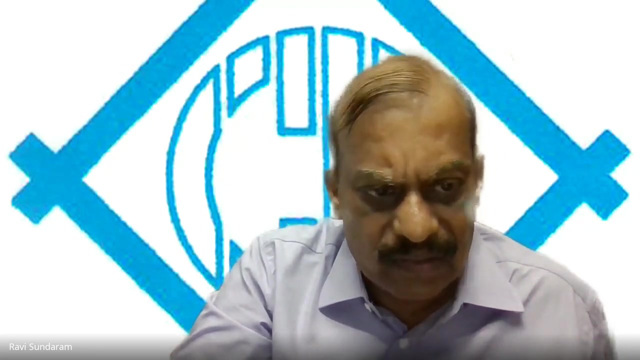 really special for us to organize and we are really grateful to you that Senja's has been invited to deliver all these seven, five events, five lectures, and so I am now sharing my screen. you I'm able to share, so you can kindly share your full screen, I mean your entire screen. okay, let me. 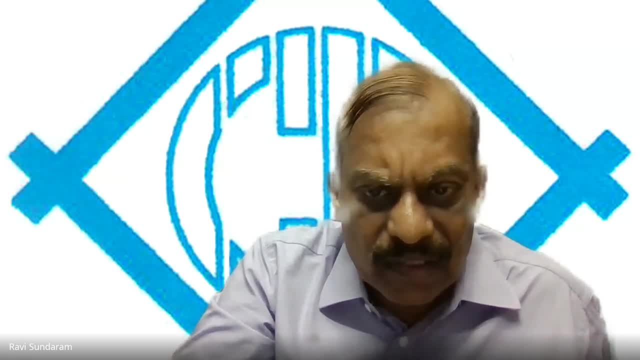 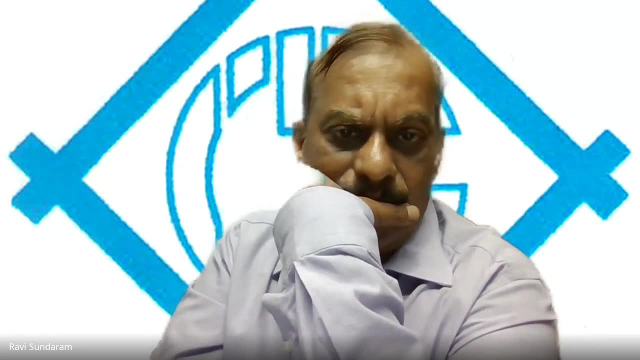 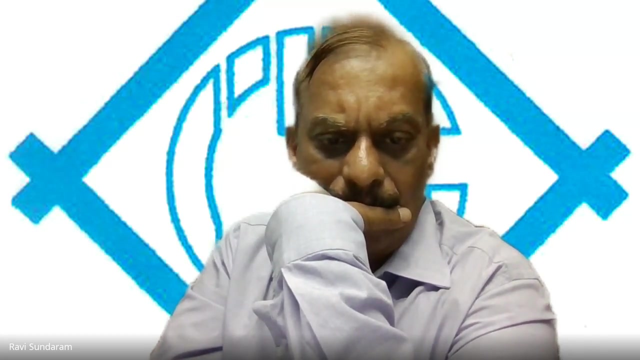 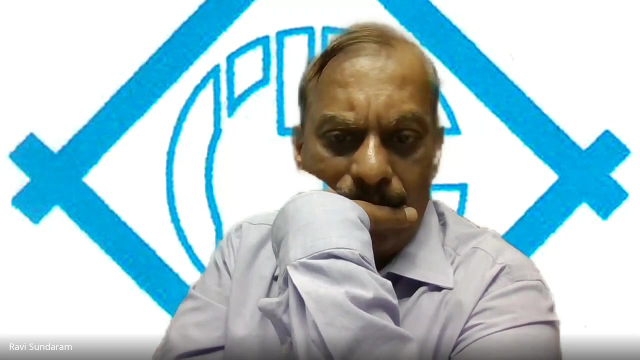 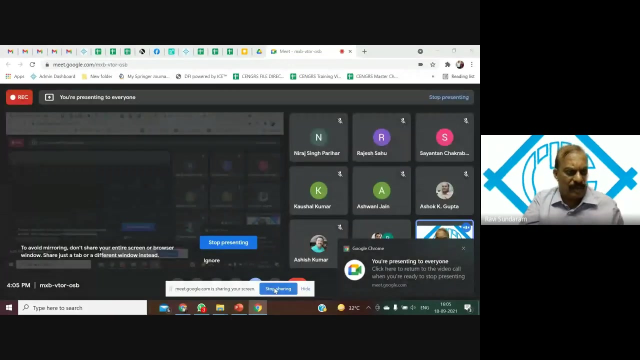 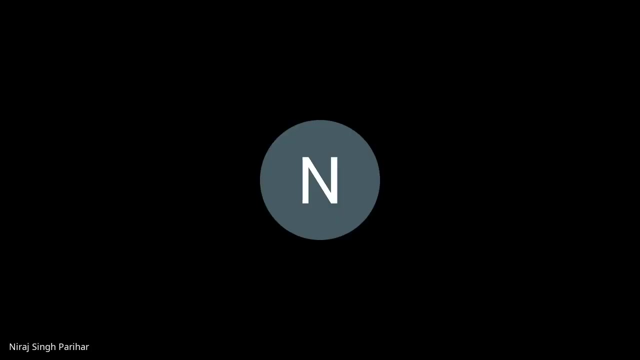 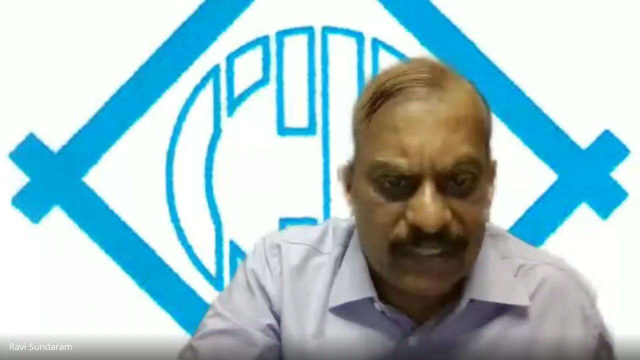 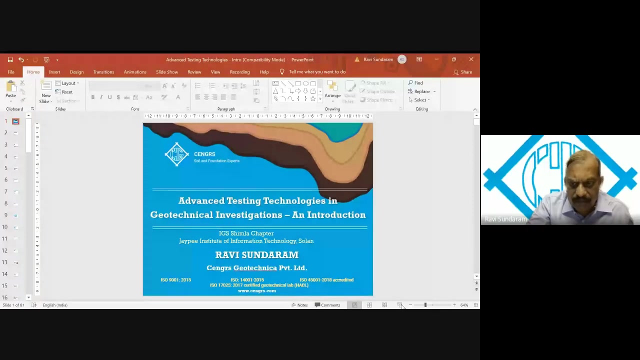 try again my entire screen, but it's not showing my presentation. how is this gonna be? it's only sharing the. yes, sir, now your screen is visible. your screen is visible. Can you see my screen now? Yes, sir, It's now visible. Is it on presentation mode? 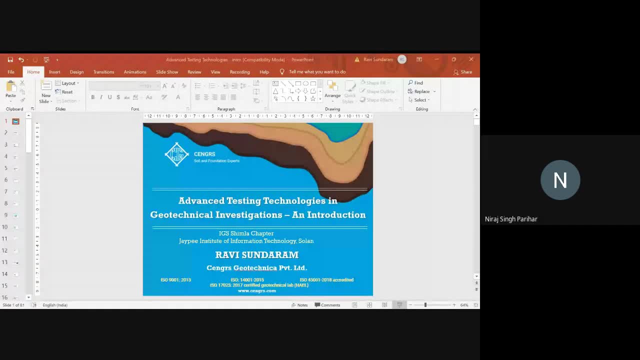 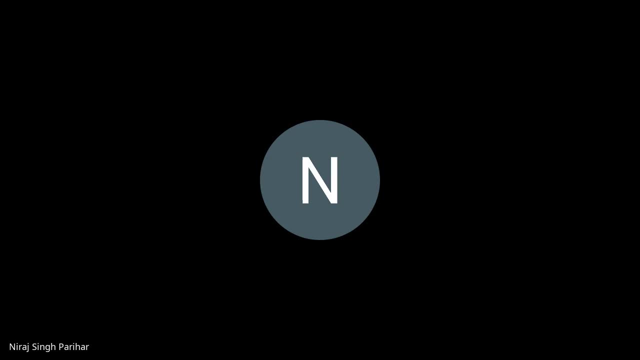 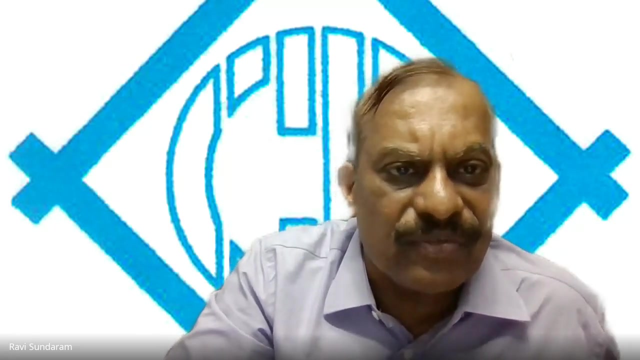 No, still not, sir. Sir, are you presenting entire screen? Yes, I'm presenting a window. No, sir, You have to present the entire screen. Then only it will go to the presentation mode, But on the entire screen it's only showing the screen of the lecture here. It is not going to my presentation. 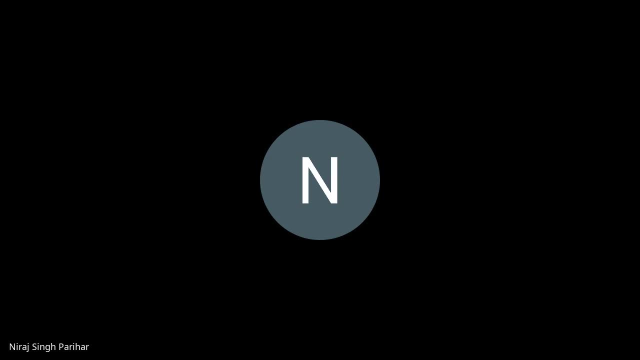 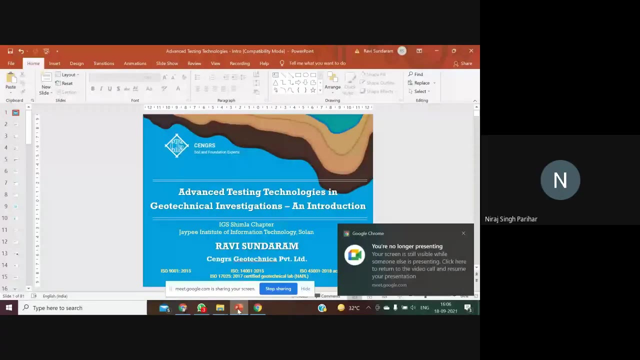 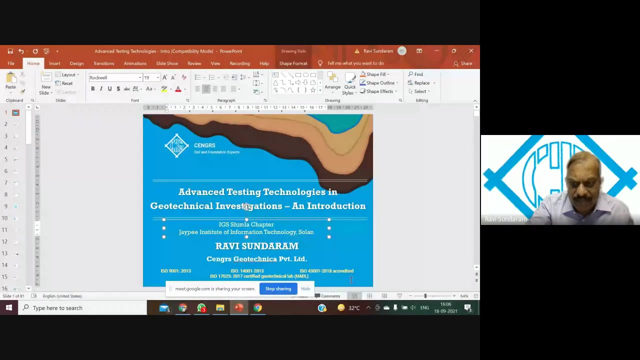 Sir, once you will click on that next, you can go anywhere onto your presentation mode also. Okay, You just need to click once there. Okay, Now can you see my screen? Yes, we can see your screen, sir, And you can see my presentation. 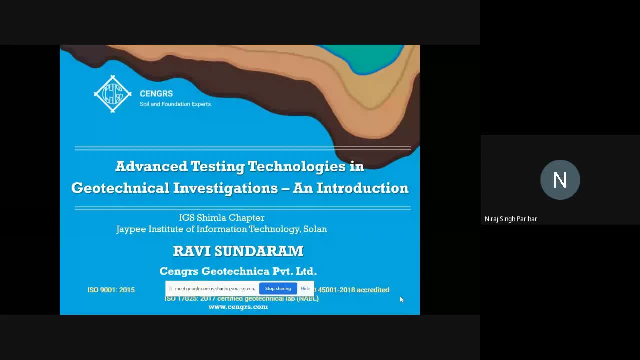 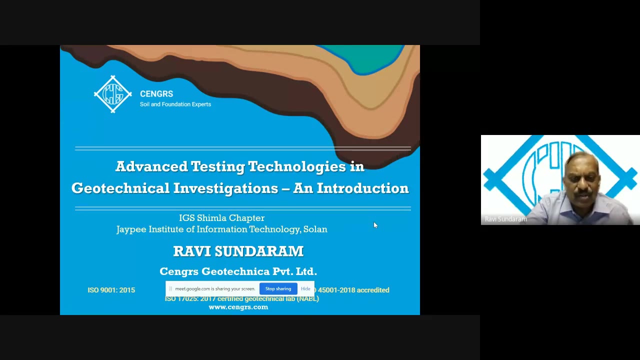 Yes, Now it's correct, sir. It's okay now. Is it on presentation mode? Yes, sir, Oh great, It's pretty fine, Okay. So this first lecture today is on an introduction to advanced testing technologies And geotechnical investigation. 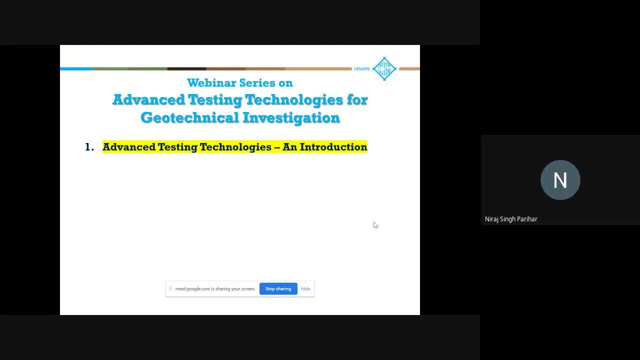 So can you see the screen here? Yeah, Great, Yes, sir. So this first lecture is on introduction And then the next one will be on static cone penetration test by Mr Saurav Gupta. Then Mr Sanjay Gupta will be presenting on pressure meter test in geotechnical design. 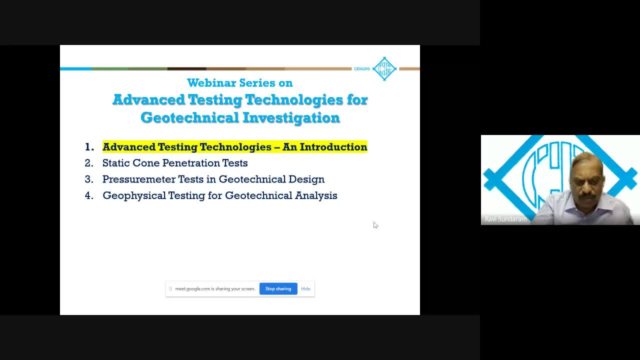 The fourth one will be by me, on geophysical testing, And the last one energy measurement for SPT. This is the latest technology which is now being adopted in India. This will be presented by Mr Ankit Uniyal. All these technologies will be illustrated by case studies to demonstrate the field application and the engineering benefits you can get by using these technologies. 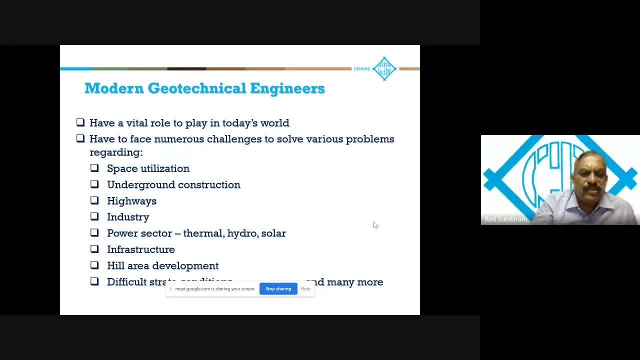 So, as you know, modern geotechnical engineers have a vital role to play in today's world. They have to face numerous challenges to solve various problems regarding space utilization: underground construction, highways, industry, power sector, thermal, hydro, solar infrastructure development, hill area development, difficult strata conditions. 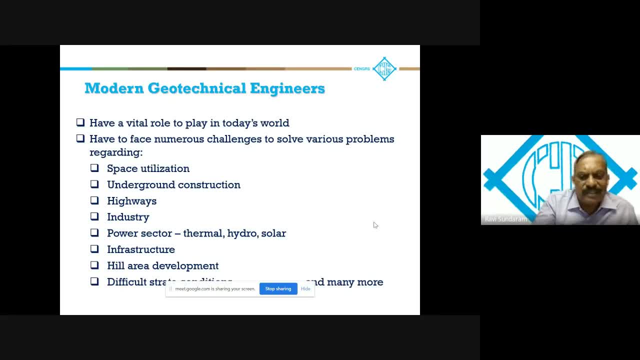 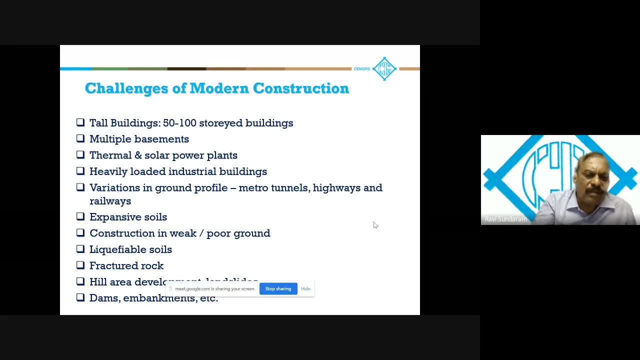 And many more. This list goes on. The challenges of modern construction include tall buildings, 50 to 100-story buildings, multiple basements, power plants, heavily loaded industrial buildings, variations in ground profile. you know particularly metros, highways and railways. 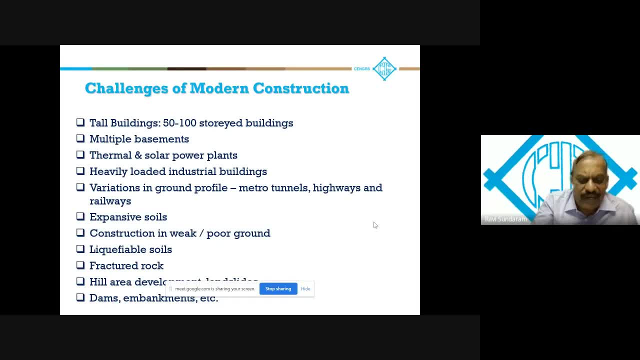 And the ground profile is different And the stratigraphy changes along the alignment. Yeah, So the design has to keep changing according to that. Then: expansive soils, construction in weak and poor ground, liquefiable soils, fractured rock hill area development dams, embankments. 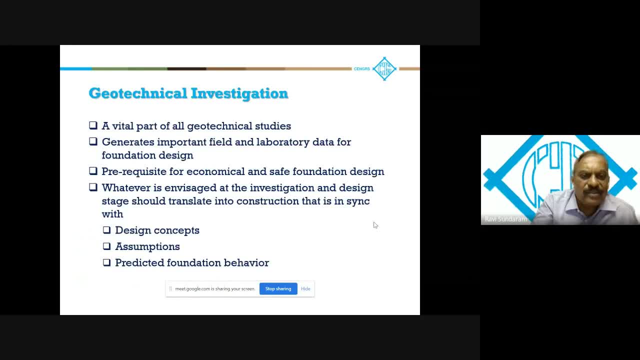 The list goes on here also. So geotechnical investigation, of course, is a vital part of all geotechnical studies. It generates important field and laboratory data for foundation design. It's a prerequisite for economical and safe foundation design. Whatever is at the investigation stage and the design stage, this has to translate into construction that is in sync with the design concepts, the assumptions and the predicted foundation behavior. 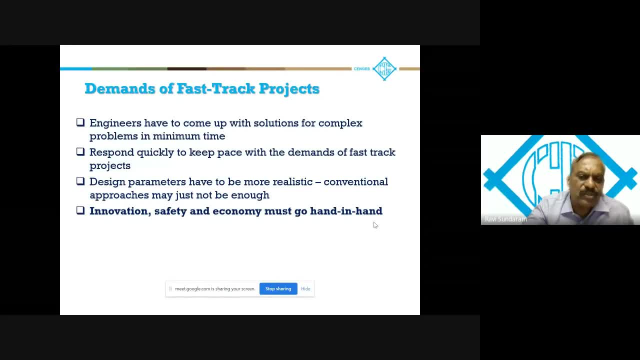 Engineers have to come up with solutions for complex problems within a minimum time. So the fast track projects. there is a real challenge nowadays. You have to respond quickly to keep pace with the demands of the fast track projects. Design parameters have to be more realistic. 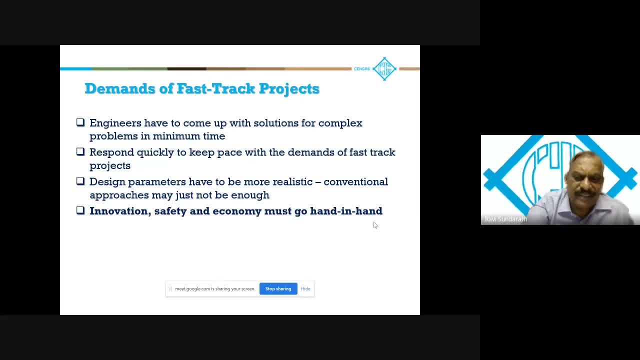 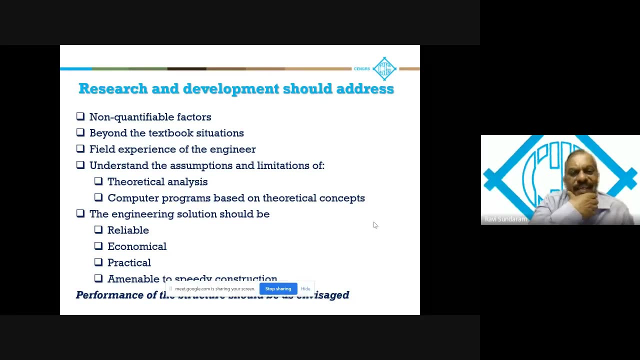 Conventional approaches. it's not just enough to be conservative. You have to go for innovation, safety and economy. These have to go hand in hand, Okay, So therefore, research and development should address non-quantifiable factors and beyond the textbook situations. 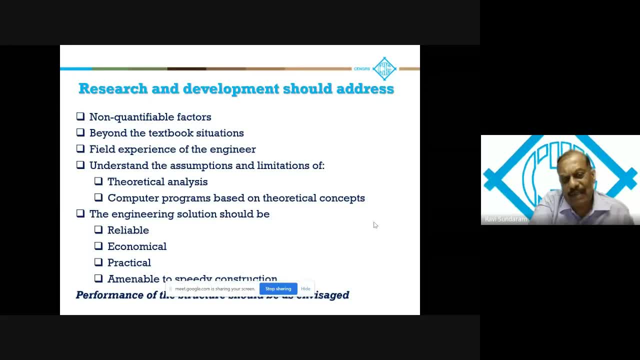 The field experience of the engineer becomes most important. You have to understand the assumptions and the limitations of theoretical analysis and computer programs based on theoretical concepts. Computer programs, softwares, are being used quite a lot, But the limitations are very limited. Okay, 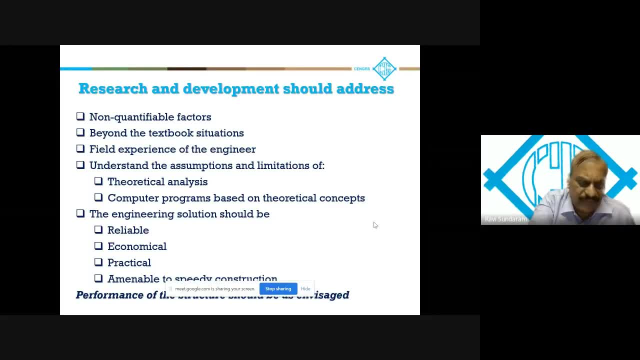 So you have to understand the limitations and assumptions that have to be clearly understood. The engineering solution which you develop has to be reliable, economic, practical and amenable to speedy construction, All this within the minimum period. The performance of the structure has to be as was envisaged. 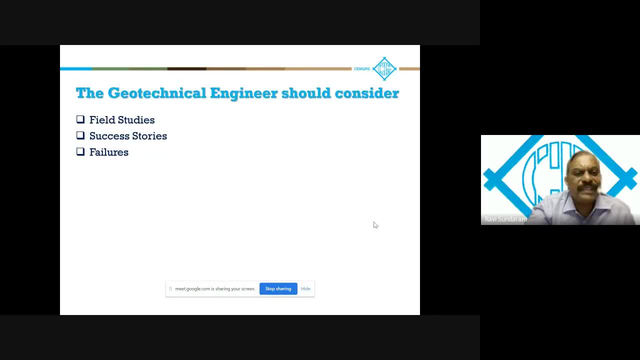 So the geotechnical engineer has to consider field studies, success stories and failures. The approach has to be systematic. The approach has to be systematic, flexible, proper choice of geotechnical investigation techniques and selection of suitable analysis methodology so that you get the right geotechnical parameters. 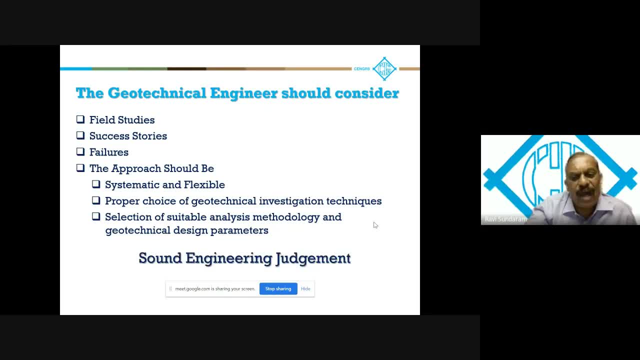 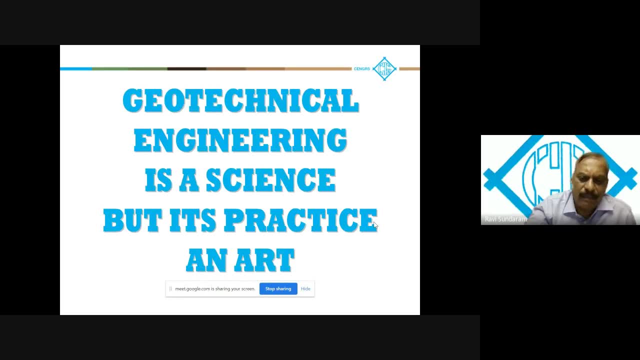 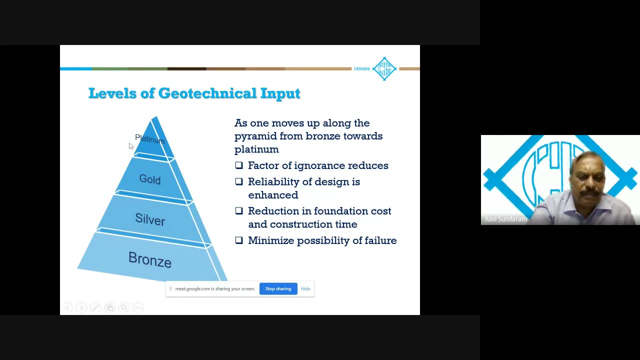 That's very critical. So what it requires is sound engineering judgment. So I'd like to highlight here that geotechnical engineering is a science, but it's practice and art. So this is called the geotechnical pyramid, geotechnical input pyramid. 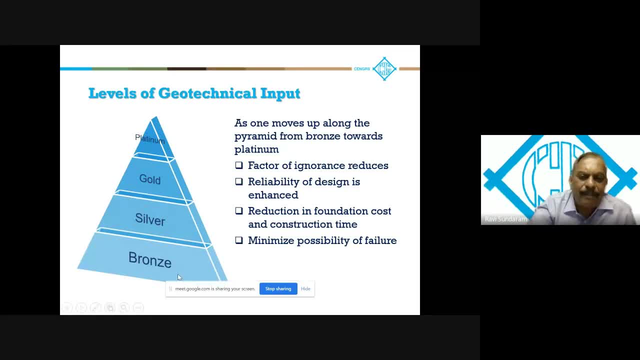 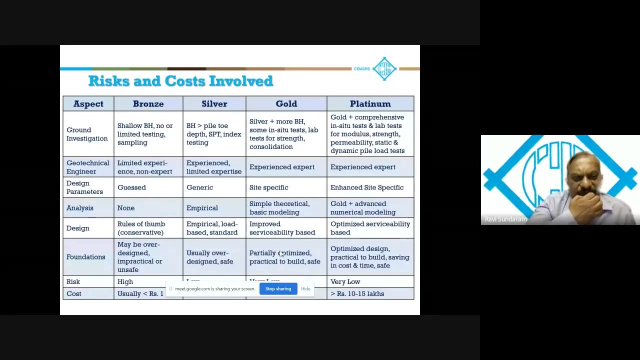 So, as you move up along this pyramid from bronze towards platinum, your factor of ignorance reduces, The reliability of the design is enhanced, There's a reduction in foundation cost and construction time, And you minimize the possibility of failure. So let us look at these bronze, silver, gold and platinum levels of investigation. 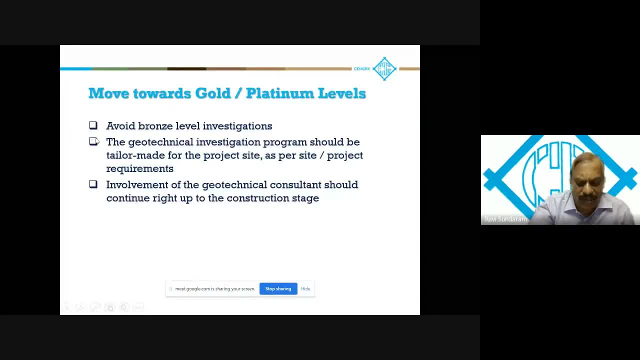 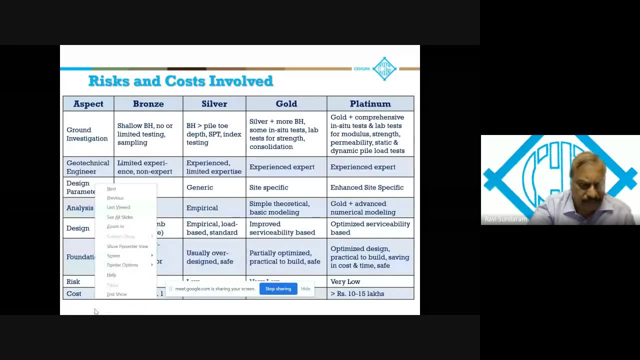 So a bronze investigation would have probably shallow boreholes, Very limited testing, Whereas if you move towards the silver you have deep boreholes beyond the pile tip. You conduct SPTs and limited laboratory tests. At the gold level you have more boreholes, more in situ tests like pressure meter maybe, or maybe static cone penetration tests, lab tests for strength and consolidation, et cetera. 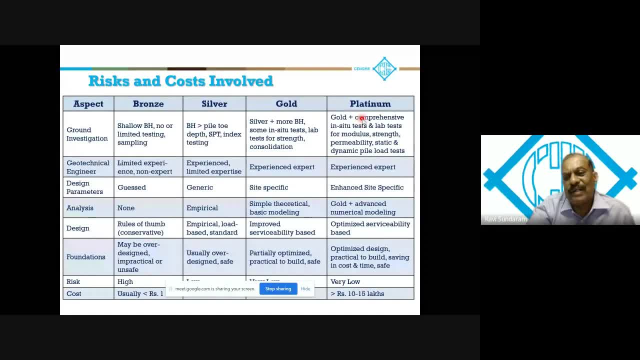 A platinum level would be a more comprehensive investigation with substantial in situ tests in addition to the boreholes, And maybe, if piles are required, you could go for static and dynamic pile load tests. The geotechnical engineer in a bronze level would have limited experience and non-expert. 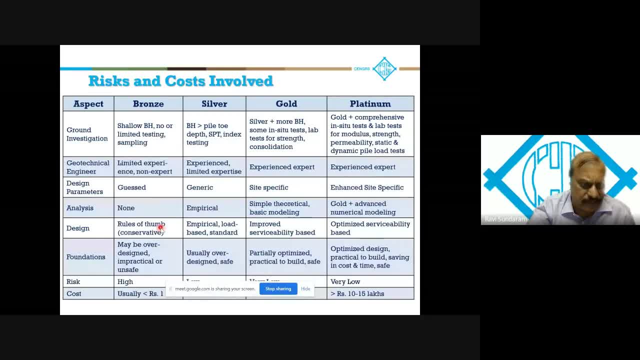 Whereas at a platinum level you have an experience. Similarly, design parameters in a bronze is primarily guessed, Whereas in a platinum level it is site-specific and site-specific The analysis design. these are all you know. as you move from bronze to platinum, you have an optimized design. 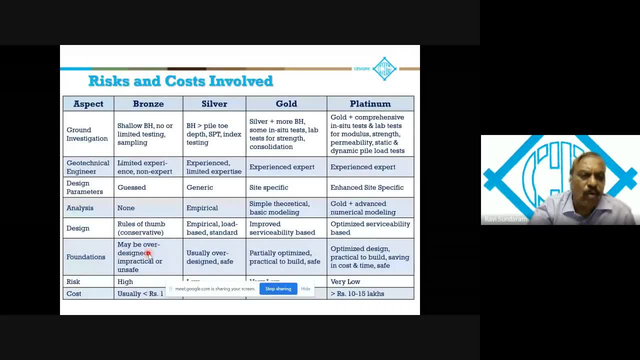 And the foundations may be over-designed or unsafe Or even impractical in a bronze level, And whereas in a platinum level it's an optimized design, practical to build, There is substantial savings in cost and time, Whereas the risks are low in a platinum investigation. 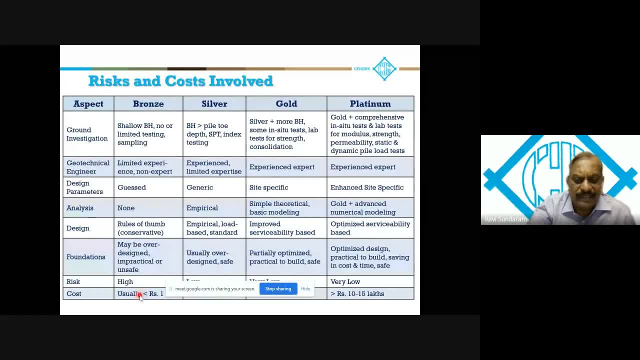 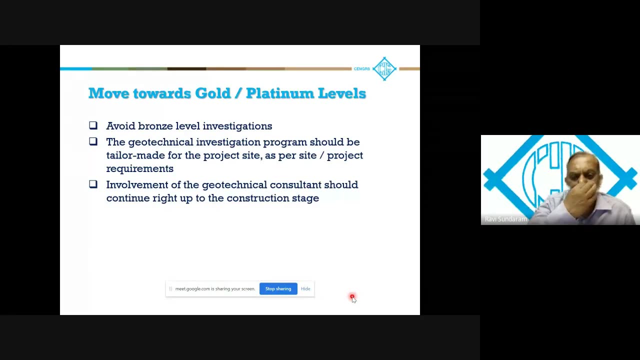 Obviously the cost is much more, But you should always remember that the amount spent in the investigation is very, very low. You save much more in the foundation cost. So we must move towards gold and platinum levels, Avoid bronze level investigations. The investigation should be tailor-made for the project site as per the site requirements. 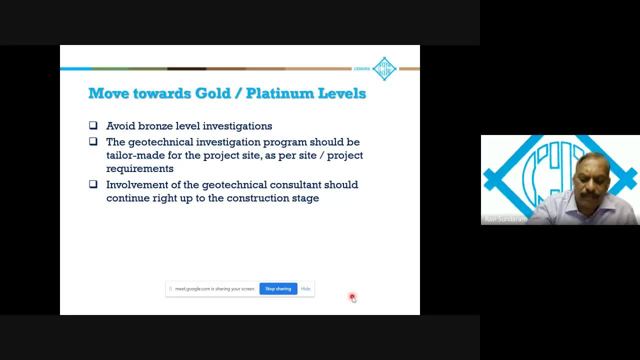 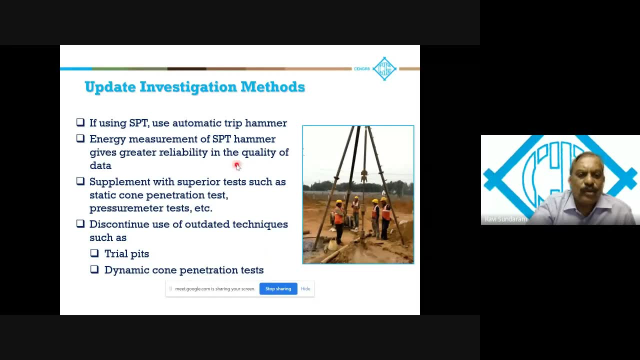 So involvement of the geotechnical consultant should continue right up to the construction stage. So the investigation methods need to be updated. If you are using SPT, go for an automatic trip hammer. Energy measurement in the SPT hammer gives greater reliability in the data and the quality of the SPT. 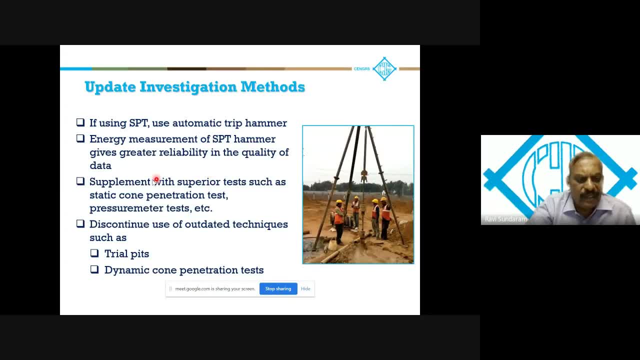 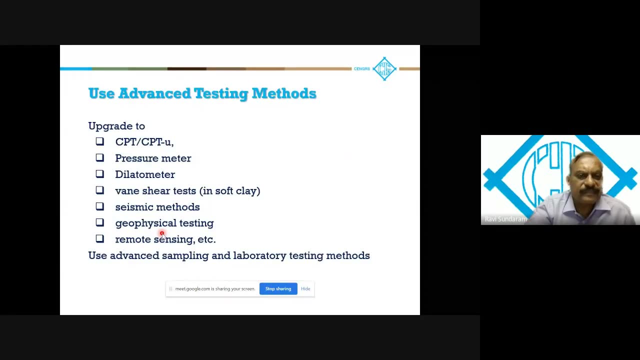 So you can see the automatic trip hammer here. You have to supplement it with superior tests like static cone penetration tests, pressure meter tests, etc. And discontinue outdated techniques such as trial pits, dynamic cone penetration tests, etc. Use advanced testing methods. 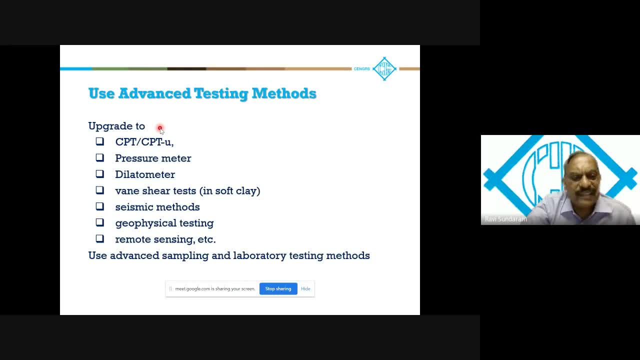 Upgrade to cone penetration tests. This would be the static cone penetration test, with or without pore, water pressure measurement, Pressure meter tests, dilatometers, rain shear tests, seismic methods, geophysical testing, remote sensing, advanced sampling and laboratory testing methods. 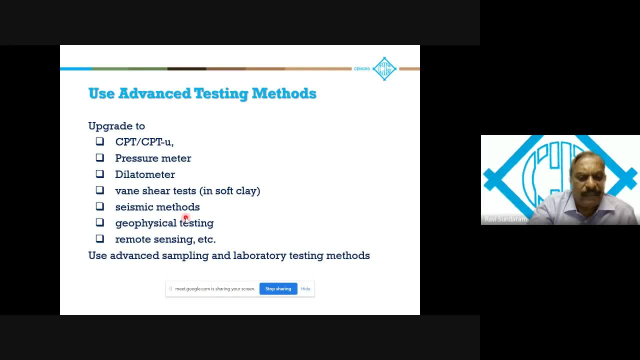 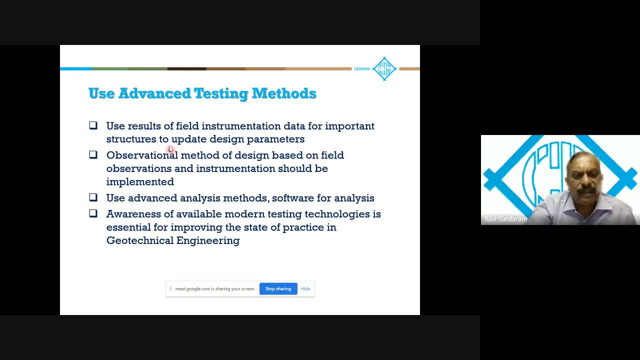 So there are various techniques available, But of course we shall be limiting to a few of them only here. Most important thing is to use field instrumentation data for important structures to update the design parameters. Observational method of design based on field observations and instrumentation. 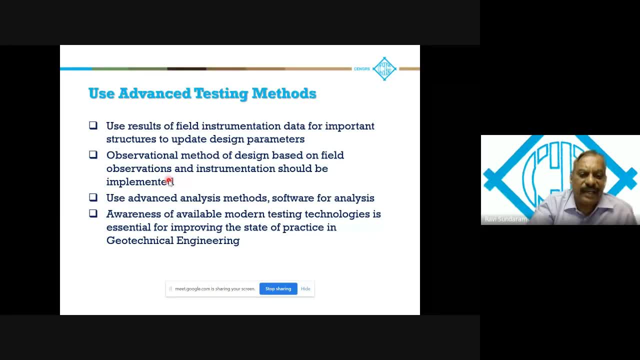 If you can implement this, you can do your design very economically. Use advanced analysis methods. These methods and softwares are available for analysis, And modern testing technologies is essential for improving the state of art, the state of practice, of the geotechnical engineering. 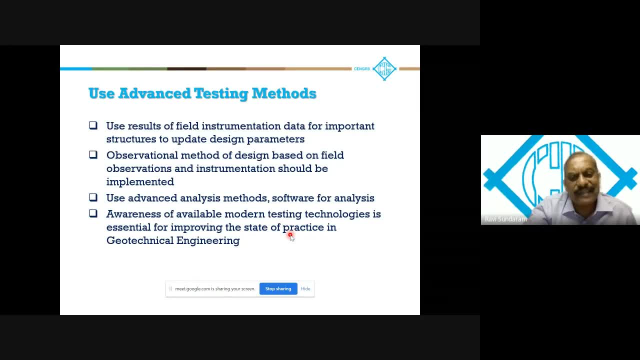 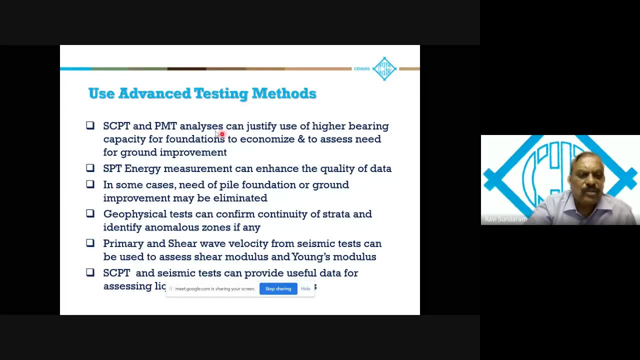 So I'd like to differentiate between the state of art and state of practice. So in the state of practice it's what you actually do there. So static cone penetration test and pressure meter test can justify use of higher bearing capacity, performance And economize so as to assess the need for ground improvement. 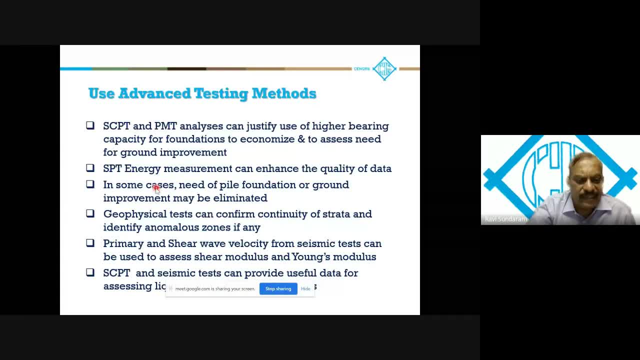 SPT measurement can enhance the quality of the data. In some cases, need for pile foundation or ground improvement may be eliminated. Geophysical tests can confirm continuity of the strata, identify anomalous zones if any Primary and shear wave velocities from seismic tests can be used to assess the shear modulus and Young's modulus. 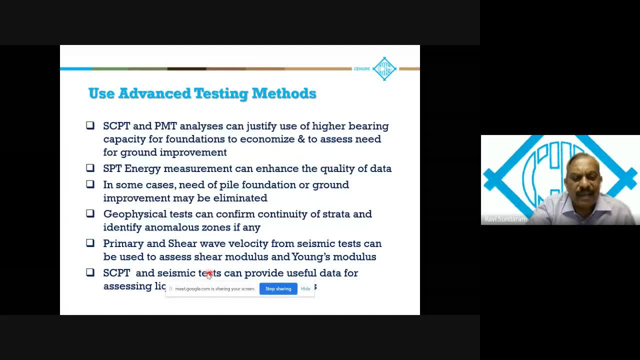 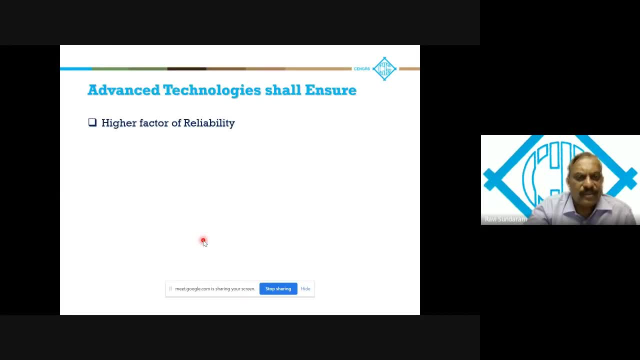 Static cone penetration tests and seismic tests can provide useful data for liquefaction analysis during earthquakes. So advanced technologies will assure higher factor of reliability as a factor of safety, Economical and safe foundation design. It will model the foundation behavior realistically So that the performance of the structure 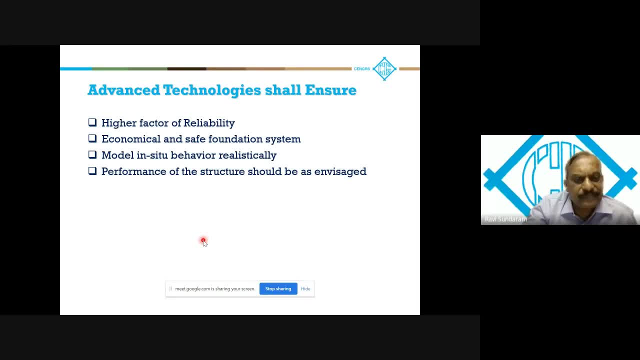 Is as envisaged at the design stage. So thus you can add value to geotechnical exploration and enhance the quality of design. So just covered in this webinar series: Cone penetration test using mechanical cone as well as using electric cone with pore water pressure measurement. 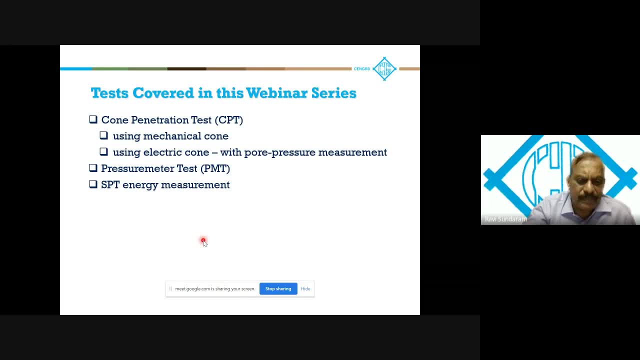 Pressure meter test and SPT energy measurement. Geophysical tests include electrical resistivity test, cross hole seismic test, seismic refraction test and spectral analysis of surface waves, That is, SASW test. So just introduction to the static cone penetration test, The mechanical cone as well as the electric cone with pore water pressure measurement. 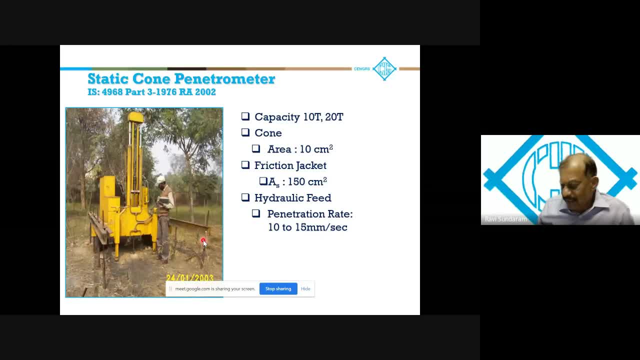 The conventional cone penetrometer Which is used In the country. This is the mechanical cone system. 10 ton and 20 ton systems are available. The cone usually has a cross sectional area of 10 square centimeter And a friction jacket of 150 square centimeter. 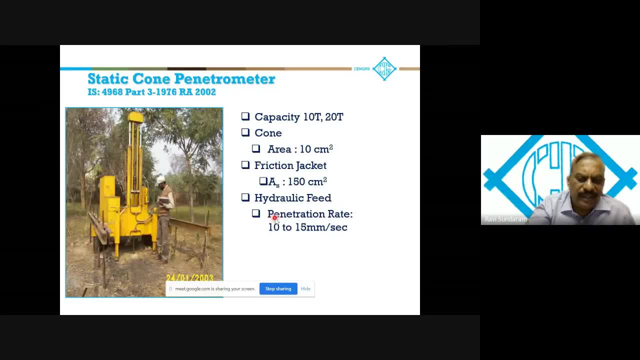 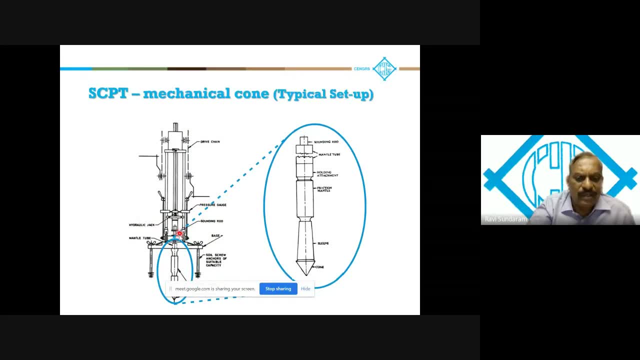 It has a hydraulic feed And the penetration rate is about 10 to 15 mm per second. So this is the mechanical cone, So you can have a look at details of the cone. So you have the cone here And the friction sleeve here. 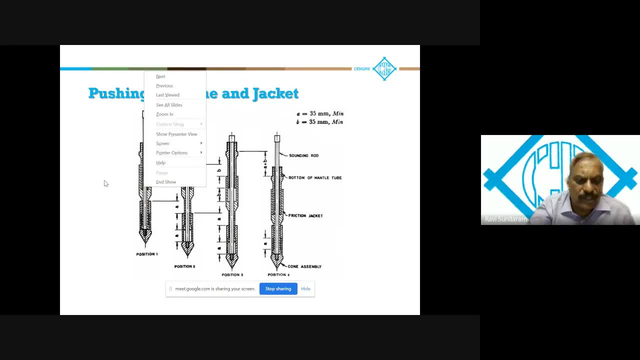 So in the first you would push the cone only, And then in the third position you are pushing the cone and the jacket together, And then this is the total system being put to the next level. So normally there is a 5-5 centimeter penetration here. 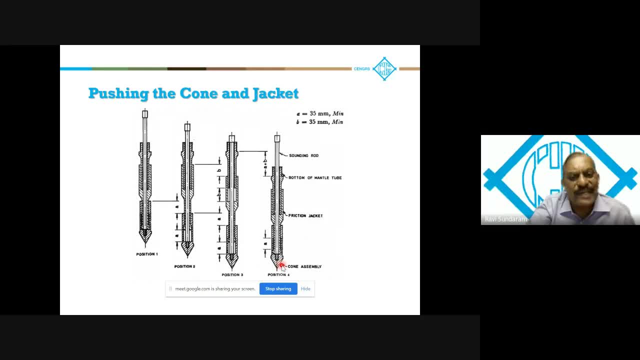 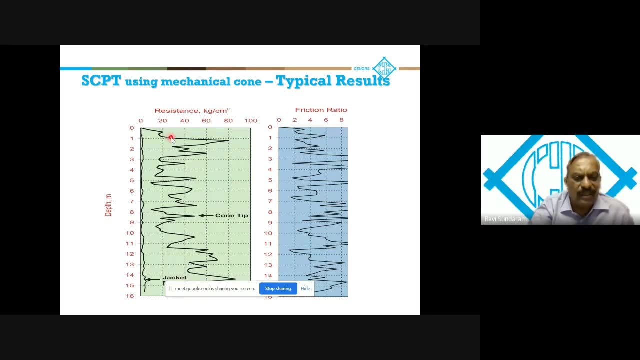 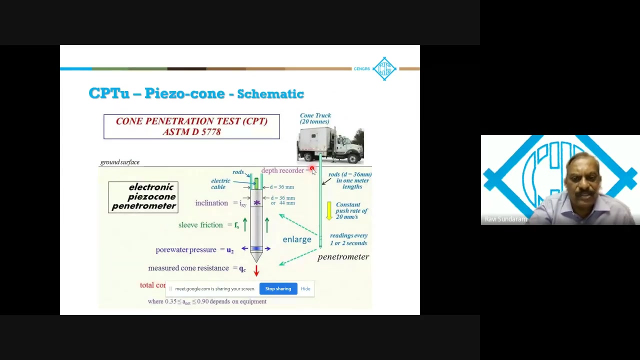 And then a 10 centimeter penetration. Total 20 centimeter penetration. So you measure the cone tip resistance and the friction resistance. Typical results using a mechanical cone. So you get the cone tip resistance and the friction ratio versus depth. This is a piezo cone. 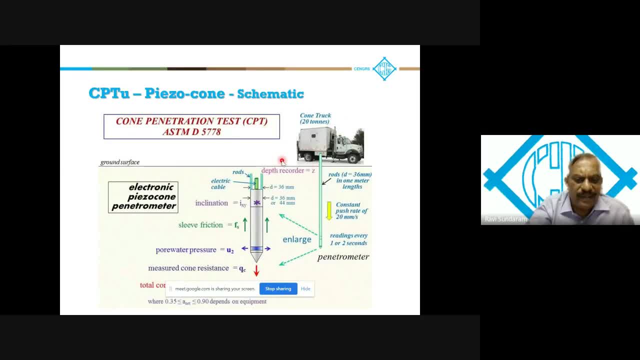 So here you have a Pore pressure measurement system here At just above the cone, And you have a data acquisition system By which you can measure the cone tip resistance, The pore water pressure As well as the sleeve friction. So this is a typical piezo cone. 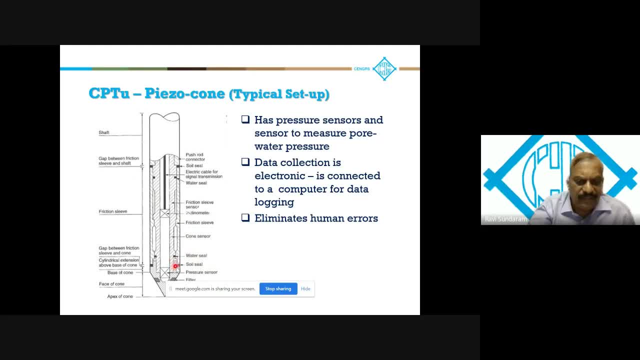 You can see here The pressure sensors And the friction sleeve And the You have at the base of the cone. You have the For the pore water pressure. So the data is collected electronically Connected to a computer. It eliminates human errors. 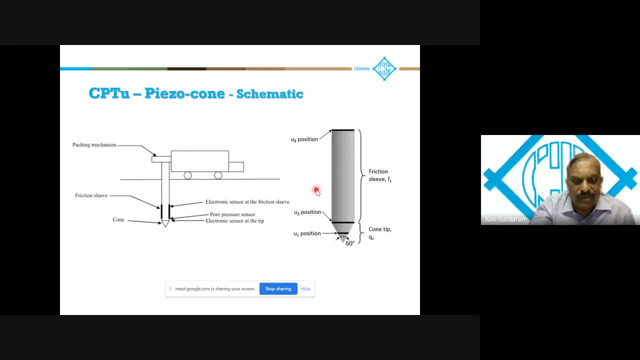 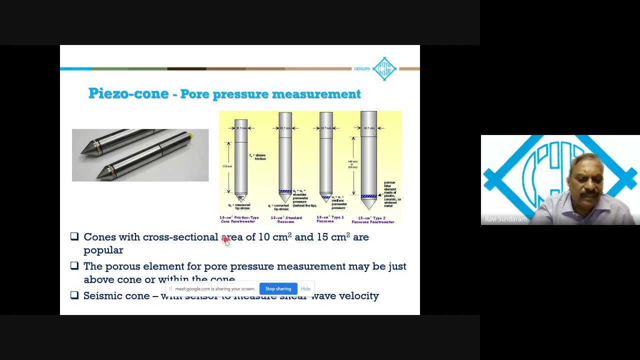 So this is the schematic of the piezo cone. Usually only the U2 is used, Although you could have a Sensor at this position also. Cones with cross sectional area of 10 square centimeter And 15 centimeters square. 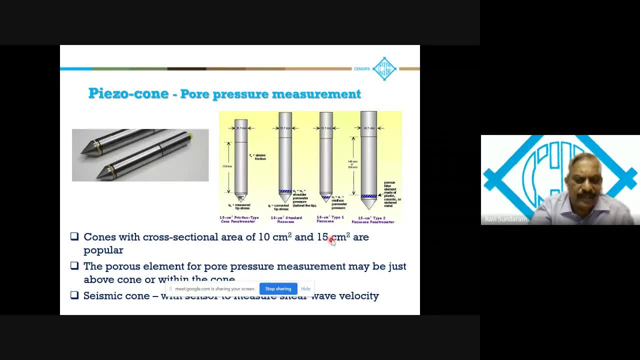 Both are popular. The 15 centimeter square is Getting more popular nowadays, The porous element. For the pore pressure measurement, Maybe just above the cone Or within the cone, as I told you, There is another small variation Called the seismic cone. 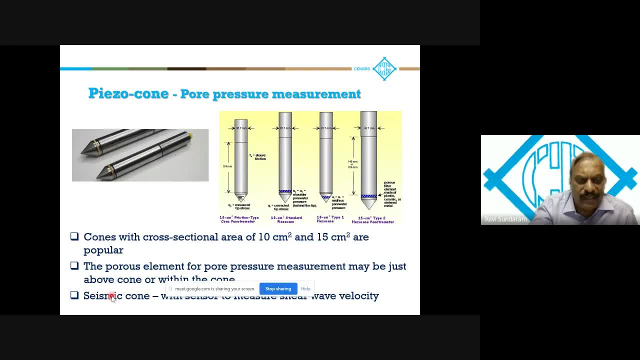 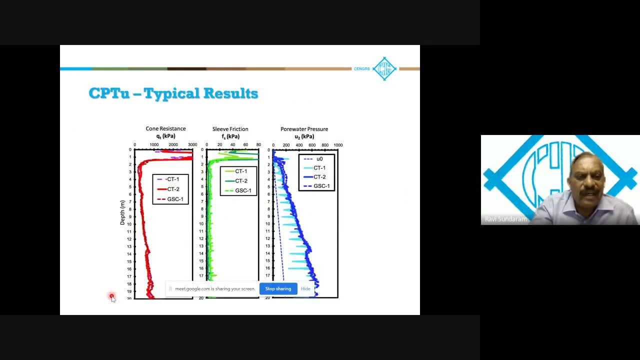 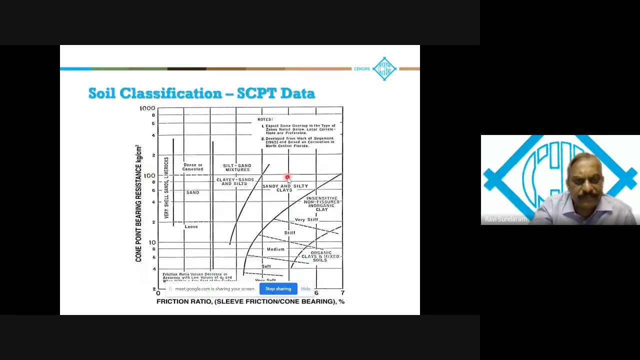 With a sensor to measure the shear wave velocity, So that is also Being used internationally now. Typical results of the Cone penetration test. You have the cone resistance, The sleeve friction And the pore water pressure Being measured. The soil classification based on 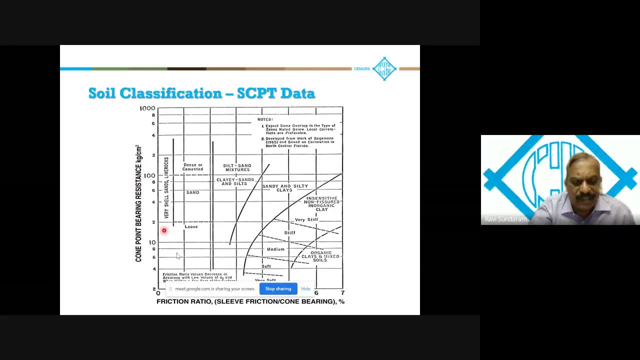 The SPD data. You have cone tip resistance. What is the friction ratio? So the low friction ratios Indicate sand And the higher Indicate the clay content. And, of course, very high Friction ratios would mean It could be organic material. 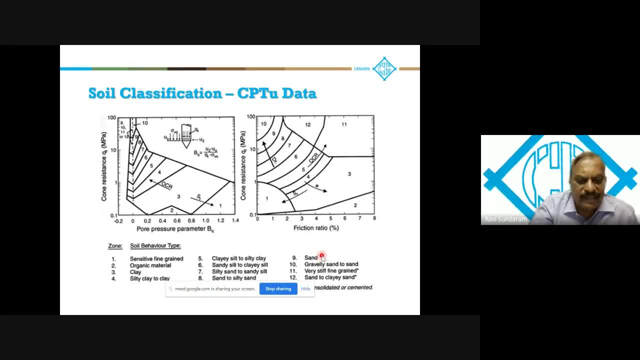 This is the interpretation Of the CPTU data With the cone With pore water pressure measurements. So there is. You measure The pore pressure parameter Bq And this is related to the cone tip resistance, And you can see these different zones. 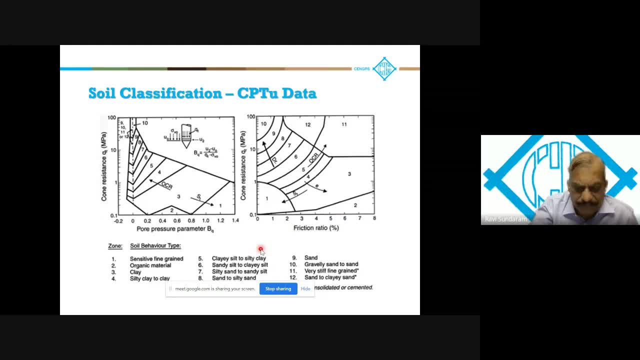 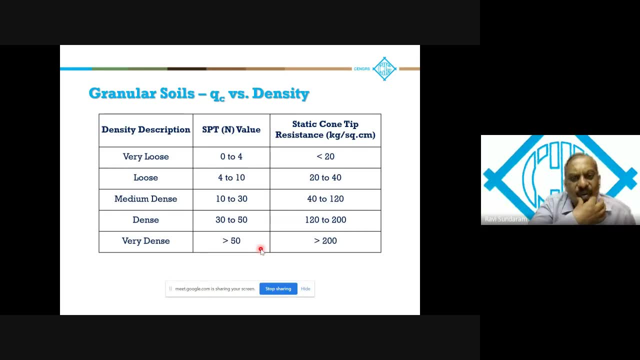 This classification is done And similarly with the friction ratio. Correlations are available For You know: cone tip resistance And SPT values versus density. So right from very loose, With the cone tip resistance of Less than 20 kg per centimeter square. 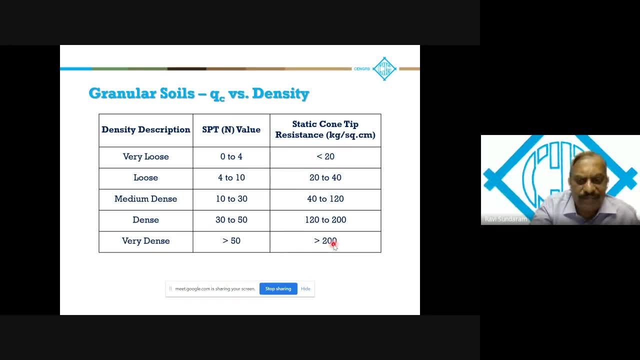 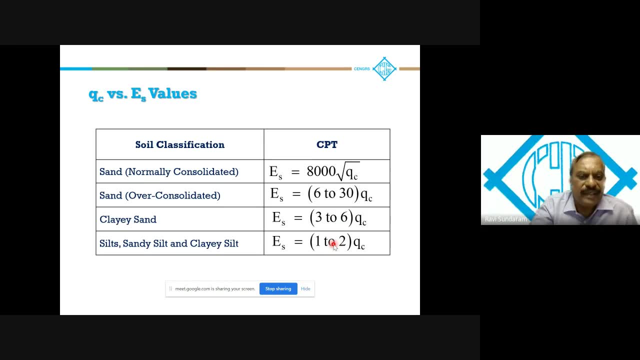 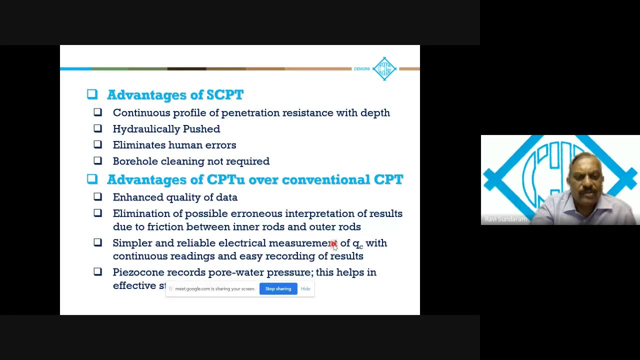 To very dense, Where you have very high values Of cone tip resistance. These correlations are available And also you can Indicate the E values with the Qc. Advantages here Is that You get a continuous profile. 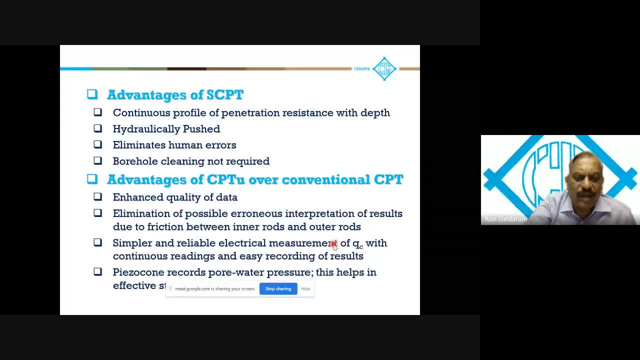 Of penetration resistance versus depth And since it is Hydraulically pushed, It eliminates the human errors And borehole cleaning is not required. And if you were to use CPTU With the pore water pressure measurements, The advantage Is that you get enhanced quality of data. 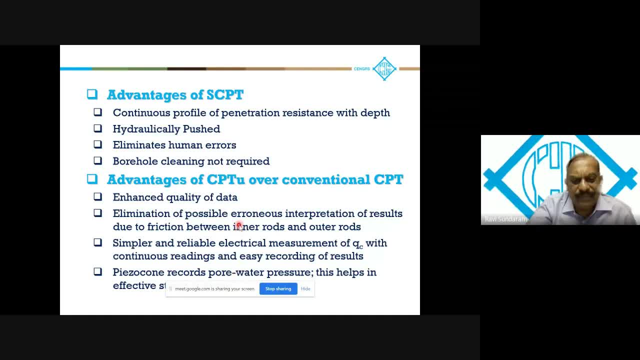 And elimination of error Due to, You know, erroneous interpretation, Due to friction between the inner and outer rods. All these Possible errors are eliminated. It's a simple and reliable Electrical measurement With easy recording The pore water pressure Effects. 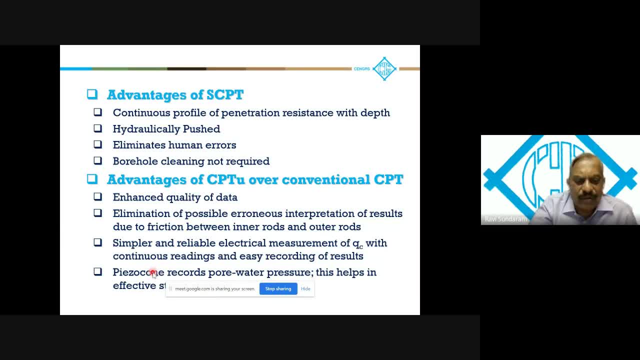 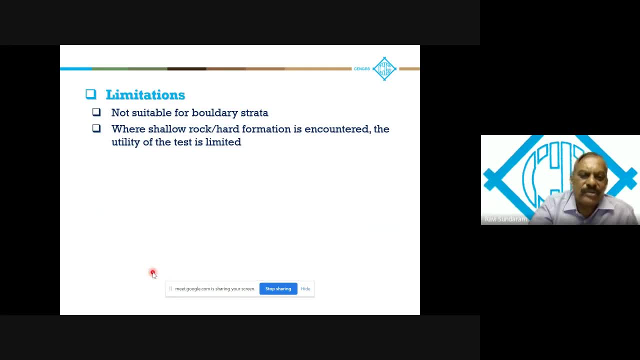 Is very helpful In the foundation design, In the Assessment of what kind of Behavior it is going to have. But of course it has limitations. It's not suitable Where boulders are Met or If you are having shallow rock. 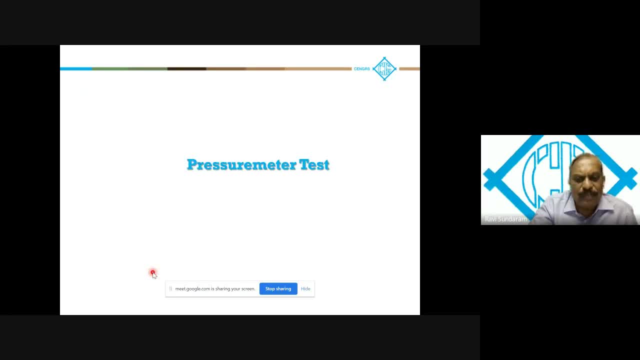 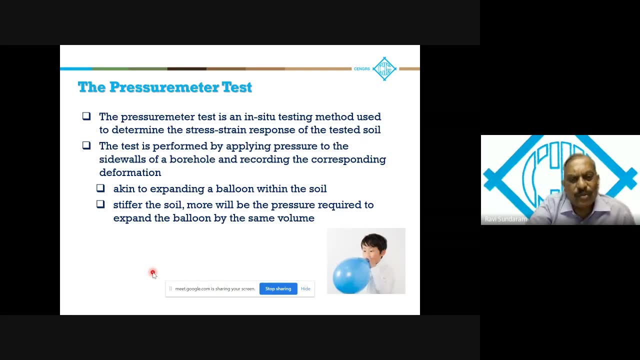 The utility is limited. I move on to Pressure meter test. The pressure meter test Is an in-situ test To determine the stress strains Response of this soil. It is performed By applying a pressure to the Sidewalls of the borehole. 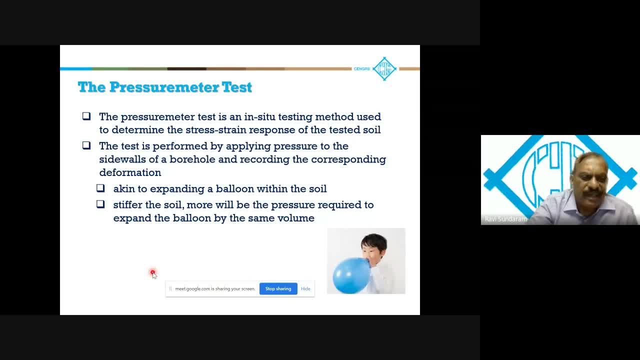 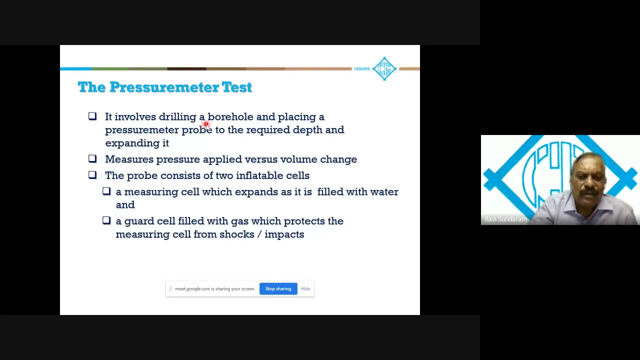 And recording the corresponding Deformation. It is akin to expanding a balloon Within the soil. The more pressure will be required To expand the balloon By the same volume. So it involves Drilling a borehole, Placing a pressure meter probe. 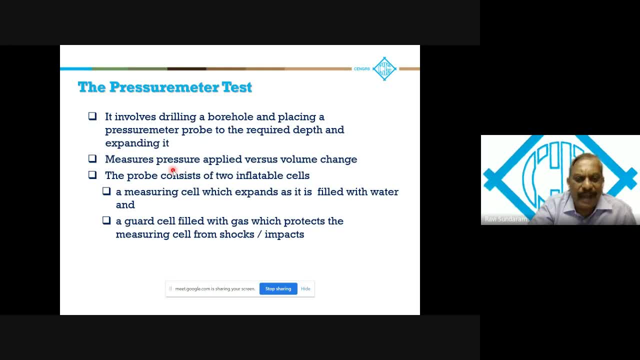 At the required depth And then expanding it To measure Pressure versus volume change. So the probe consists of Two inflatable cells: A measuring cell which expands As it is filled with water And a guard cell filled with gas. It protects the measuring cell. 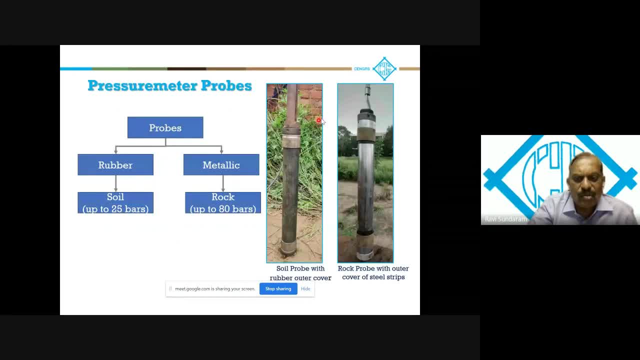 From shocks or impacts. So These are the Probes You have a rubber probe For Pressures up to 25 bars And a metallic probe, A metallic outer cover For pressure up to 80 bars. Units up to 200 bars. 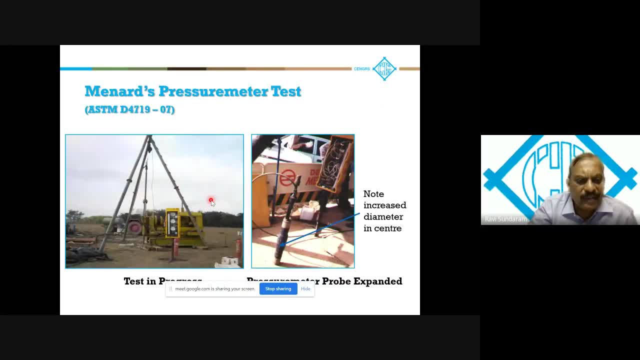 Are also available In the industrial market. So it's a typical Pressure meter Control panel And You can see the probe here Being expanded. You can see the center is Having a larger diameter Because it has been expanded. 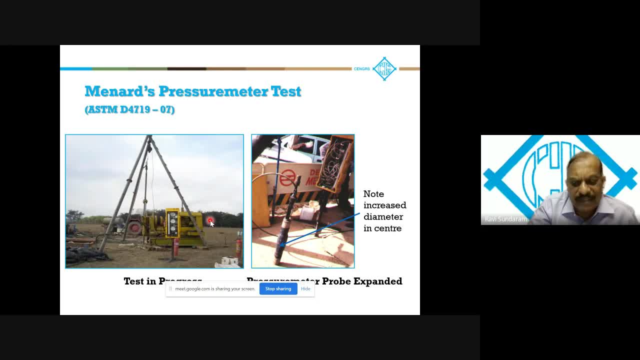 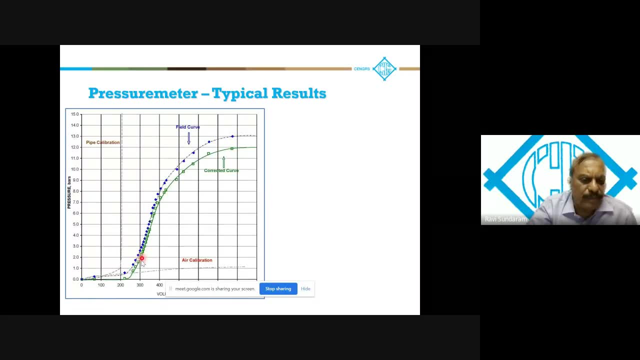 So This is the test In the presentation Two weeks from now: Typical results. So what you would be plotting Is pressure versus volume change. There is First, you would expand it in air To check what Pressure is required to expand it in air. 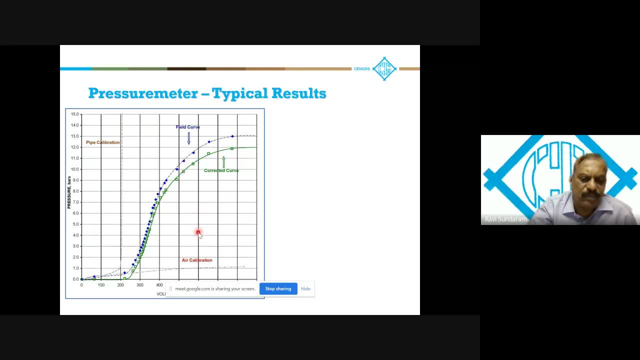 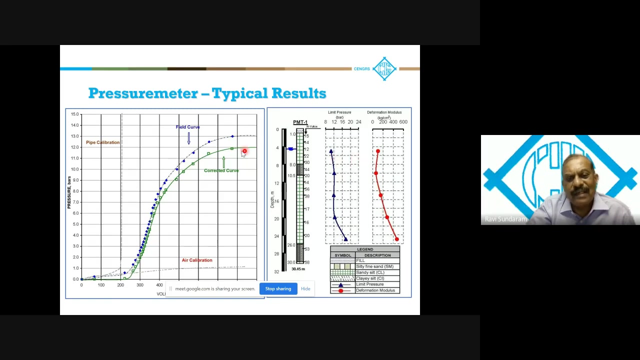 And then you expand it in The soil And the difference between the two Gives me the Pressure required to expand in the soil. it is also corrected for the expansion of the hoses by expanding it on a stiff pipe- typical results. so what you would be measuring. this is called the limit pressure, the maximum pressure. 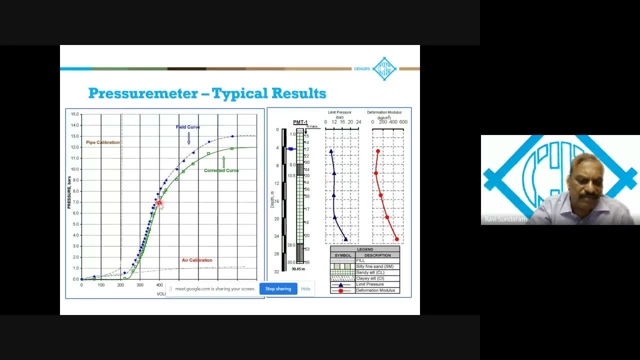 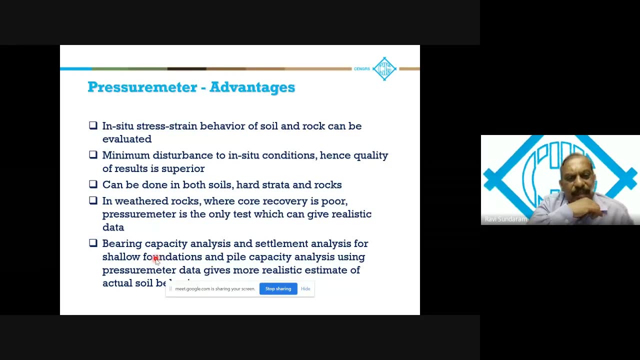 that you can apply, and the deformation modulus is a function of the slope of the straight line portion of the graph, so you could plot this versus depth. the in situ strain- be stress strain- behavior of the soil can be evaluated and there's a minimum disturbance to in situ soil conditions. therefore, 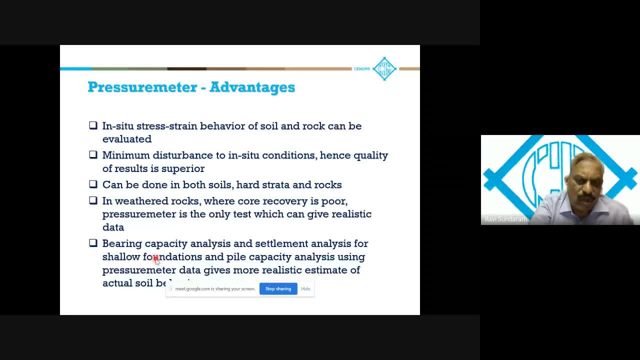 the quality is superior can be done in both soils, hard strata and rocks. in weathered rocks, where the core recovery is poor, pressure meter test is the only test which can give you realistic data: bearing capacity analysis and settlement analysis for foundations and pile capacity analysis using pressure meter data gives. 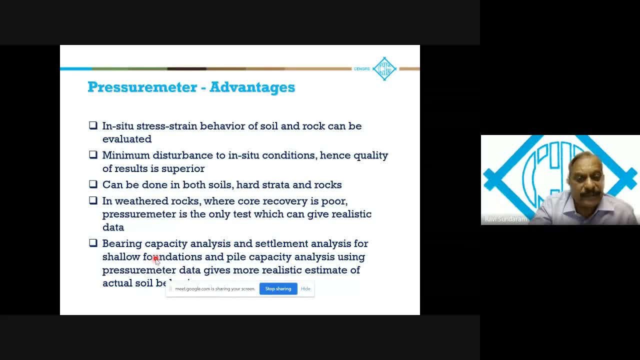 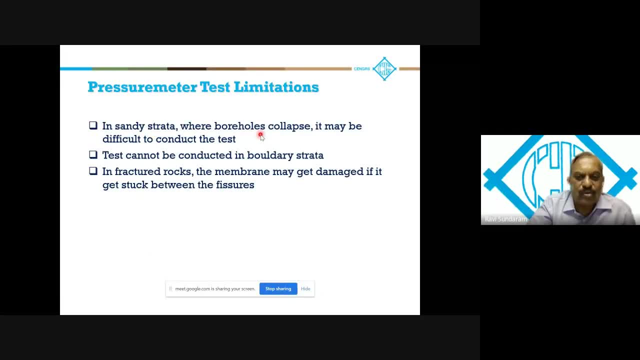 you more realistic estimate of the actual soil behavior. of course every test has its limitations. in sandy strata where the boreholes collapse, it may be difficult to conduct the test again. in boulders you cannot do it in fractured rocks. the membrane may get damaged if it gets stuck between 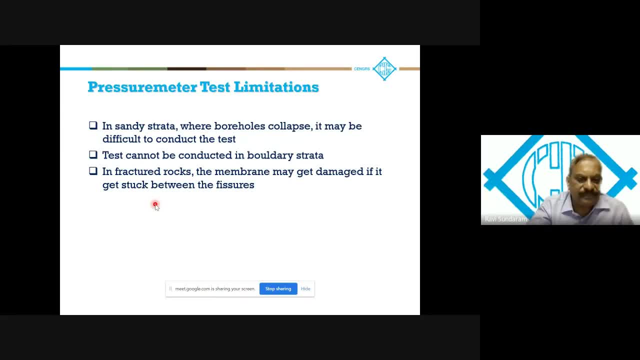 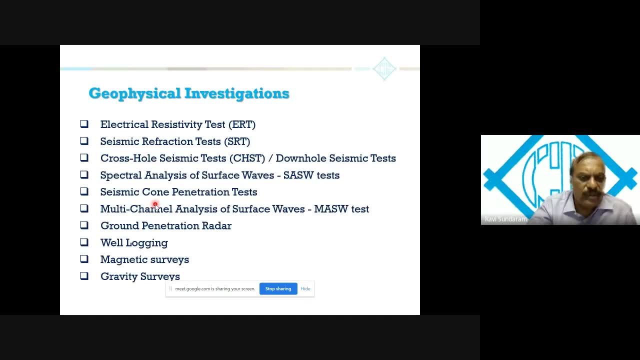 the fissures. so these are some of the limitations of this test. I move on to geophysical tests. So there are various geophysical tests which are available: Electrical resistivity, seismic refraction, cross hole seismic test, SASW, seismic cone penetration test, MASW test, ground penetrating radar. 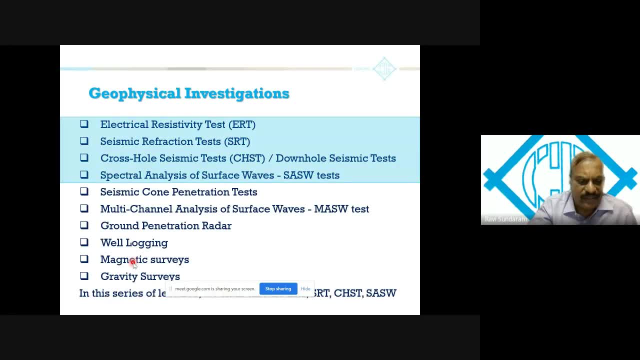 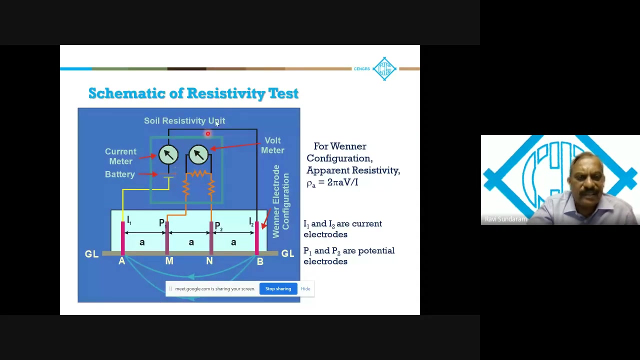 cell logging, magnetic surveys, gravity surveys, etc. In this series of lecture we will be talking only about the first four: resistivity, seismic refraction, cross hole and SASW. So I start with electrical resistivity test and introduction. So this is the schematic of 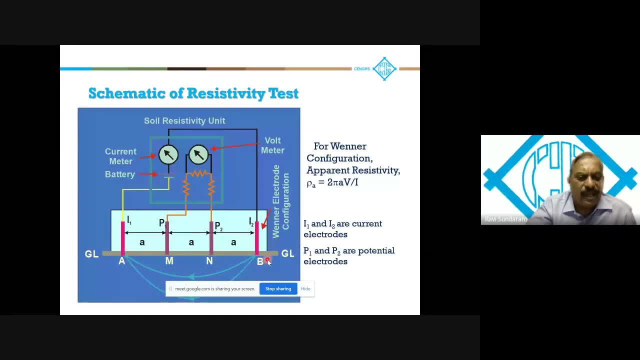 the resistivity test. You have four electrodes, usually Okay- Embedded in the ground. The inner one are the potential electrodes and the outer ones are the current electrodes. And for the Wenner configuration you have an equal spacing of the electrodes, So the depth of penetration of the current is usually equal to the electrode. 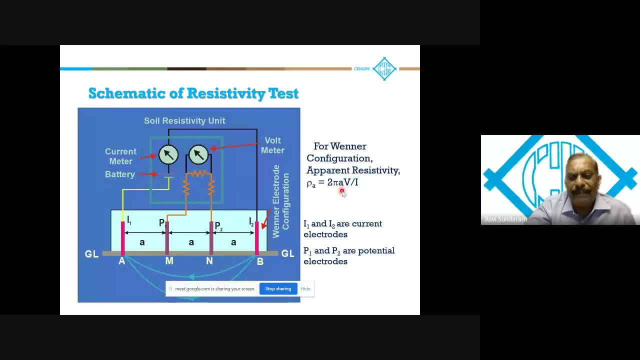 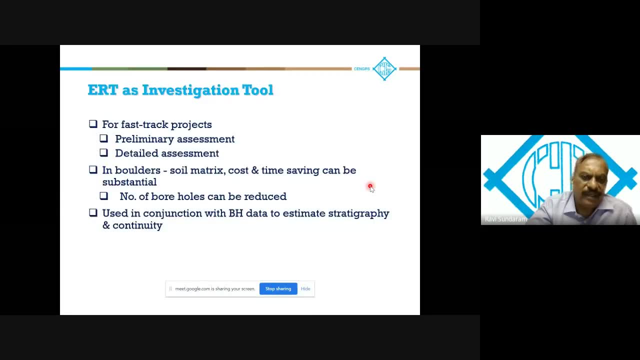 spacing So you can calculate your apparent resistivity by this correlation. What is susceptible, which is basically purely relative, is involved. Yeah, Let's see where is this correlation here. It can be used as an investigation tool for fast track projects, preliminary assessment as well as detailed assessment in boulder. 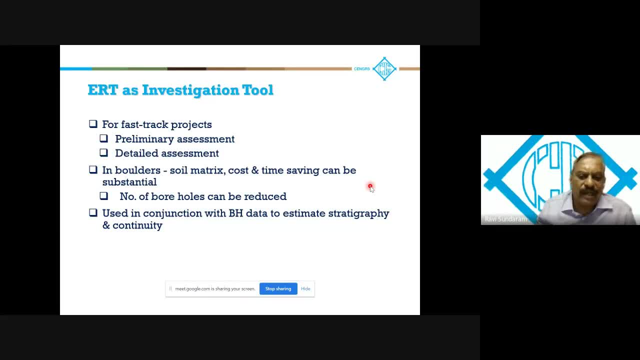 soil metrics, cost and time savings can be substantial. Number of boreholes can be reduced. Using conjunction with borehole data, It can be used to estimate the stratigraphy and for confirming the continuity of the strata. Okay Okay, Electrical resistivity, of course, is governed by Ohm's law. 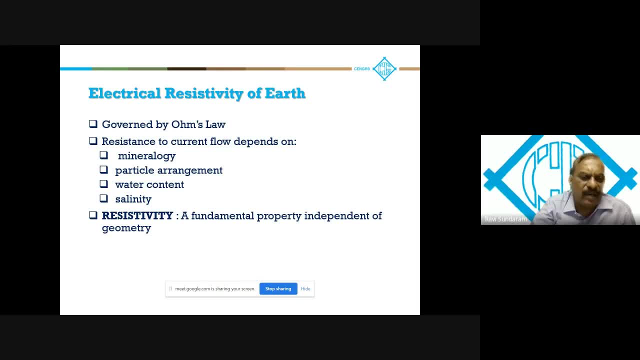 The resistance to current flow depends on mineralogy, particle arrangement, water content, salinity, etc. Resistivity, of course, is a fundamental property of the soil. It is independent of geometry. We'll discuss this in more detail in the presentation two weeks later. 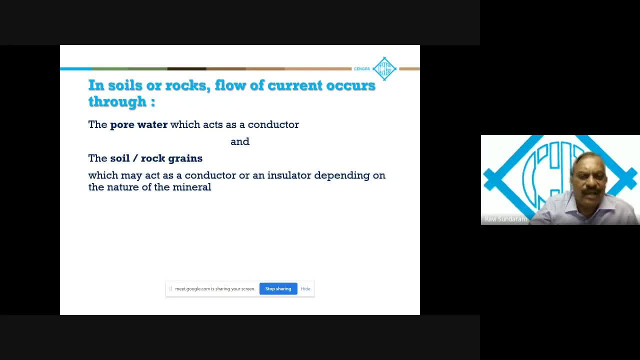 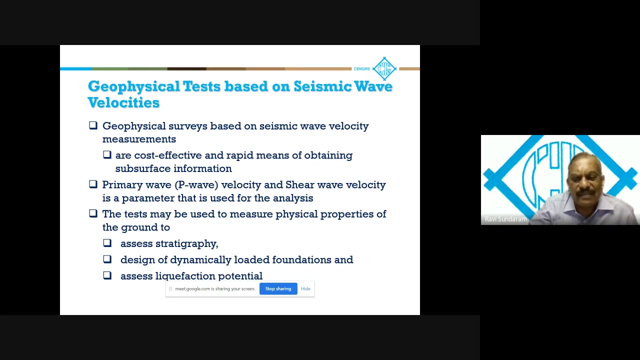 The current actually flows through the pore, water, which acts as a conductor, as well as the soil and rock grains, which may act as a conductor or an insulator, depending on the nature of the mineral. I move on to seismic tests for wave velocity: geophysical tests based on seismic wave velocities. 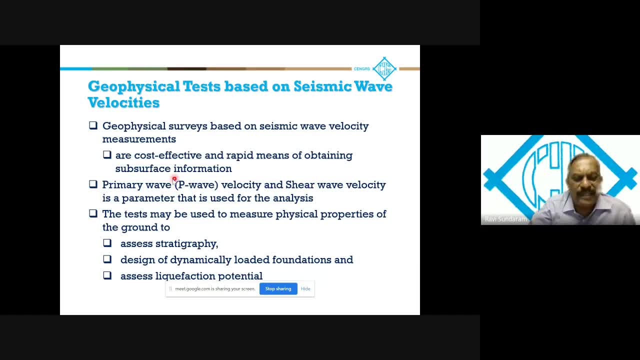 So these are cost effective And rapid means of obtaining subsurface investigation. The primary wave velocity and shear wave velocity is a parameter that is used for the analysis. The test may be used to measure the physical properties of the ground, to assess the stratigraphy. 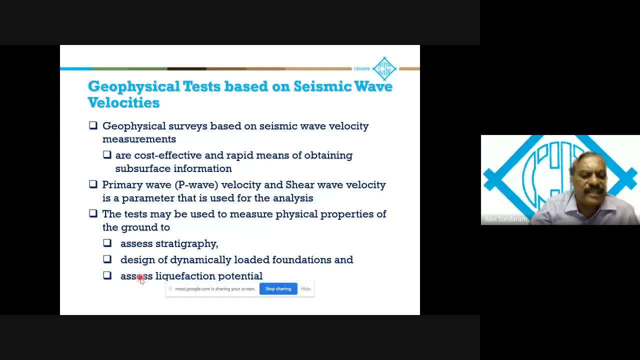 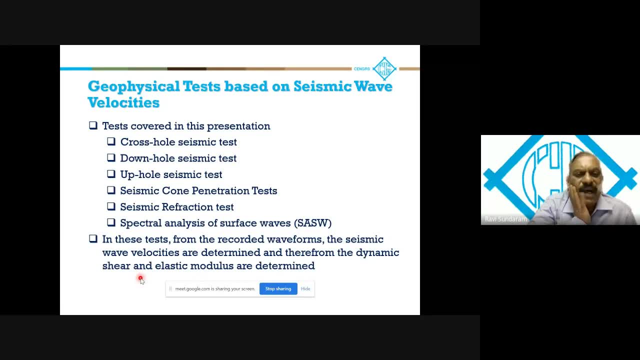 design of dynamically loaded foundations and to assess the liquefaction potential. So the test covered in this presentation here I'll just be briefly talking about the cross-hole seismic test, The downhole seismic test, the uphole seismic test, seismic cone penetration test, seismic. 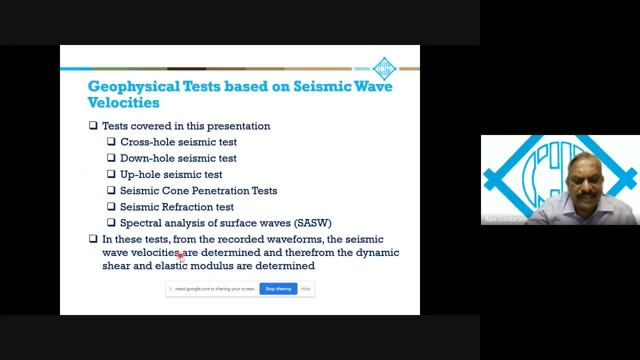 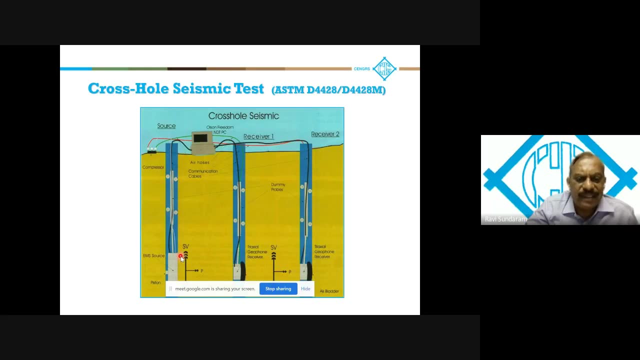 refraction test and SASW test. In these tests the recorded waveforms, the seismic wave velocities, et cetera are determined, And from there we'll determine the various parameters. So start with cross-hole seismic test. So here you have three boreholes. 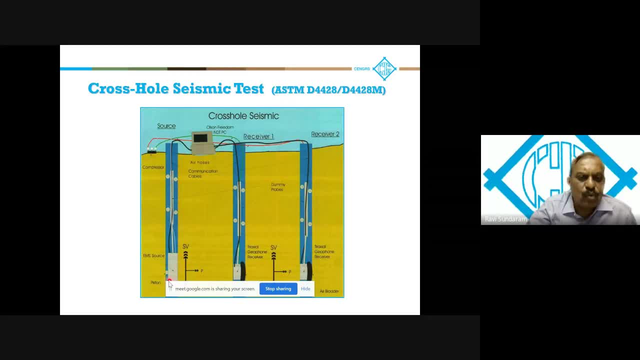 This one. this borehole would act as the source where you create an energy impact, And you have the parallel boreholes, normally three to four meters apart, And here you have geophones at this level, at the same level as the, where the impact 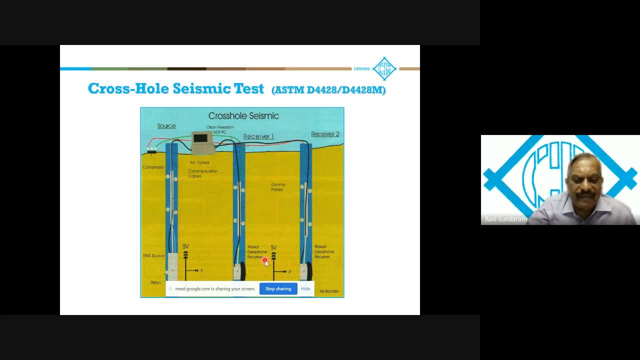 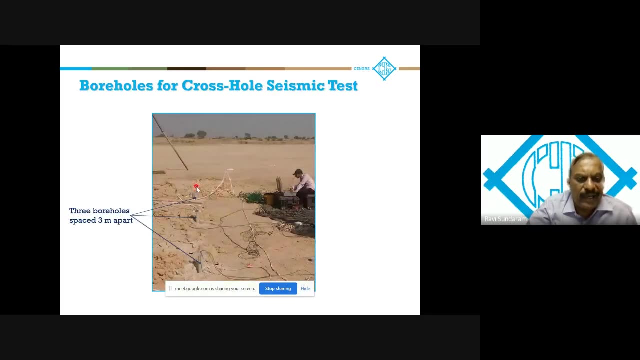 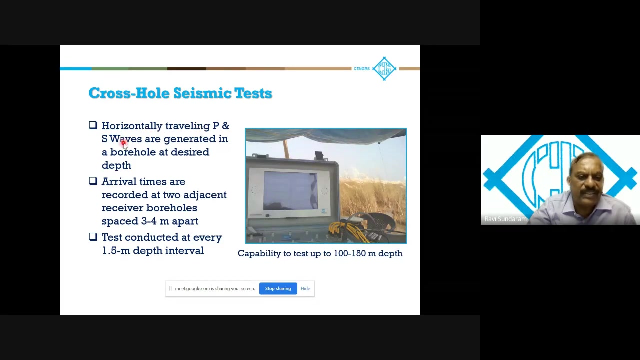 is being generated And what you would do is you would measure the record, the time, So you would measure the time of arrival of the wave at these two locations. So we have three boreholes here and the data acquisition being done. So here cross horizontally traveling P and S waves are generated in the borehole at the 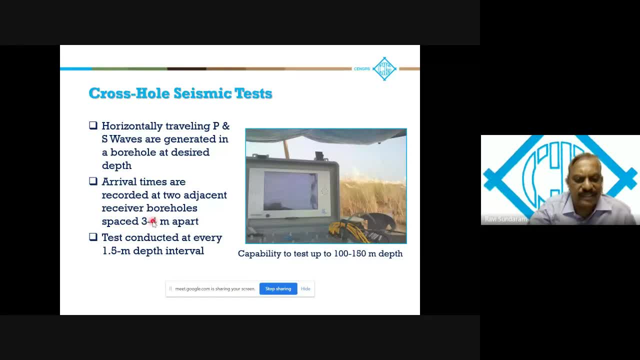 desired depth. Arrival times are recorded at two adjacent boreholes And the data acquisition is being done. So here cross horizontally traveling P and S waves are generated in the borehole at the desired depth And you wie the test is conducted. usually the test is conducted at every 1.5 meter depth. 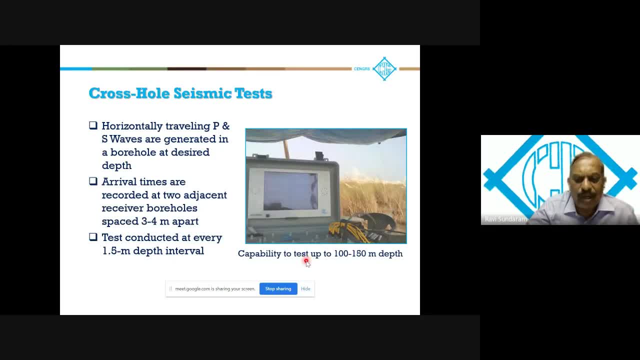 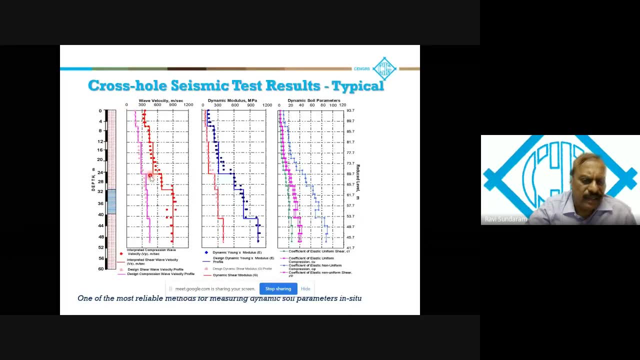 interval. You can use the system to test up to a hundred hundred 250 meter depth Typical results. So this is the primary wave when the sorry. this is the chain velocity for the primary wave And this is the velocity of the shear wave. 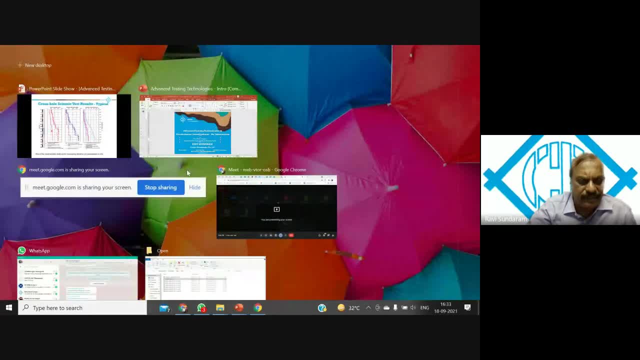 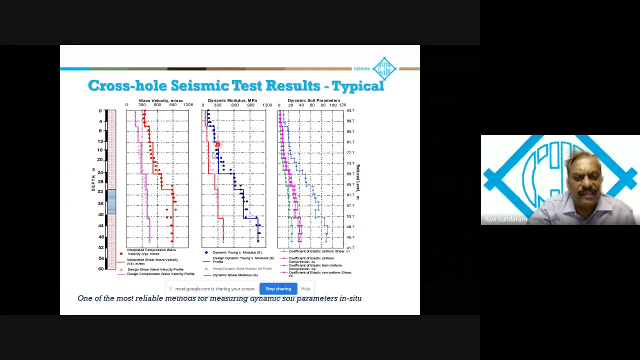 So you can see how it is increasing with depth. So back here, here is a wave And this the depth of the beam, The density, the order of descent. So dynamic modulus, including the dynamic Young's modulus and the dynamic shear modulus. 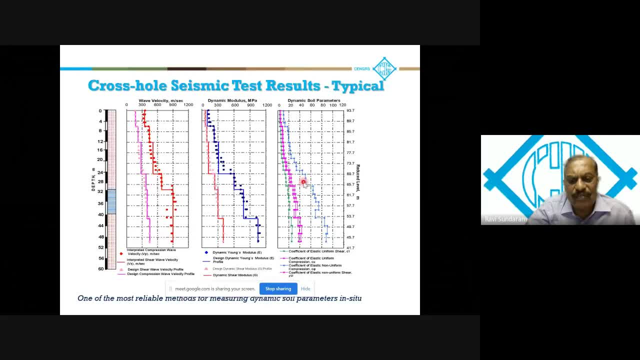 can be determined. There are various other parameters, like coefficient of elastic uniform shear, coefficient of uniform compression, non-uniform compression as well as non-uniform shear. All these parameters can be determined. It's one of the most reliable methods of measuring dynamic properties of the soil in situ. 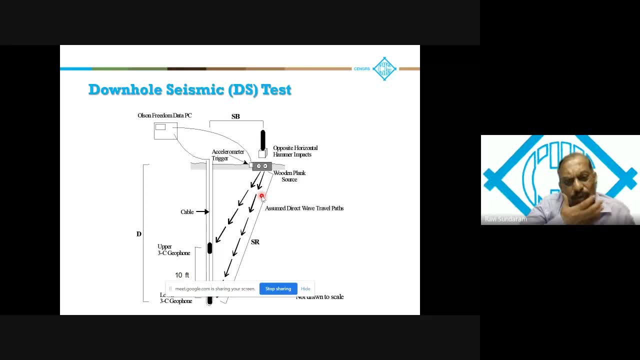 The downhole seismic test is a small variation. here You need only one borehole and the impact is created on the ground, and usually you would have two geophones suspended at two different distances and from the arrival times you can calculate the hypotenuse distance and then the vertical, of course, the wave velocity. 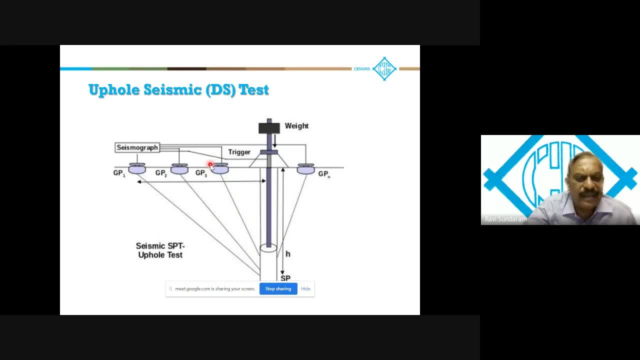 The uphole seismic test is a test in which you create the impact down here and you have geophones placed along a line and normally impact is created. So the impact is created on the borehole and you can do the uphole seismic test. 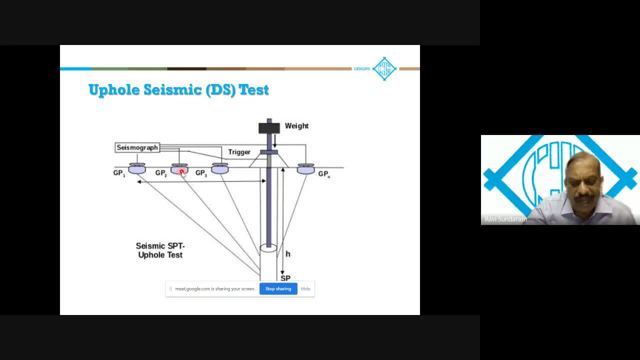 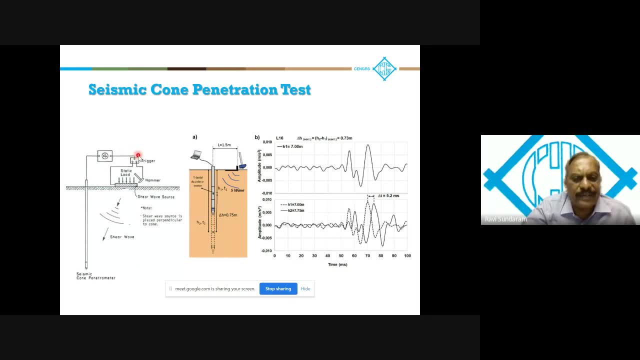 This would be similar, slightly different from the downhole. The seismic cone penetration test uses the same cone penetration test. The cone has a sensor by which you can measure the wave velocities. The impact is again created at the ground surface. then you would measure the response. now i move on to seismic refraction test. 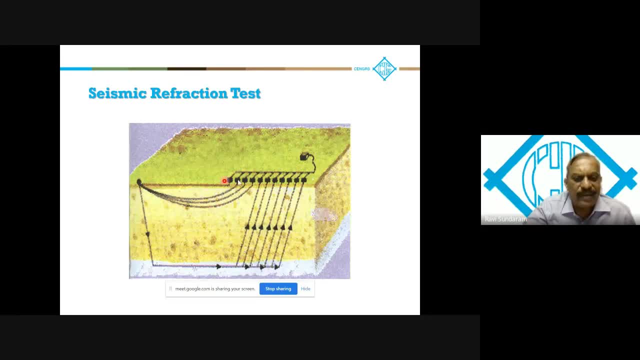 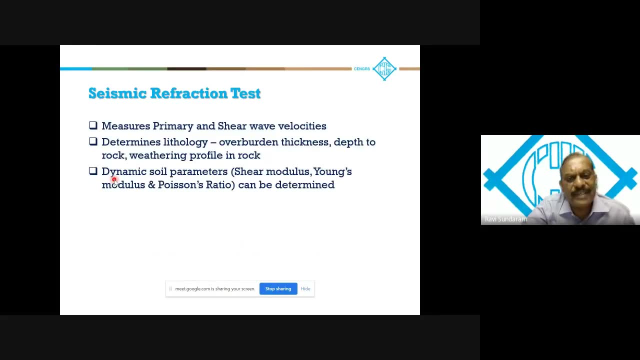 here impact is generated at one point and you have a series of geophones along a line. so it measures the primary and shear wave velocities. it determines the lithology, the overburden thickness, depth to rock and weathering profile of the rock. dynamic parameters in the shear modulus, young's modulus and poisson ratio can be determined. 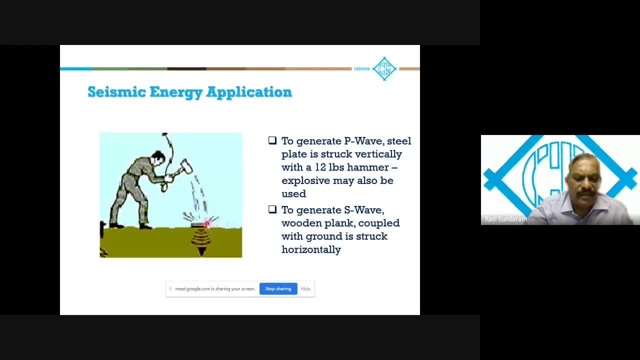 so here you would generate the p wave. you strike a plate on the ground with usually a 12 pound hammer. an explosive can also be used if you want to get the energy down to greater depths. to generate shear wave, a wooden plank can be used. coupled with the ground is struck horizontally. 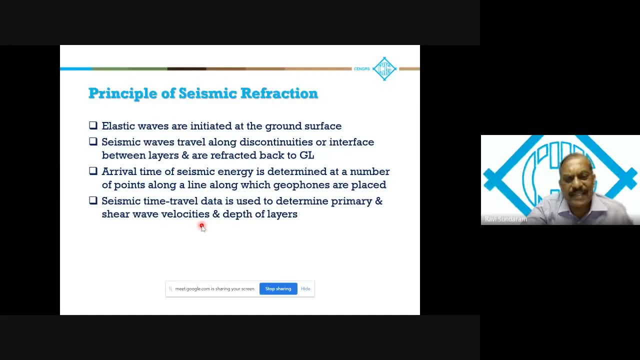 so the principle is that elastic waves are initiated at the ground surface and the seismic waves travel along the discontinuities or the interface, and then they are uh, reflected, refracted, back to the ground level. the arrival time of the seismic energy is determined in a number of points along the line, along with the geophones. geophones are placed and 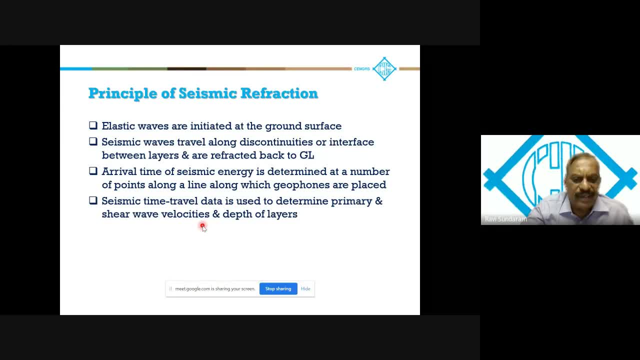 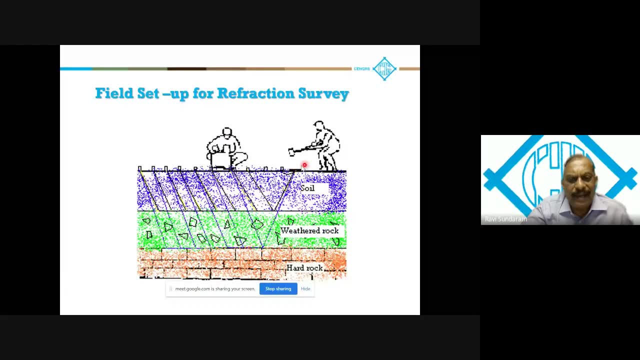 the travel time data is used to determine the primary wave and the shear waves and the depth of the layers. so this is the field setup where you have an impact and then you measure at the various geophones so the impact gets refracted along this and you get the refracted wave. 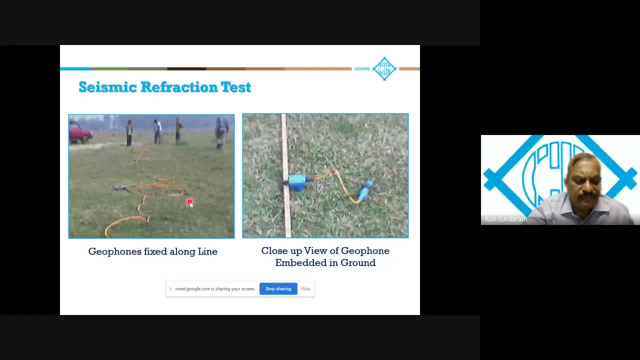 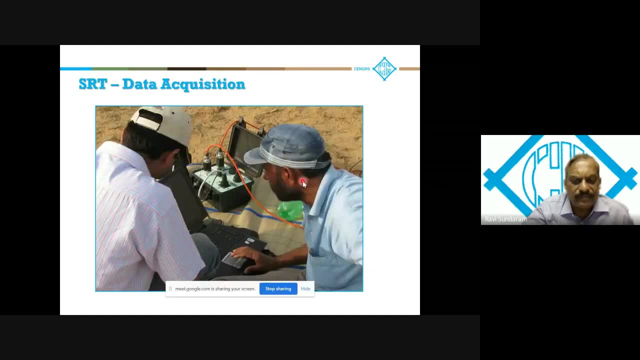 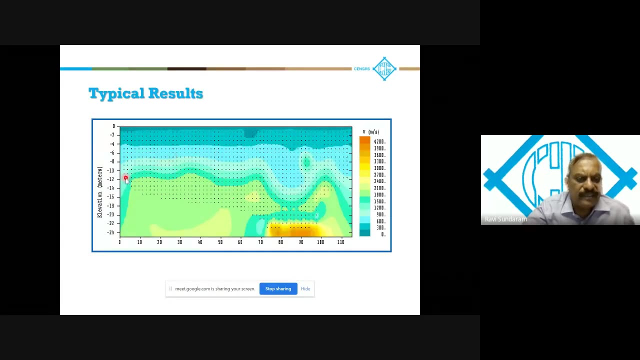 so you can see here how the uh любим. you can see the direction of the shock and the服 can see the geophone fixed along the line and a close-up of the geophone data acquisition being done here, the typical results. you can see the different layers. 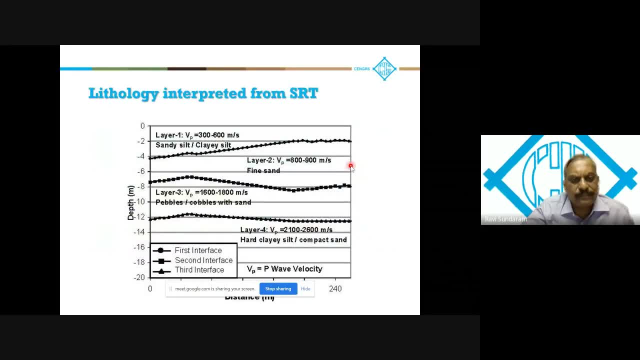 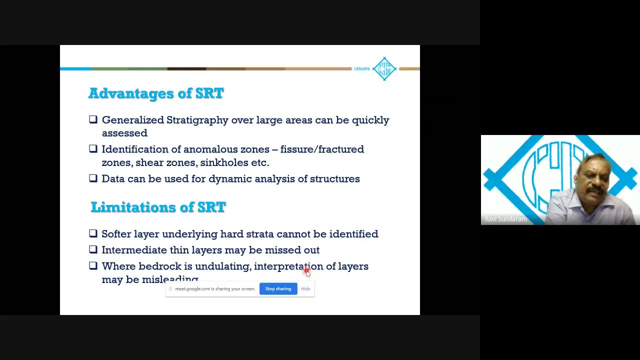 how they are. very so you can interpret the lithology from the test. so the various layers can be interpreted along the line you know. so the advantages is that generalized stratigraphy over large areas can be quickly assessed. identification of anonymous zones, fissured and fractured zones, shear zones, sinkholes- all these you can identify. data can be used for dynamic. 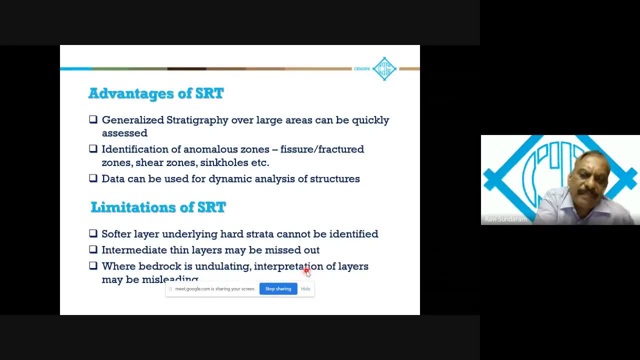 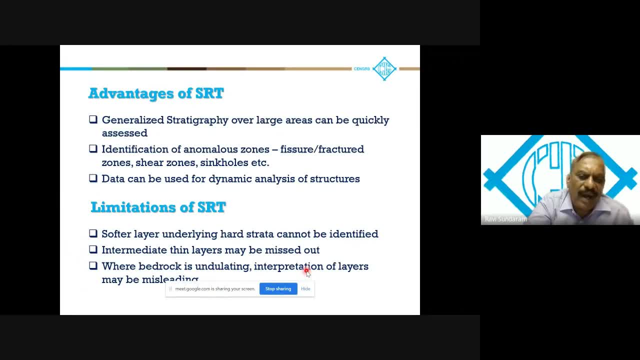 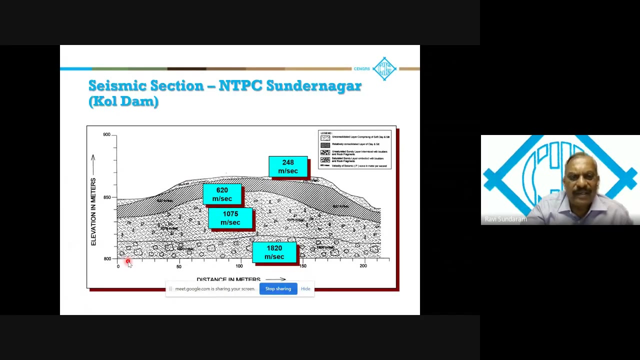 of course are there. the softer layer underlying a hard strata cannot be identified. intermediate thin layers can be missed out. the bedrock is undulating interpretation of the layers can be misleading. typical interpretation based on the a seismic refraction test. you can see here at NDPC Sundar Nagar we had 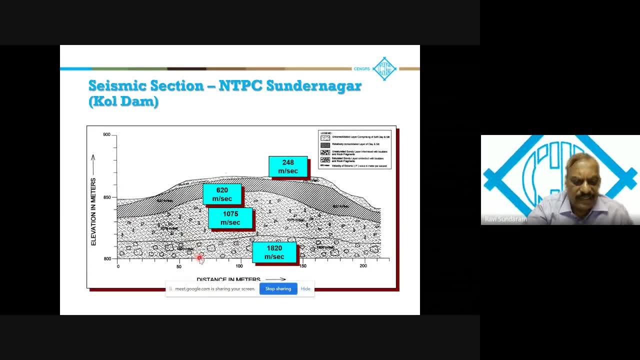 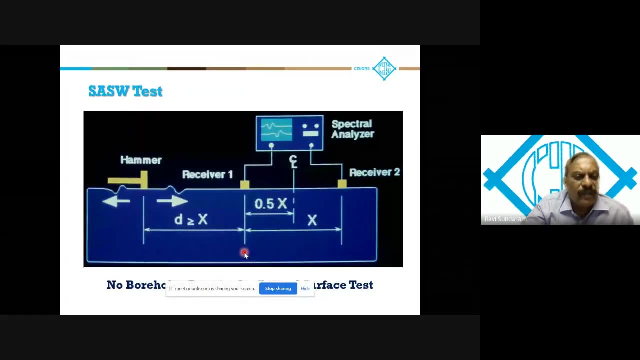 identified the various layers and the velocity of the layers and each of these layers. we could interpret from the borehole data that the deeper one is the saturated rock. I move on to SASW test. this again is similar to seismic refraction. of course, geo phones are slightly different, which are used here. so again, no borehole dough. 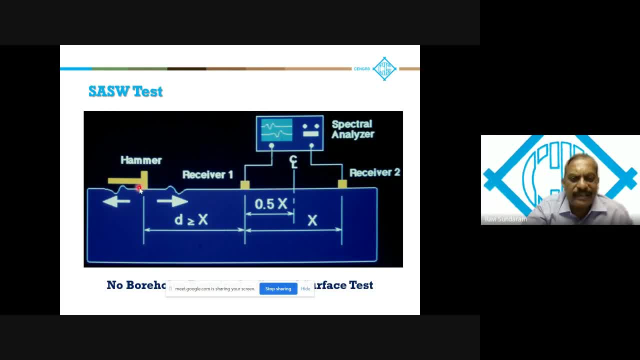 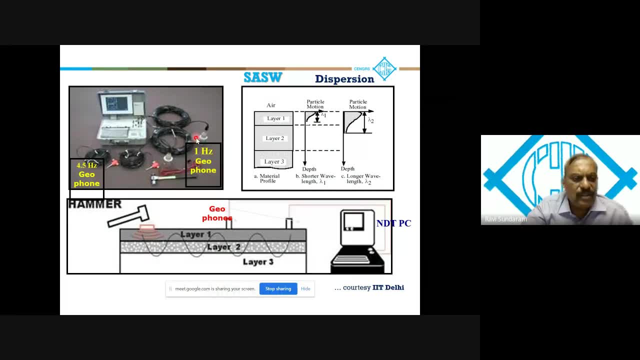 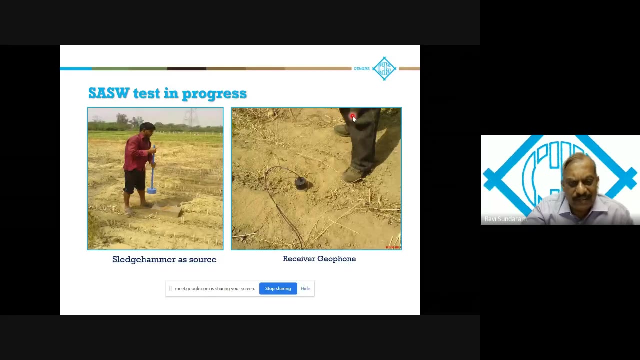 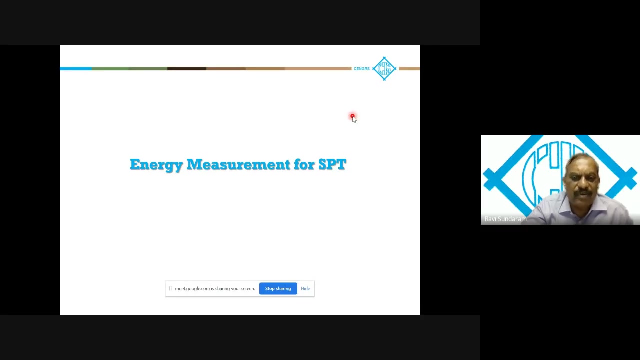 quiet here, so you have an impact, and then an array of geo phones. so this is The System Which is Used to Determine the As Asw tofu morose on coach force and steel block 1918 paper: jis asw agile Nicholas e c Cup steel as a source, so you can see the geophones here. now I come to energy measurement. 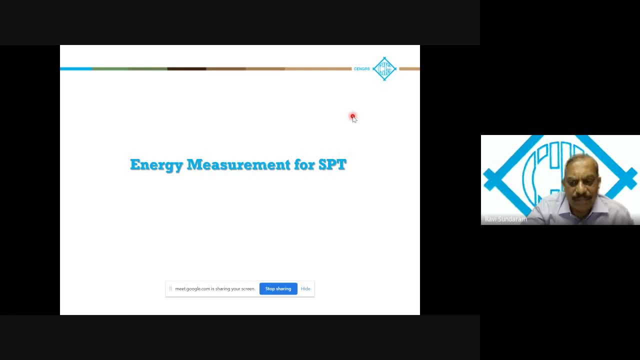 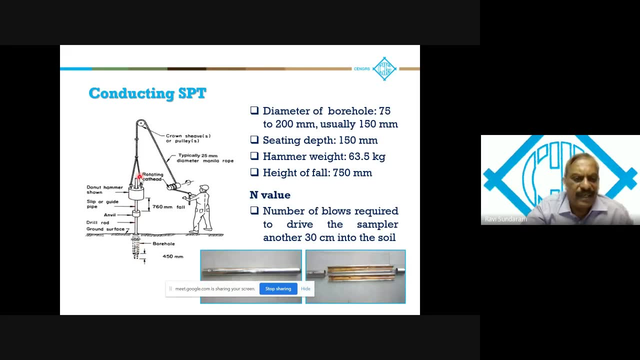 for SPT. this is the last section of my presentation here. all of you are aware of the conventional SPT system where you have a split spoon sampler and you hit with a. not normally you have a 75 to 200 mm diameter, usually 150 mm diameter. 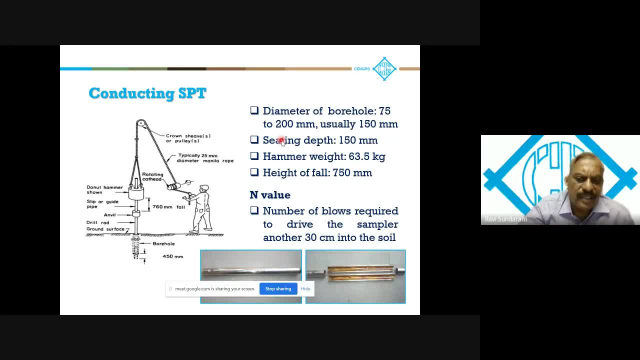 holes. so this split spoon sampler, 50 mm diameter, the hammer weight is 63.5 kg and the height of fall is 750 mm. so you drive it by first 150 mm, so those blows are ignored, and then further you drive it by another 30 centimeter. record the blows every 15 centimeter and the 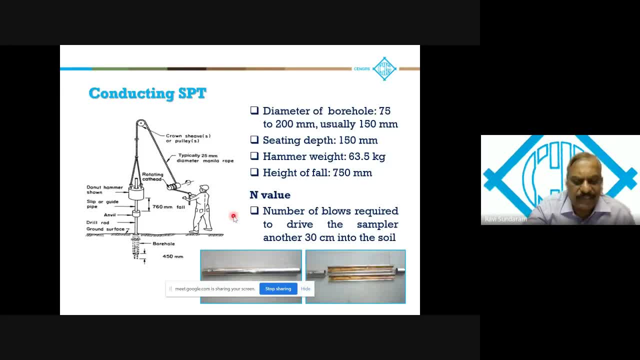 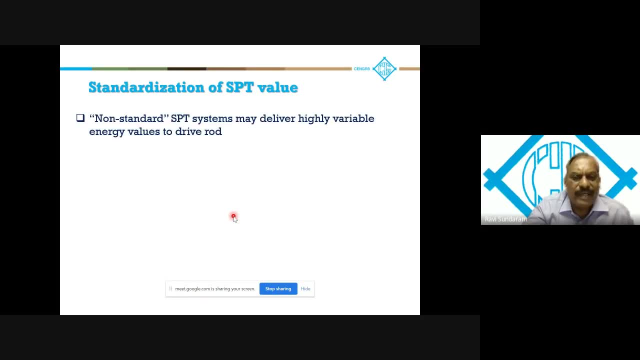 sum of the last two blows is taken as the SPT value. now standardization of the SPT value becomes very critical because non-standard SPT systems may deliver highly variable energy values to the drive rod. the energy transfer affects the n value, so the energy transfer. 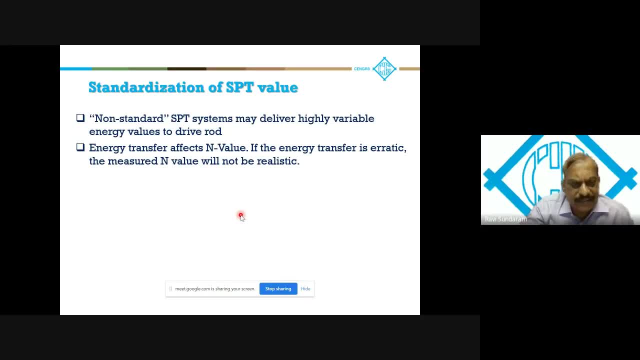 is erratic, the measured n value will not be realistic. so the soil strength, safe bearing, pressure, foundation settlement. other geotechnical parameters are usually based on the average n value. so lower energy will yield in higher end result in a high end value, leading to unsafe predictions. high energy could 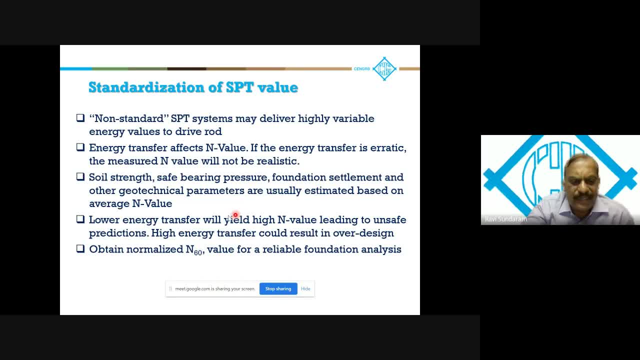 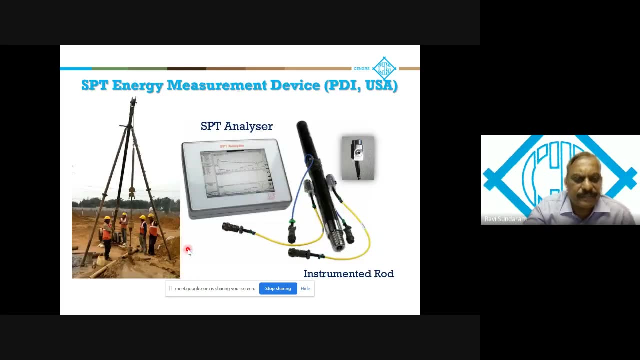 result in over design. so you must obtain a normalized n60, which is 60% efficiency, for reliable foundation analysis. a liquefaction potential also uses n6, n16, which is 60% efficiency. so the SPT analyzer is a very effective way of doing this here you. 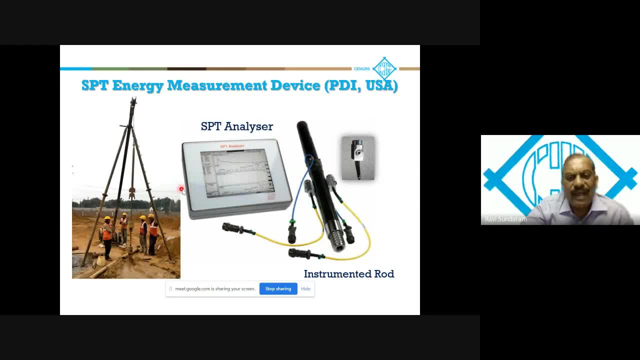 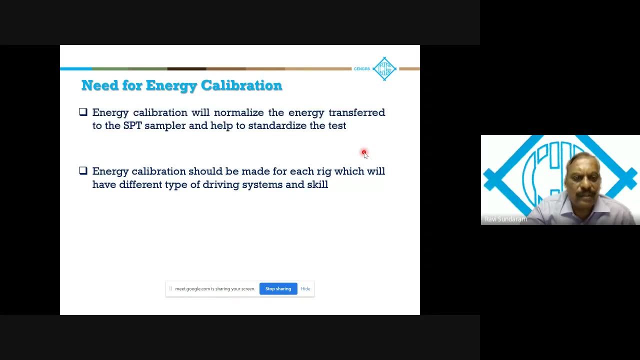 have a instrumented rod which is used at the top and this with the analyzer. you have a accelerometer and a strain gauge fixed at the top. so energy calibration will normalize the energy transfer to the SPT sampler and help standardize the test. it will remove the scatter in the values and thus enhance the reliability. 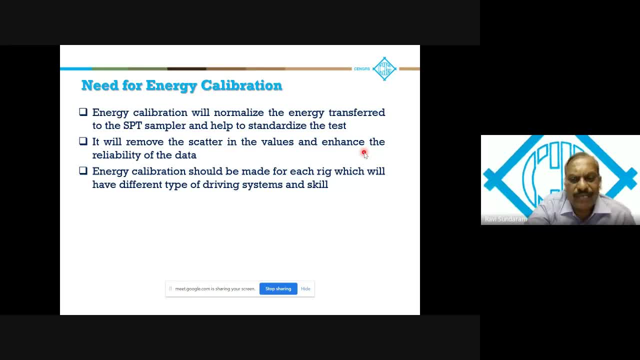 of the data. energy calibration should be made for each rig which will have different types of driving systems and skill of the operator. it should be standardized to 60% energy transfer so that all the correlations which are used with n they can still be valid. IAS 2131 and 1893 shall be similar in while addressing 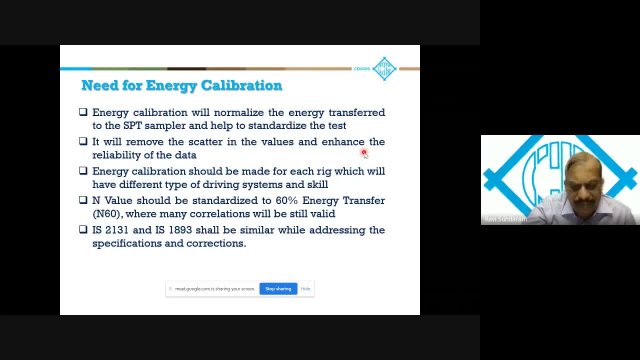 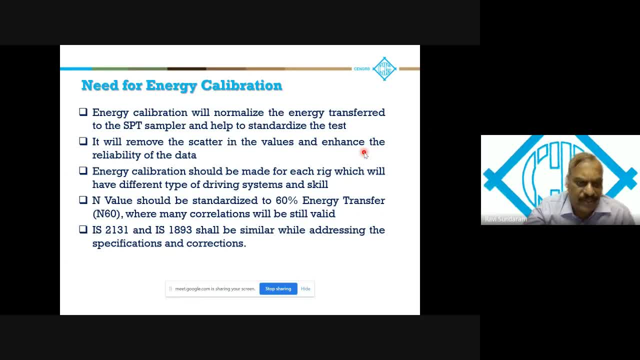 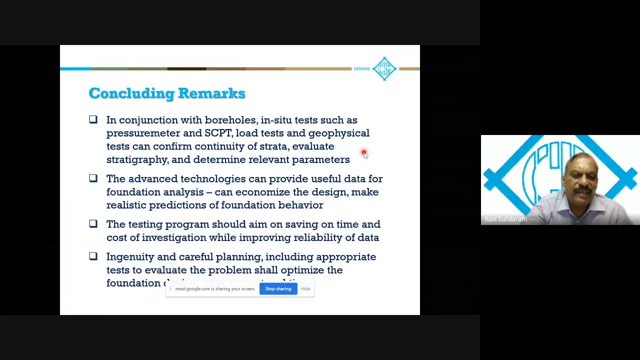 but energy calibration. but the code is under revision and hopefully this will be introduced in the code very soon. ASTM of course has a energy calibration is advised. so with this I come to the conclusion of this presentation. in conjunction with boreholes Institute tests such as pressure meter test and SP is static code penetration test, load test, etc. they 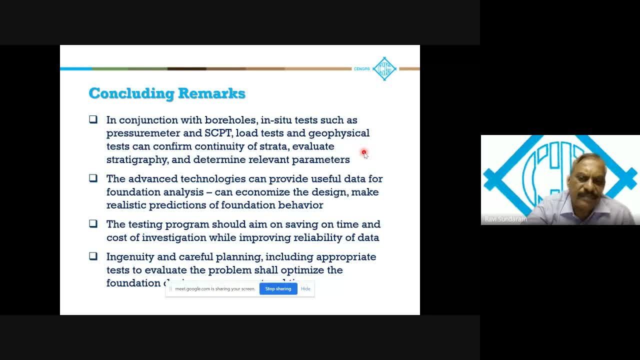 can, as well as geophysical tests. this can confirm the continuity of the strata, evaluate the stratigraphy and determine the relevant parameters. the advanced testing technologies can provide useful data for foundation analysis. it can economize the foundation design, make the predictions more realistic so that we 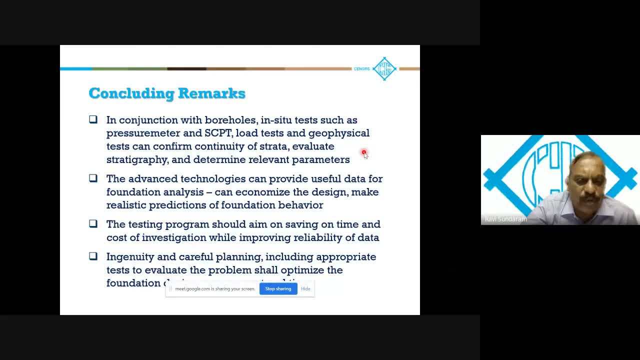 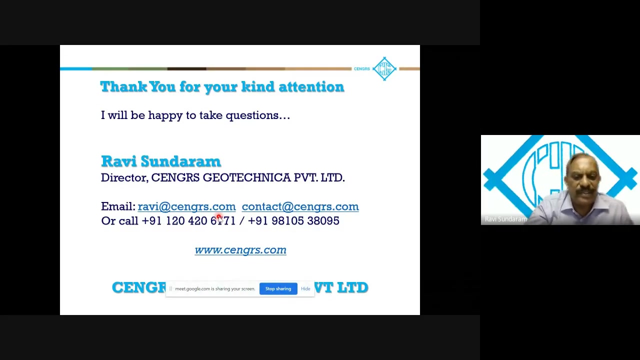 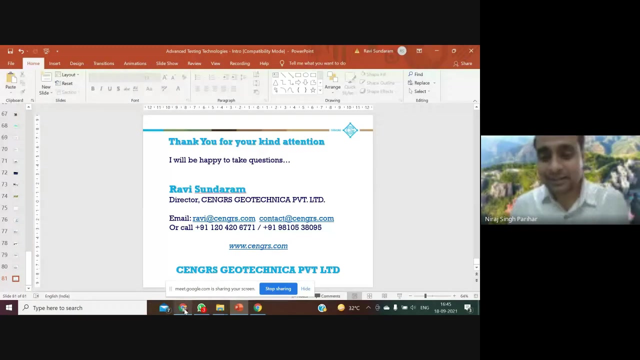 can have a better control on the foundation behavior. the testing procedure testing program should aim on saving time and cost of investigation while improving the reliability of data. it should also aim on performance, efficiency and Islam will. quipl vehicle models are applied and each technical forearm been everything. a capacitors. we cannot just fished out д? cc, car très schautz a catuara construction speedy doivent thế gi vert ces tests too, as will be talked a lot about. you talked a lot about engineering, the engineering technology, rather than nuggets, the endured, do not check the engineering part there. so as well, thank you very much for your kind attention. actually be happy to take questions, thank you as well. thank you, sir. thank you very much for the kind lecture of yours. it started from the very basics and directed to the field testing where as well we talk about Meanwhile there is talking about engineering is also connecting to different test types. so we cannot repaired element like the understanding cases. it IC, space engineering focused all depends on what you say is very difficult items has a technical needs also memorable and it were, I think, sure that the 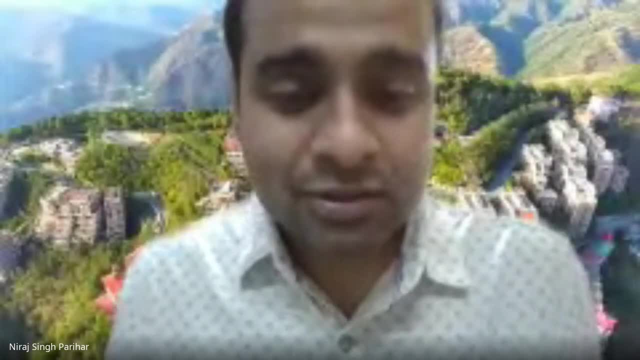 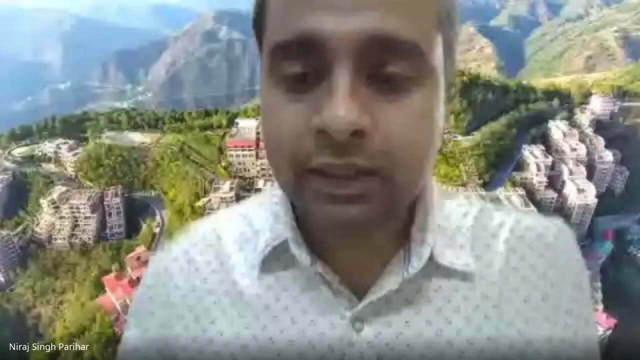 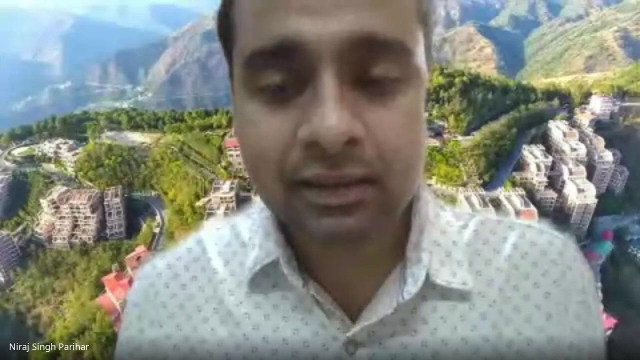 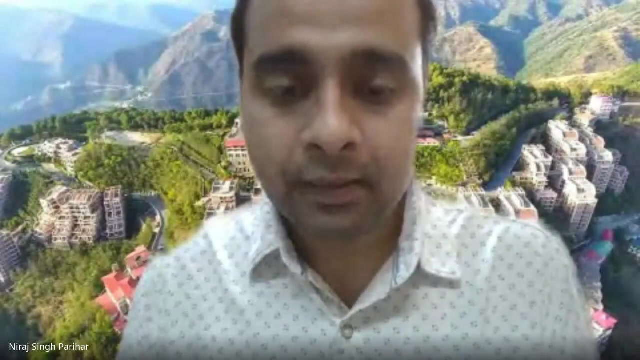 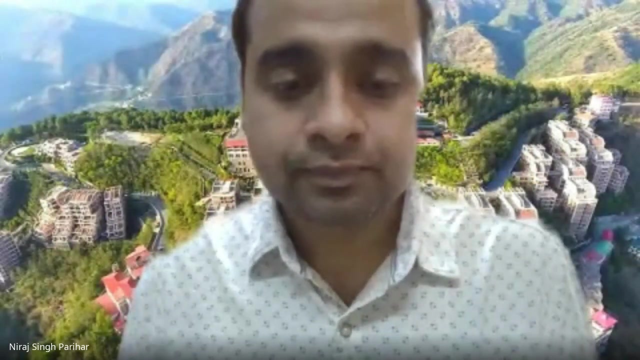 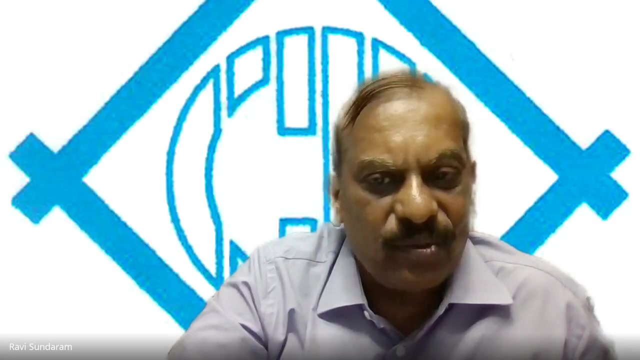 the advanced testing required in this field. so, with your kind permission, can we go on to the query round? yes, please. thank you, sir. so if any of the participants want to ask questions directly to the cell, they can unmute themselves and ask the questions. I don't know whether I went above the heads or it was too elementary. 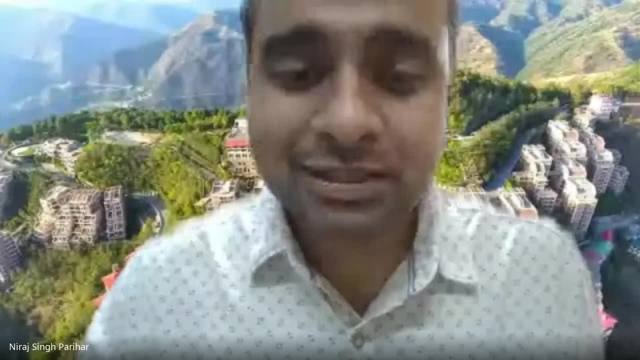 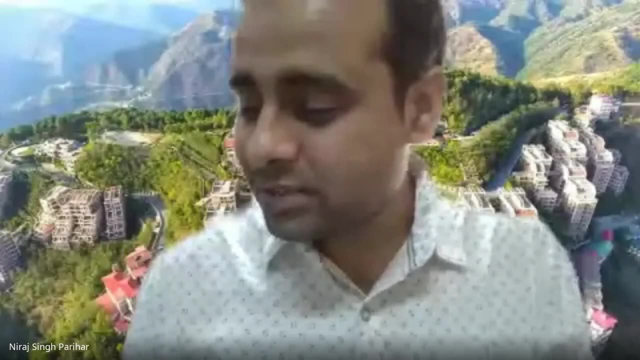 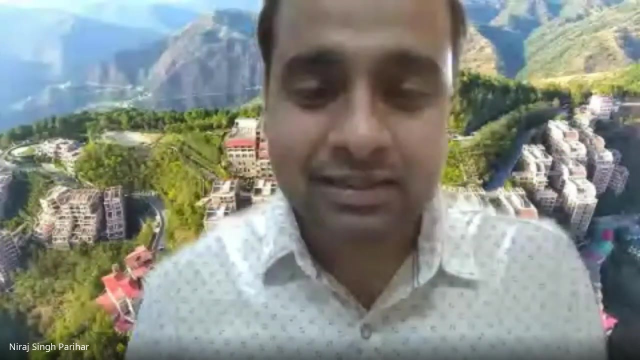 they're not in the chat box. sir, I had a few questions coming from his students with me. yes, shall I narrate them please? one of them has asked what is the difference between striking the hammer vertically or horizontally? in seismic refraction test, the vertical striking is used for the primary wave velocity and 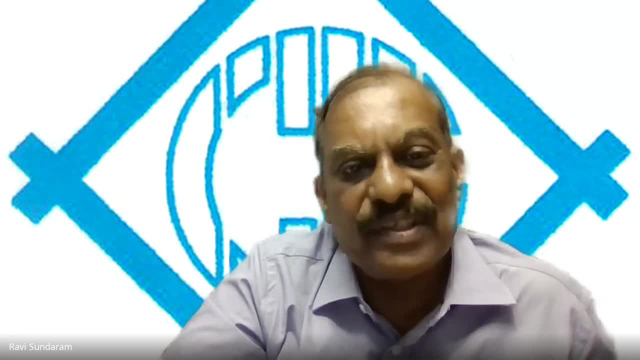 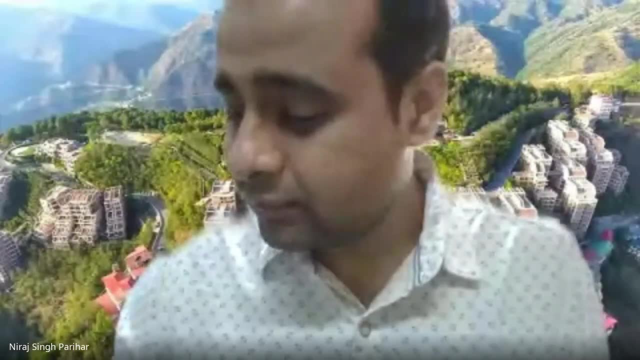 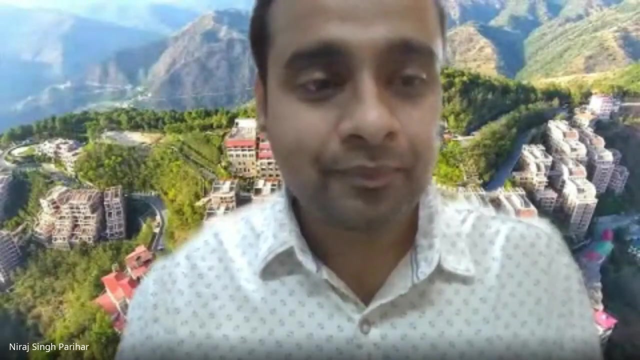 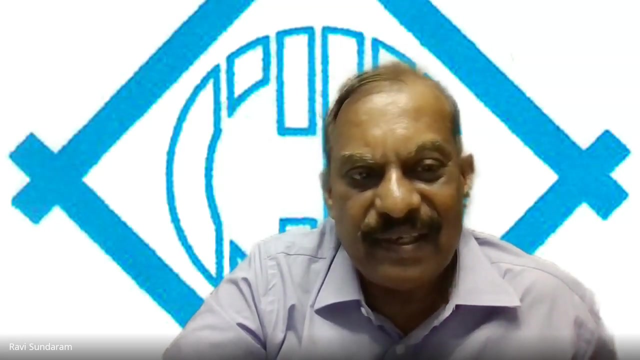 the horizontal striking is used for the shear wave velocity measurement. okay, I hope that will solve the query, sir. another question we have: can we comment on the mineralogy based on the geophysical test? well, electrical resistivity test gives you an idea of the resistivity of the ground and you 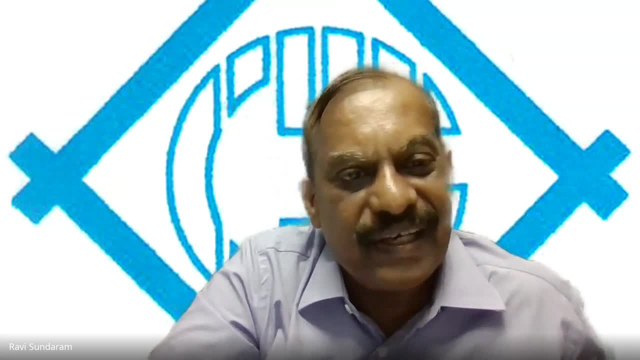 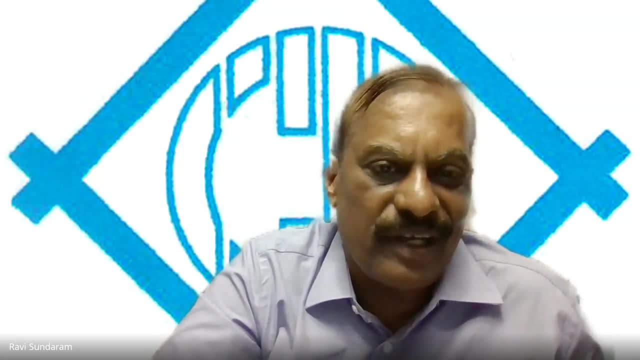 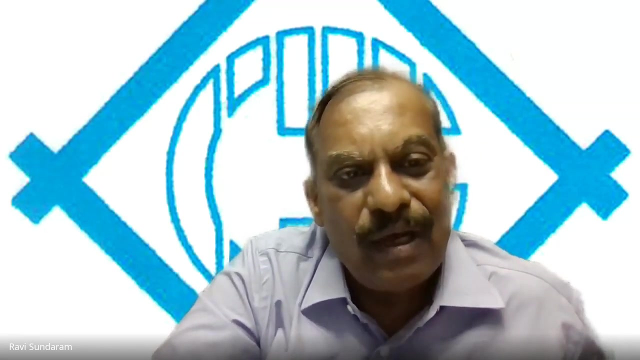 will have to compare them with the published values in literature to identify the rock type or the soil type. and then, of course, mineralogy cannot be assessed. if you can, you, you would have to know much more about the geology of the area, to know what type of rock it is, and then you know. test the material for. 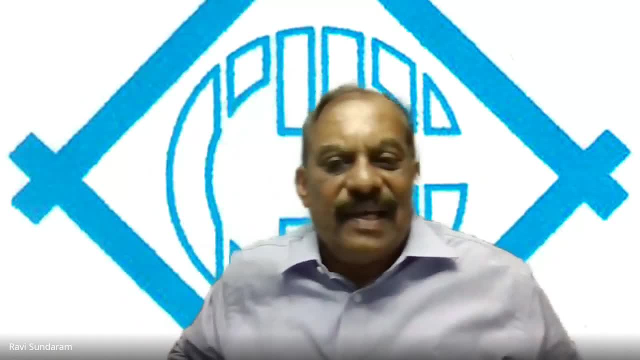 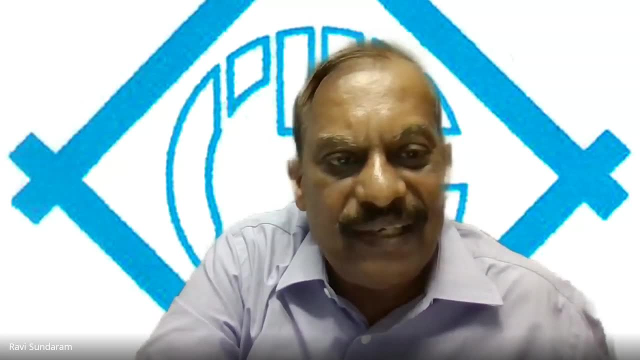 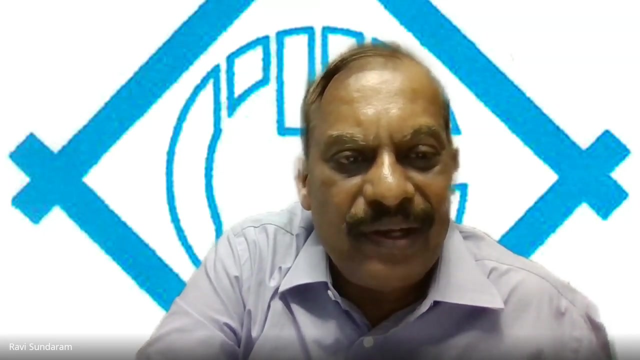 mineralogy. it can only give you a guidance as to if you are in Shimla, I know what kind of rock we should be getting there, and if you are in Delhi, I know that there would be quartzite here. so, depending on that, where I am and the kind of rock that is likely to be met you. 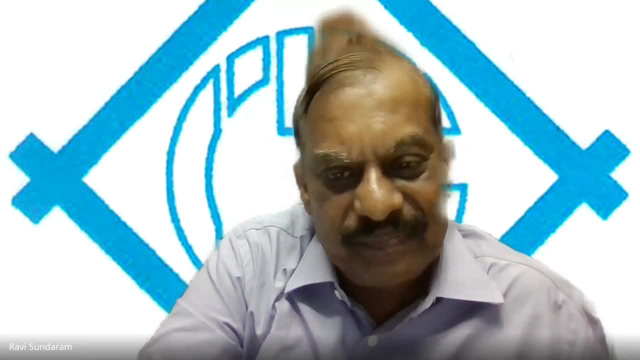 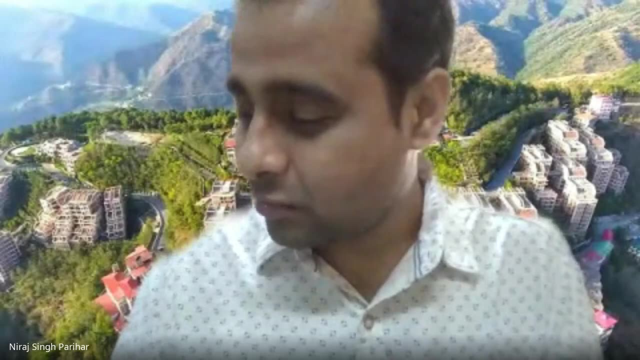 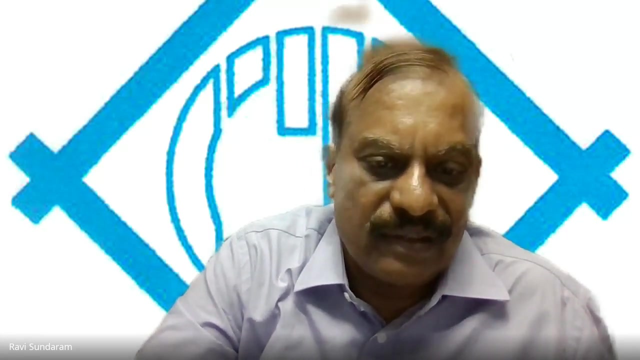 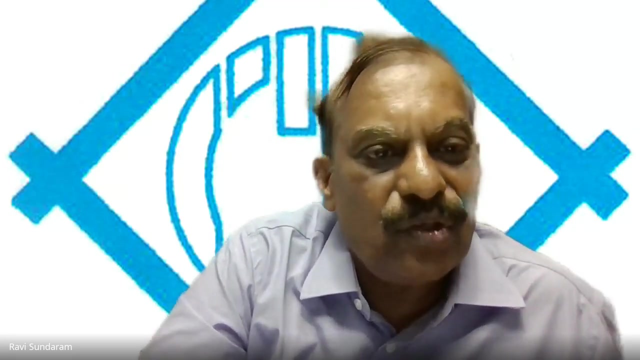 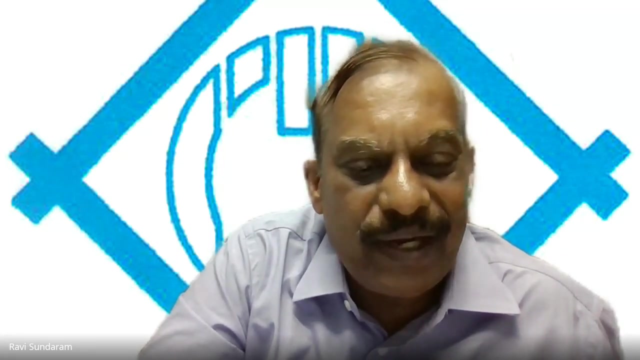 should be able to make an assessment of the mineralogy. yes, sir, there is another question again regarding the crosshole test: how the crosshole and downhole test results differ, how they differ. the downhole is a little cheaper because you know you need only one borehole and whereas crosshole requires three boreholes. so there is an additional cost of two more holes. more reliable data is from the crosshole because you get the data at the same level, Whereas in a downhole test you would get the average properties from the ground level, where the impact is made, to the level at which the bore holes are being where you are doing. 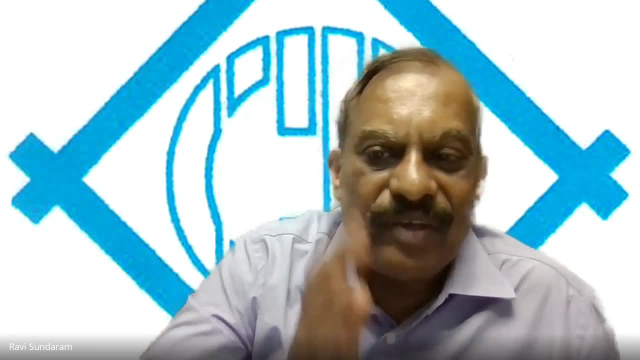 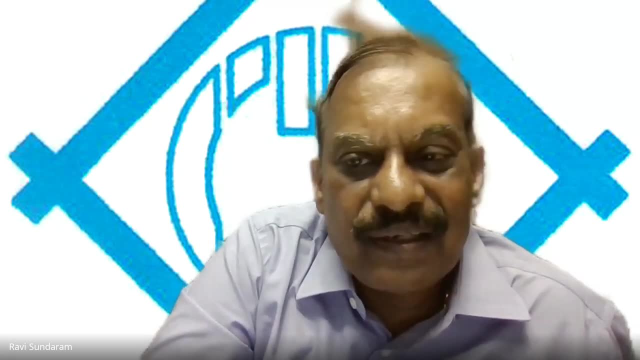 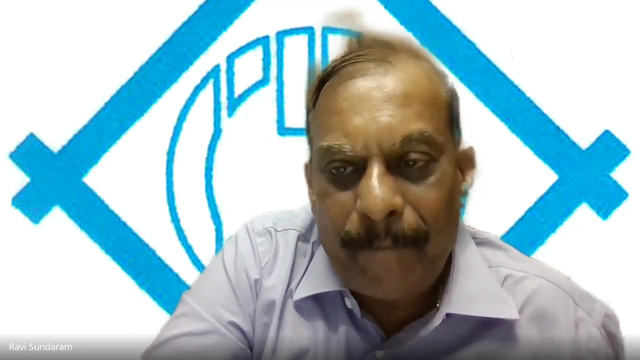 the test. So that would be an average property. So obviously it will help in getting you know the specific property at that particular level. you would have to go for crossword test, Okay, so thank you very much. So there is another question from Jitendra Raul. 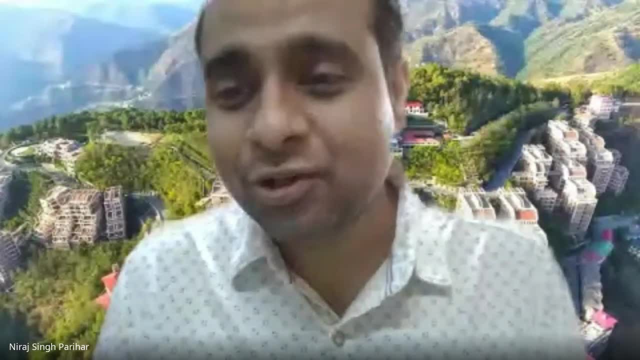 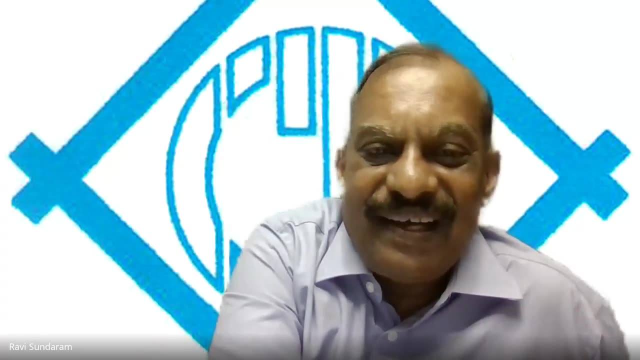 Namaskar sir, It's a very nice presentation. If presentation will contain short videos of the test, it will help us a lot. That's the suggestion, I suppose. Yes, thank you very much for the suggestion. We will include some videos, if possible, in the future presentations. 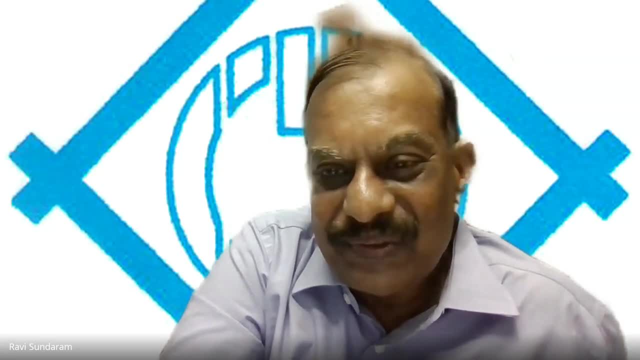 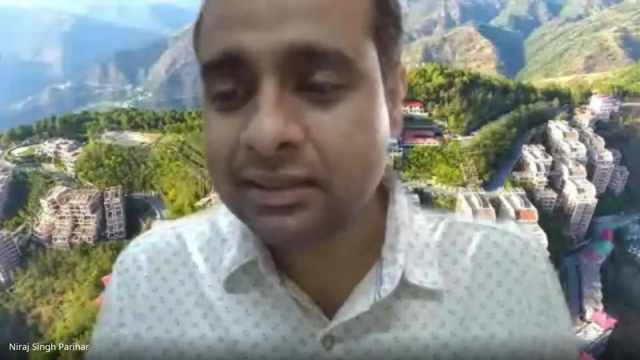 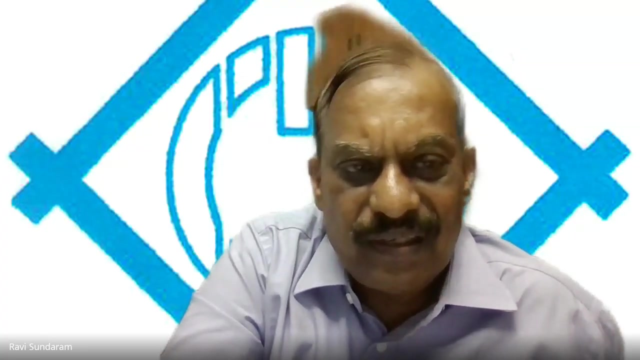 There are four more presentations due. There is another question from Kiran K. May I know the significance of VS30?? Why only at 30 meters? VS30, what is that? I think that's the shear velocity. Shear velocity is measured at all depths. 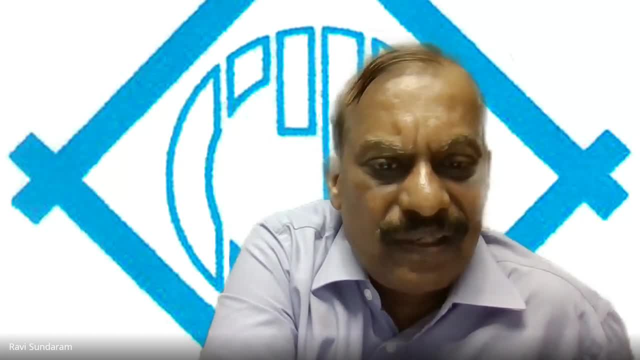 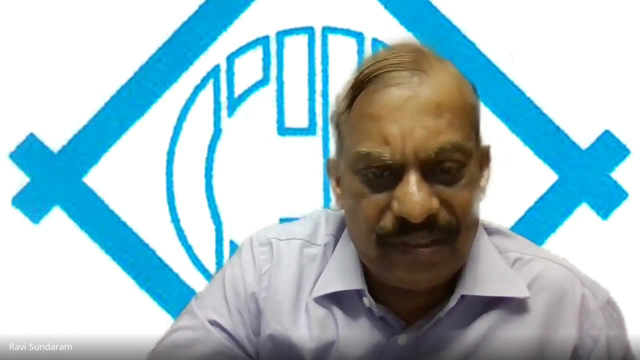 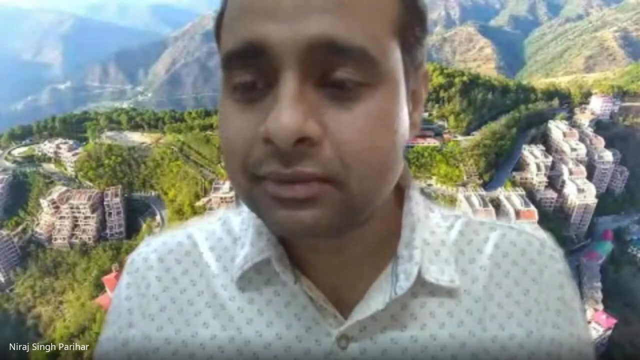 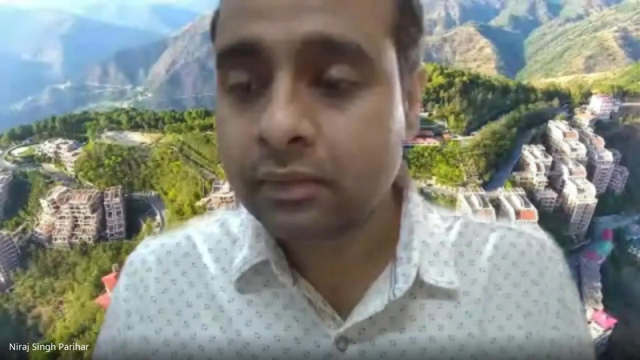 Why not? It's not only at 30 meters. I did not mention anything specific about 30 meters in my presentation. Kiran ji, are you here? Can you please further specify your question? Yes, sir, A typical case study which I had. 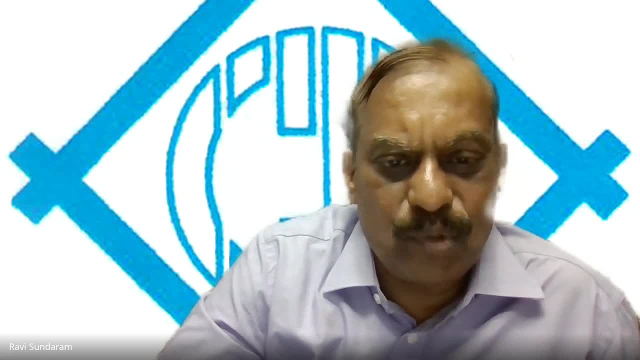 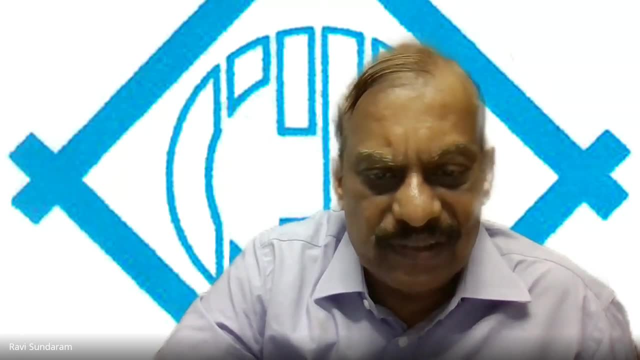 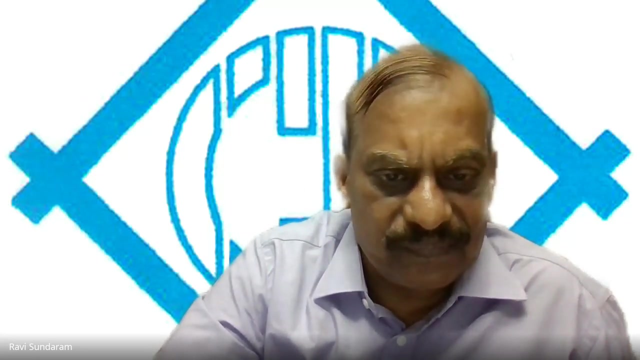 data which I had presented that was up to 30 meters, But of course you could have any kind of. it would depend on the depth at which you would do it. Yes, I think. yes, now he's satisfied. 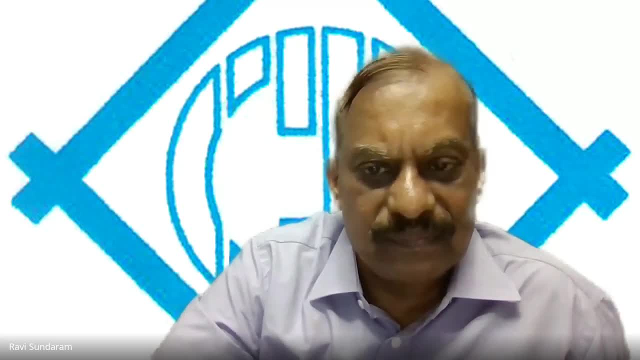 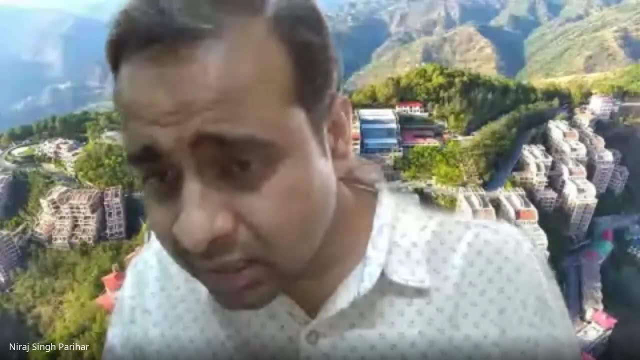 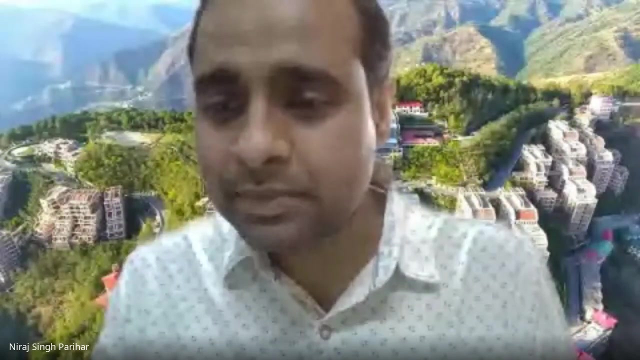 Okay, thank you. Okay, sir, I do not get any. Okay, there is another query. So this is REG pressure meter test. Yeah, It is not possible to test in sandy soils due to borehole collapse In weathered rocks. there is high chance of damage of probe. 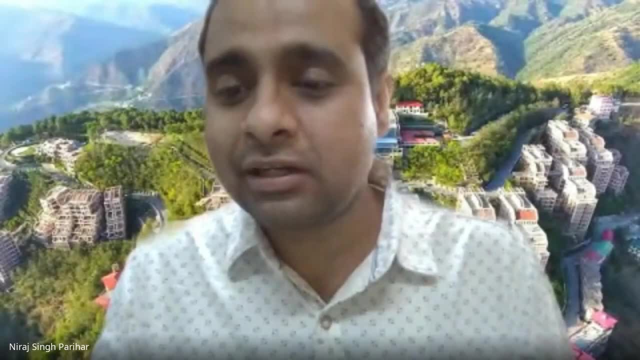 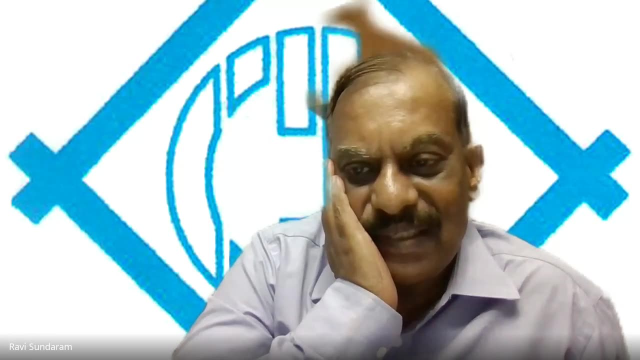 The question is: for hardy stratum like SPT and value more than 100,, what is the necessity of pressure meter test then? Okay, Now, as far as a pressure meter test in sand is concerned, it is not possible. possible is not the answer. 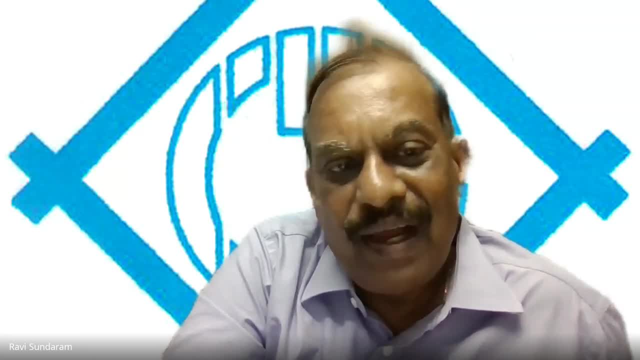 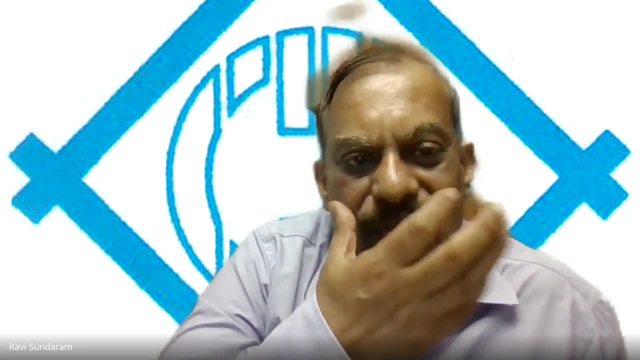 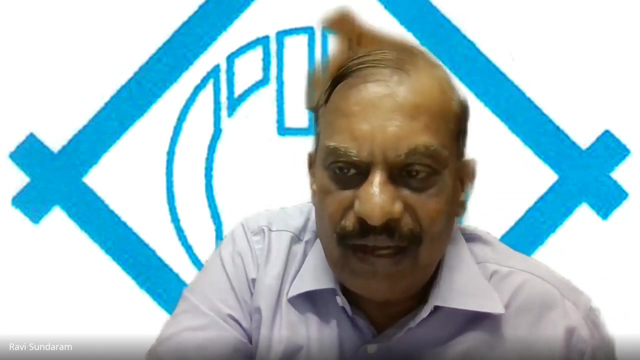 There are some limitations. We have to be very careful and it has to be very carefully done to make sure that you are able to do the test in sand. It could be challenging, Of course, in loose sands. only the boreholes will collapse. 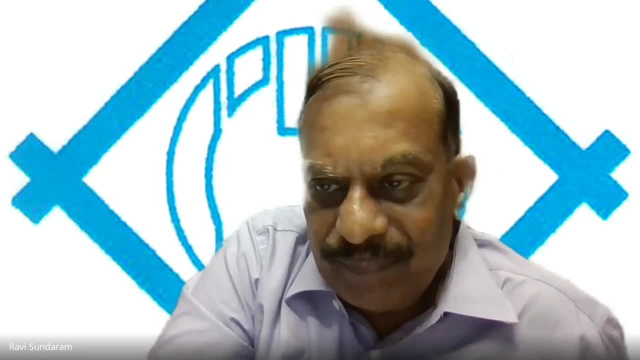 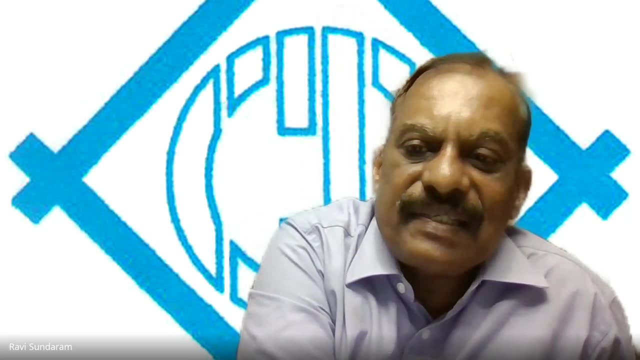 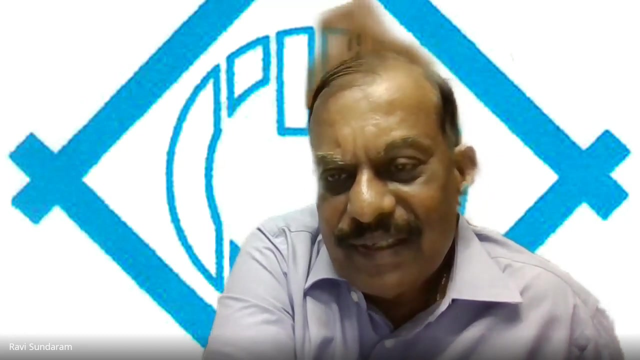 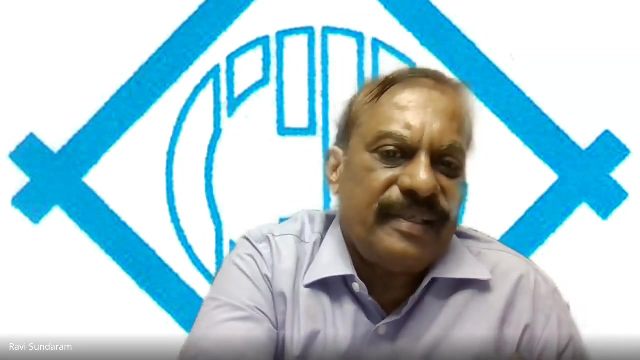 In dense sands, they may not collapse. As far as hard stratum strata, fractured rocks is concerned, you see, it depends on what your application is. Now there are some very heavily loaded facilities, particularly like you are aware of these new bridges. 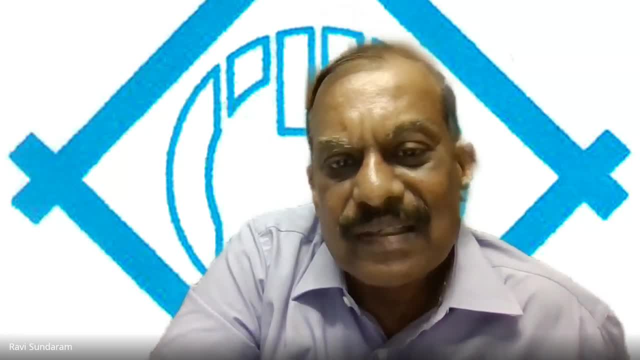 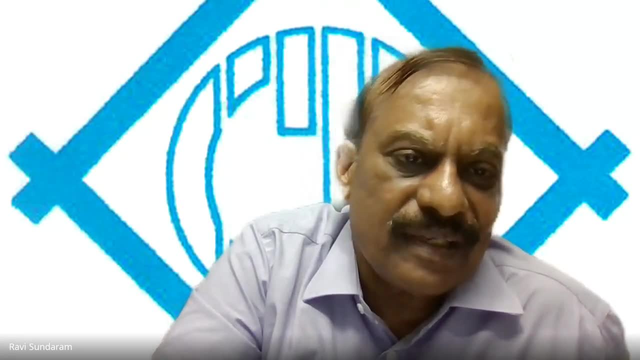 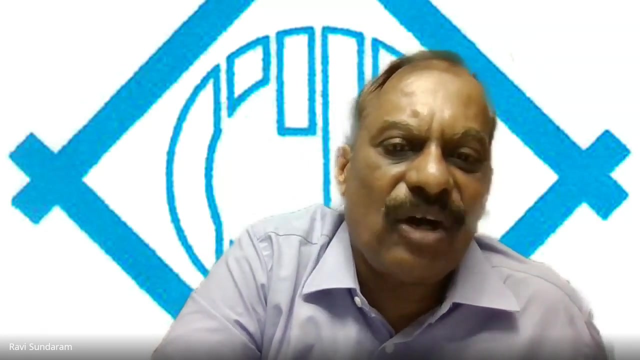 which are coming up with a large span, Similarly nuclear facilities which are very heavily loaded. you may want some of the parameters in the fractured rocks, in the hard rocks And for normal kind of buildings which are maybe 10,, 15 stories. 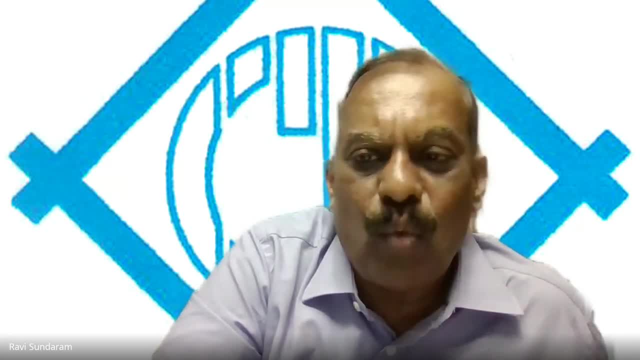 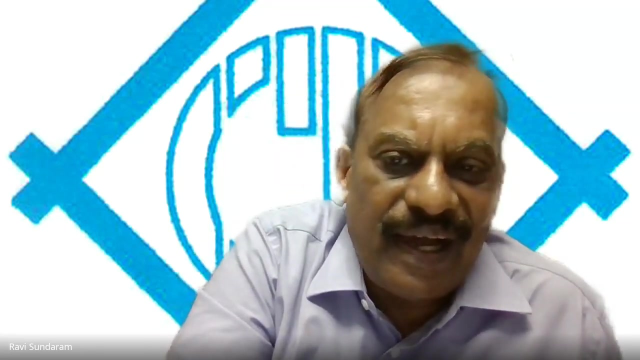 it may not be required, But you have to carefully look at what your application is And if you are going to have a bridge across a river like Brahmaputra, where the currents are very high and the water depth is also substantial, you could have very high stresses in the rock. 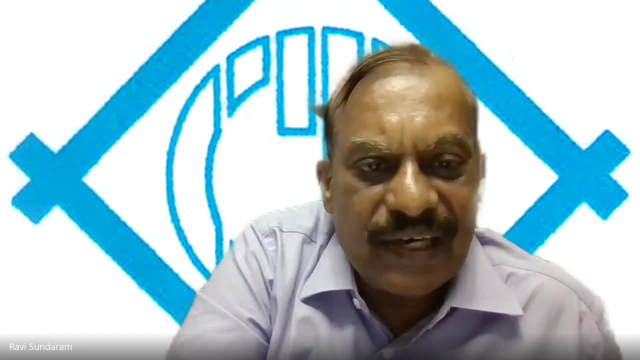 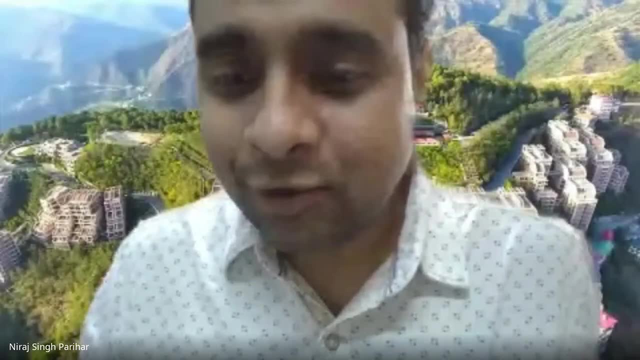 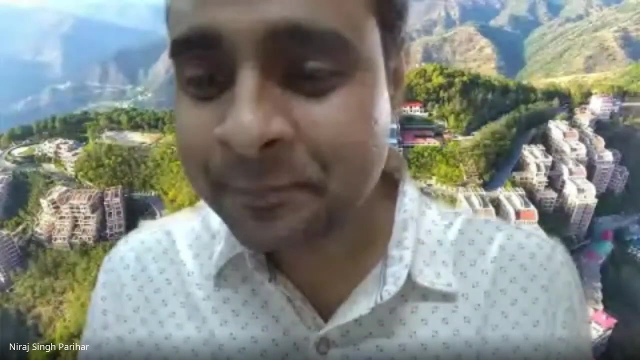 if you are having a pile or a well foundation seated in that rock. Thank you, sir. There have been a lot of comments. People really liked your lecture And lot of had commented nice and very informative presentation. There are a few more comments now. 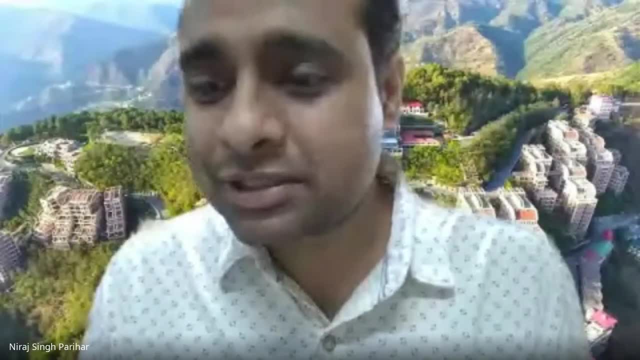 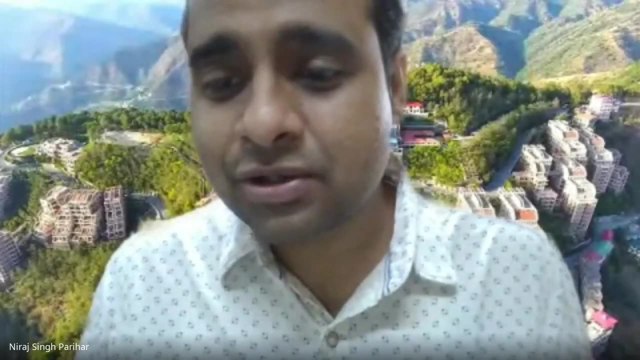 Dr Chayan Gupta Namaskar. sir, First of all, very congratulations to the team for arranging such a nice session. Thank you, sir. Sir, I want to know which type of tests are supposed to be used in soil having fractured rock on shallow depth. 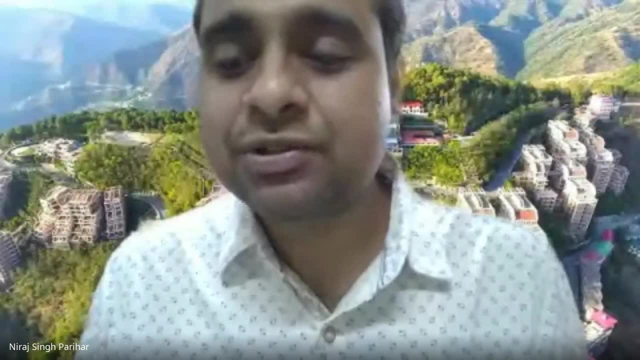 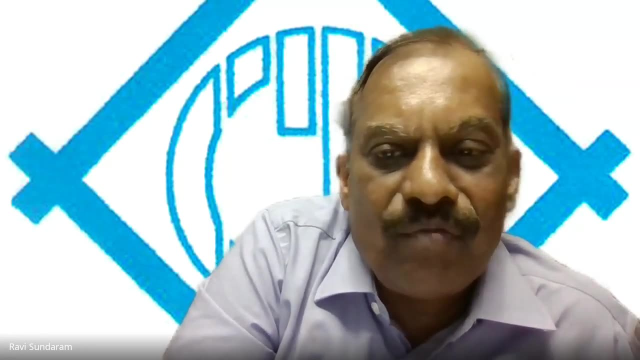 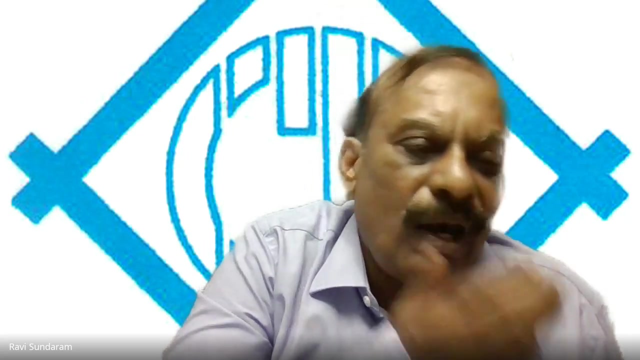 It is possible to apply SPT test on that situation or not. In a rock- fractured rock- you would usually get a SPT value of much greater than 100. It will not give you very good results. What I would suggest is that. 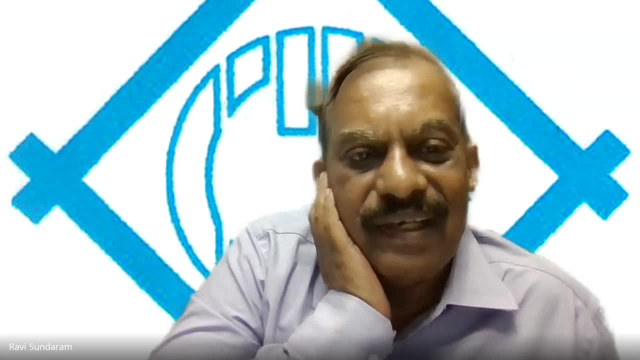 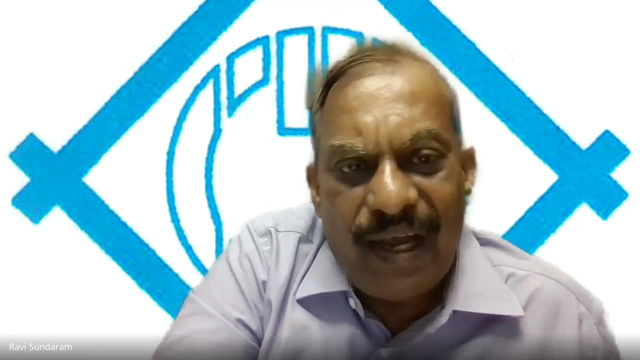 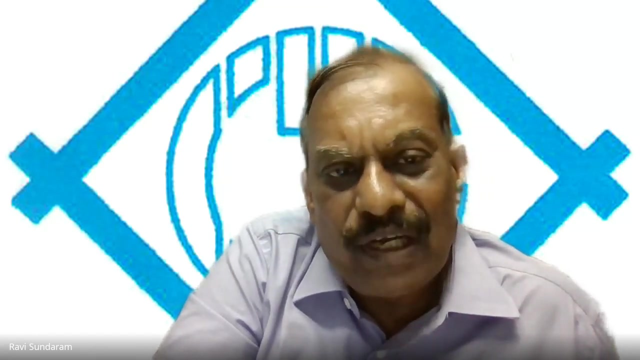 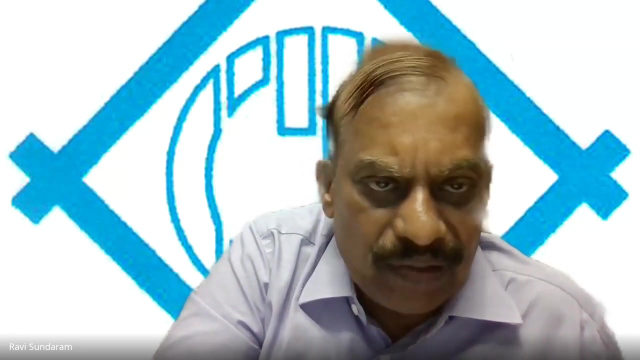 you should go in for drilling with triple tube core barrel so that you get a good recovery of the rock and then you know what kind of jointing is there. Seismic refraction test could also tell you to what depth the rock is fractured and below what depth you are getting stronger rock. 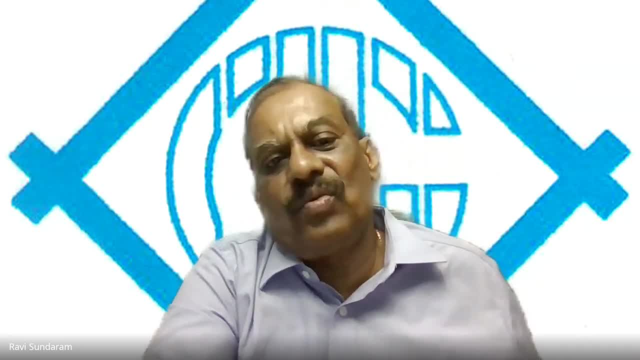 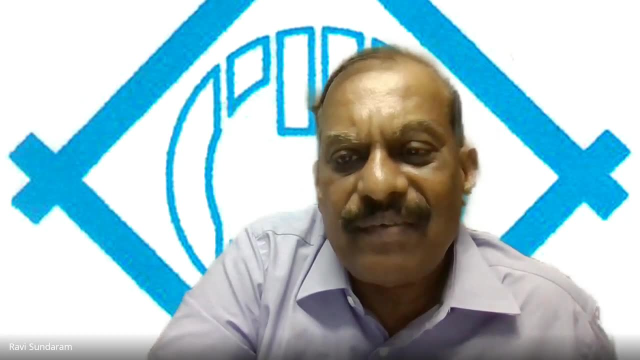 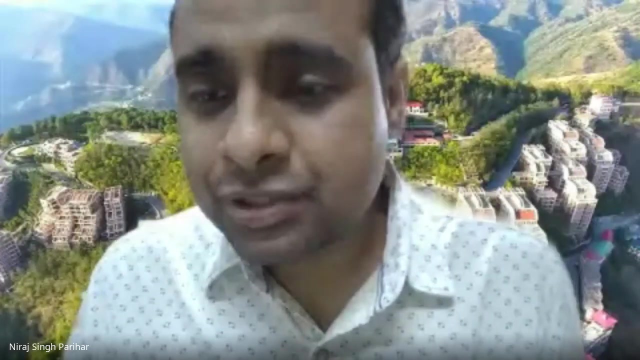 And then, of course, it is not just the strata, It also depends on what you are constructing on top of it. So, depending on that, the various testing scheme has to be worked out. Okay, sir, There is another question from Amik Kumar Mandal. 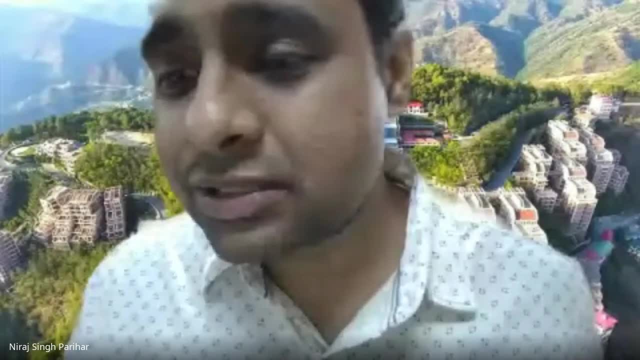 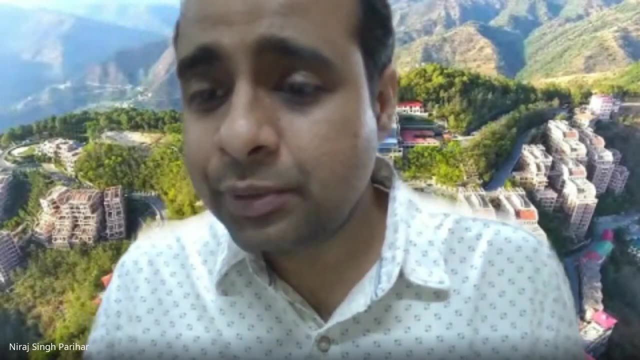 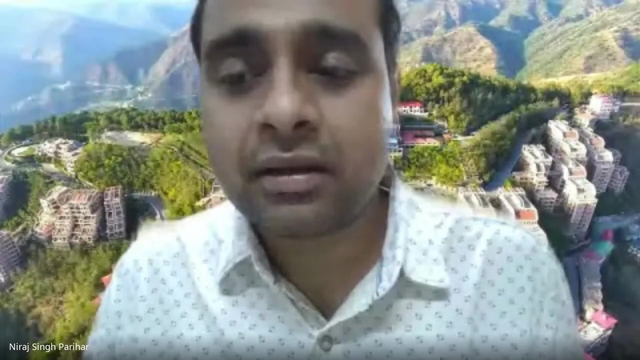 Very informative, comprehensive and useful presentation. How does to get the in situ shear strength of the hard clay with SPT more than 30 foundation strata, as the UDS is not usually not collected due to the occurrence of disturbances while sampling in the hard clay strata? 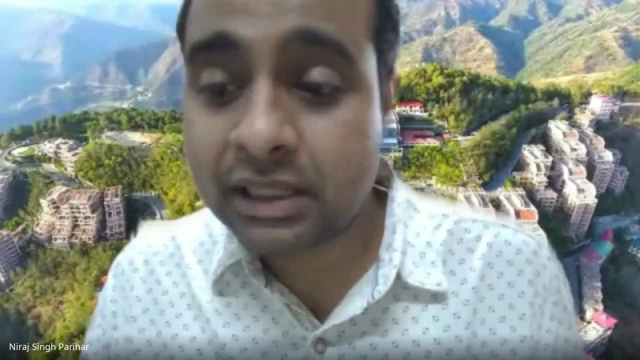 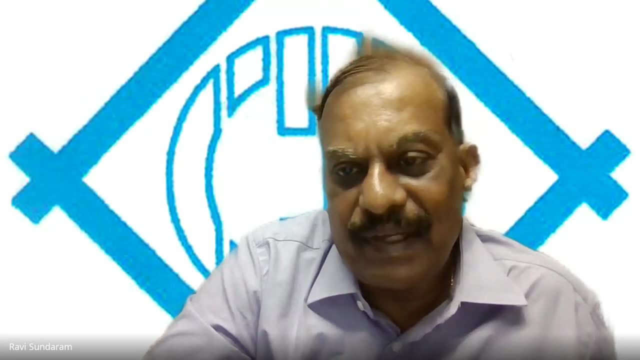 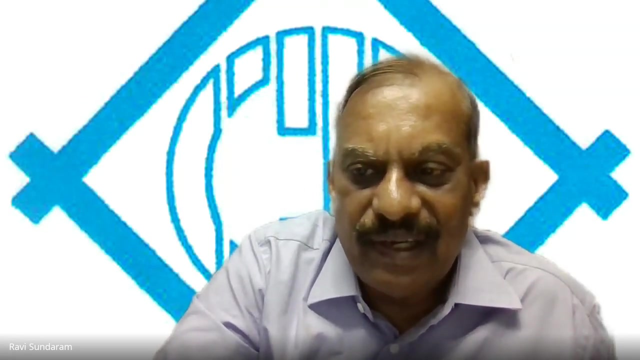 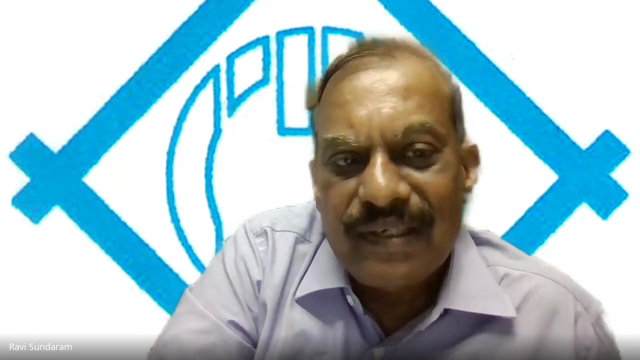 Can the pressure meter test or any other suitable field test can be done in this case? Please discuss: Pressure meter test is the ideal test for this application because pressure meter test is going to give you very confirmatory parameters. from the there are correlations available. 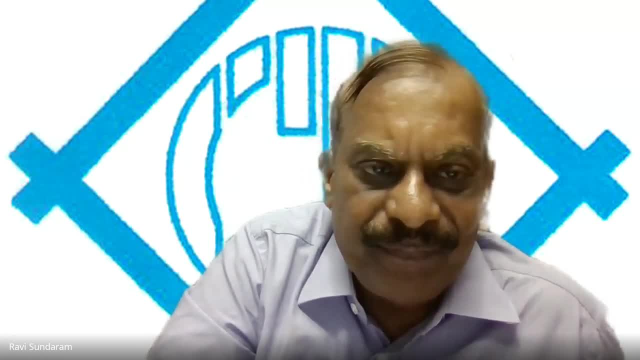 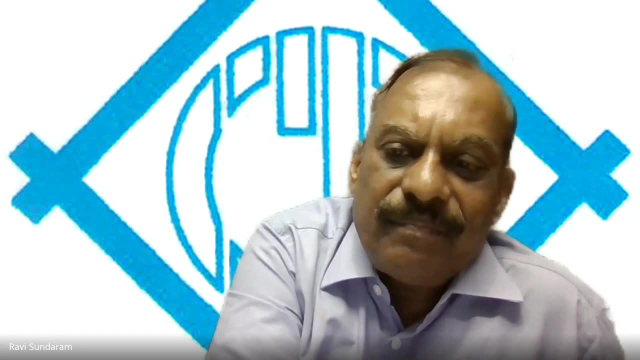 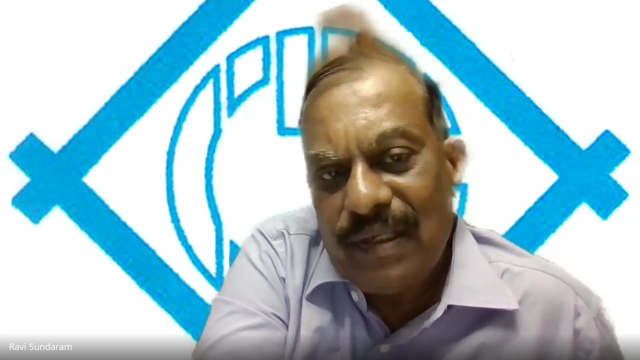 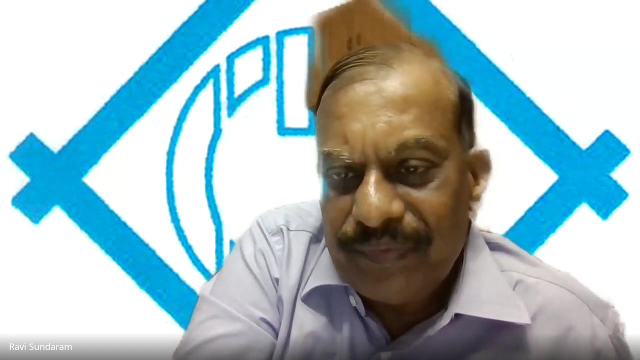 between the limit pressure and the shear strength of the clay, And these are very well published and documented. So once you know the limit pressure and the modulus of elasticity, you can work out the shear strength, You can work out the over consolidation ratio and all these other parameters from the pressure meter test. 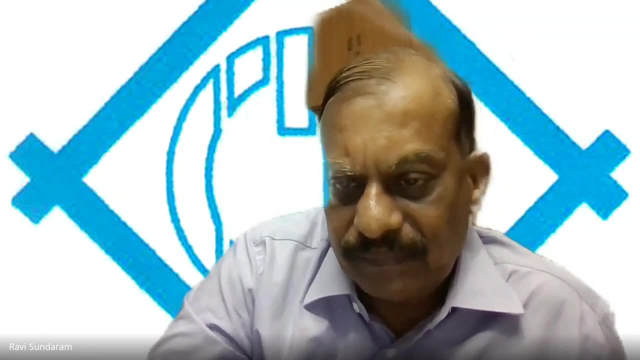 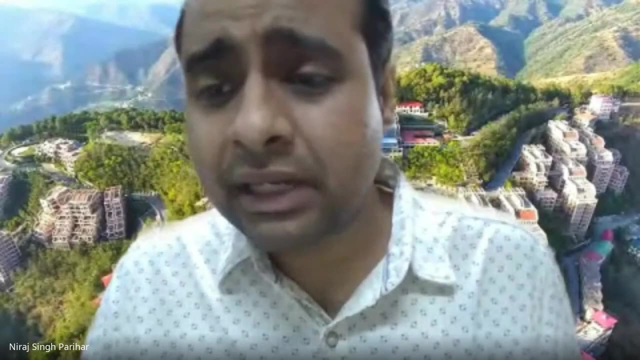 It's a very useful test. Okay, I hope that will solve the query. There is another one from Sudhir Bhatsi. He is asking that resistivity may vary with moisture content and should be specified with it. Please clarify. I agree with you. Resistivity will vary with the moisture content and the season during which you do the test matters, because in the dry season you could have high resistivities and during the monsoons, particularly the surficial soils could have a lower resistivity. So you have to interpret it. 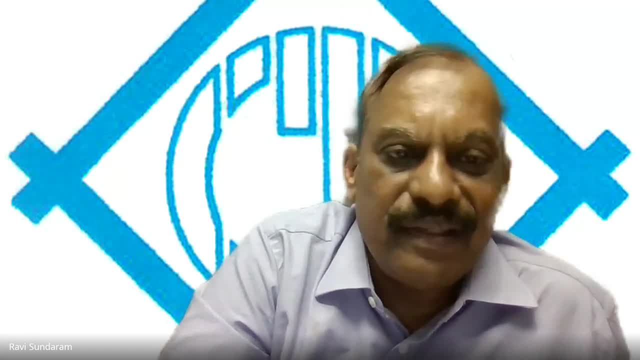 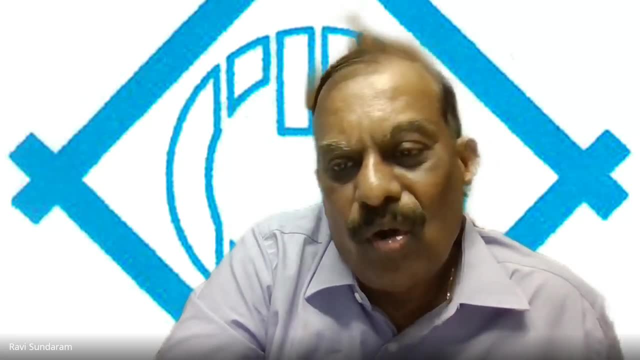 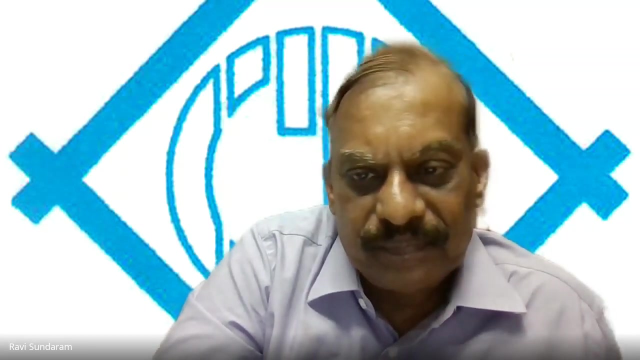 considering the level of the water table, because you would have to do it along with boreholes, so that you know what the borehole data is and how you can match the resistivity data with it. Okay, sir, Sir, I think that's it. 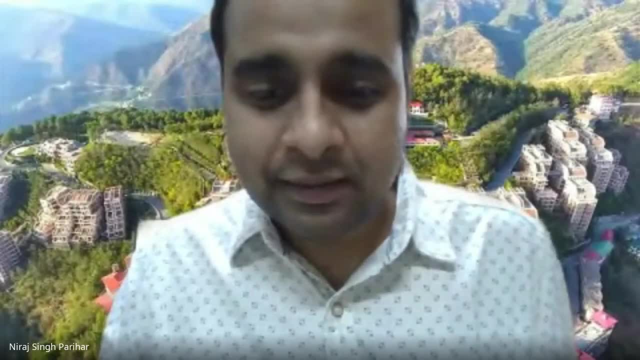 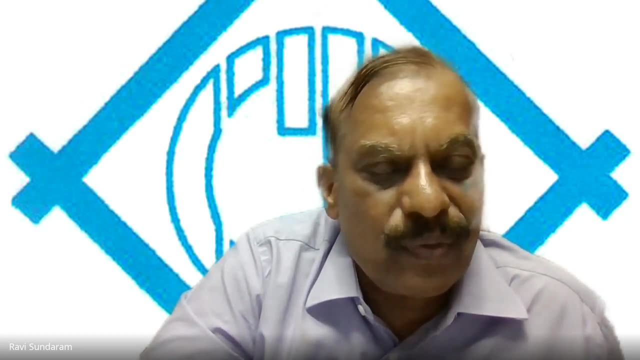 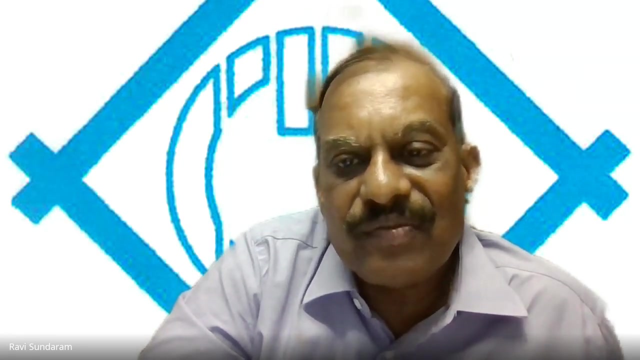 We are done with the question and answers. Okay, so the next presentation will be next Saturday, in which cone penetration test will be discussed in detail. So each of these tests, actually, what I have given today is just a brief introduction and just try to explain it. 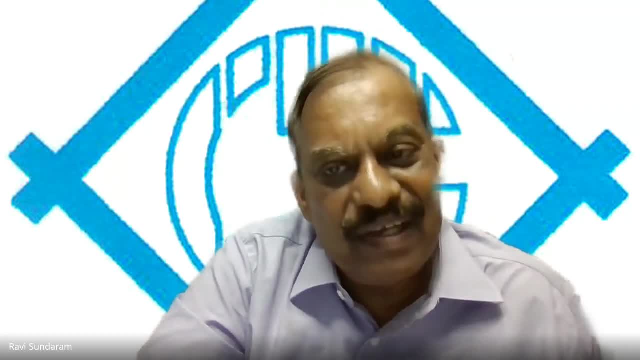 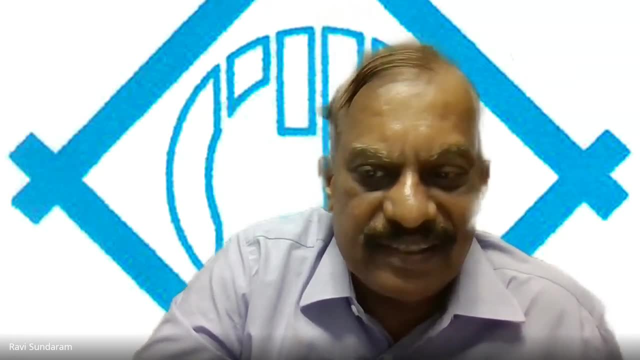 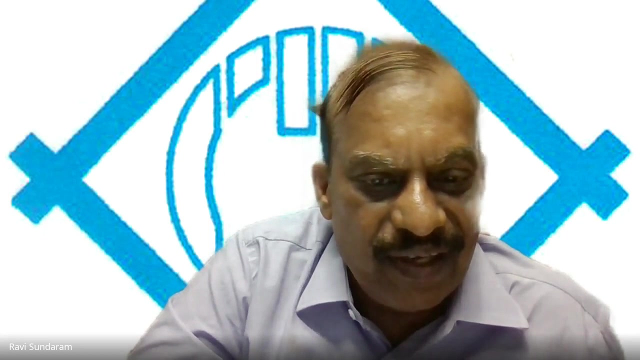 Just try to tell you that these kind of tests are available, and you would have to do a little bit more study on each of these tests to be able to, you know, figure out where it is applicable and how best you can do it. That's about all I have to say. 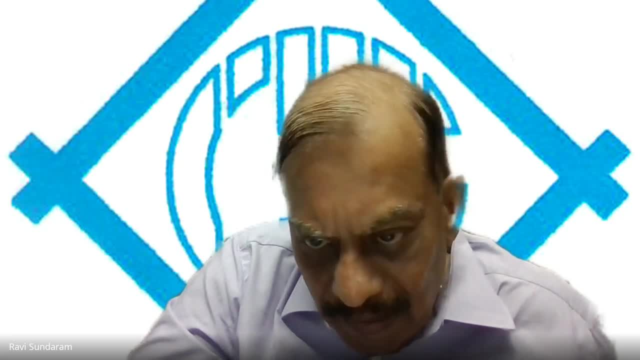 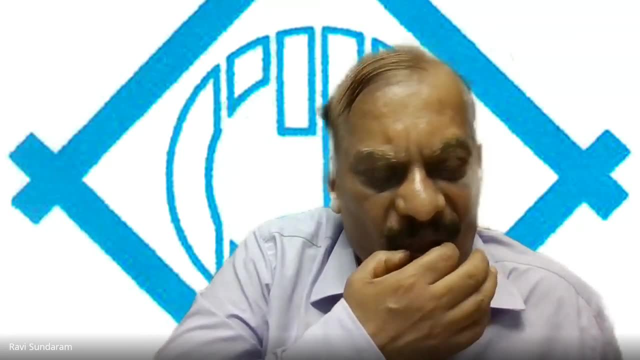 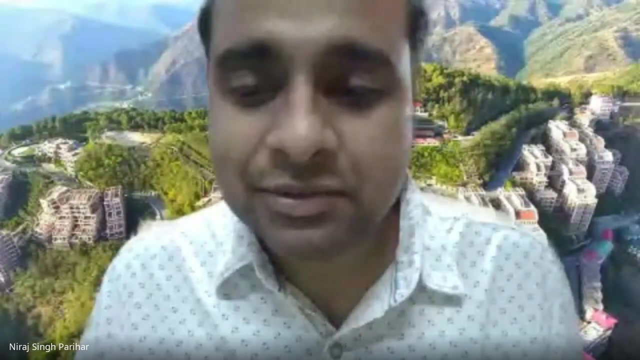 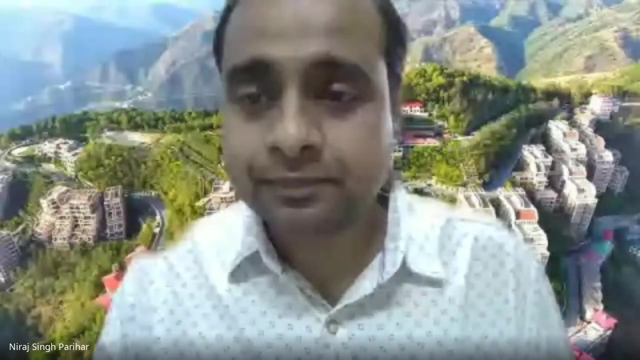 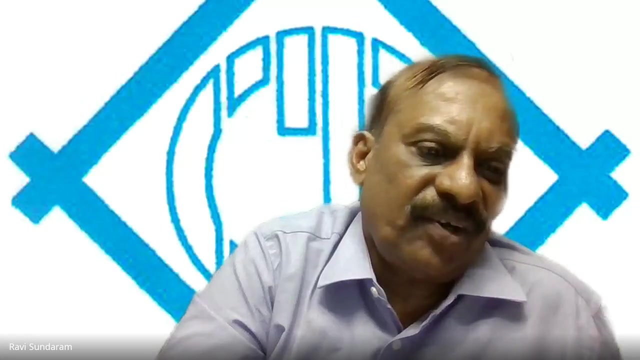 I see Pravaram Panda has raised his hand. if there is anything which you would like to say, So any of the participants want to ask the question, they can kindly unmute themselves and directly ask the question. Sir, I don't feel there are any left. 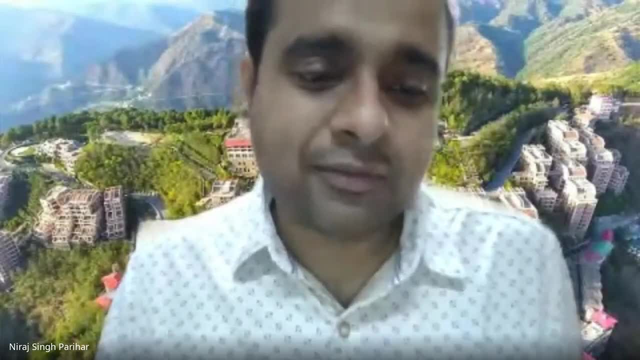 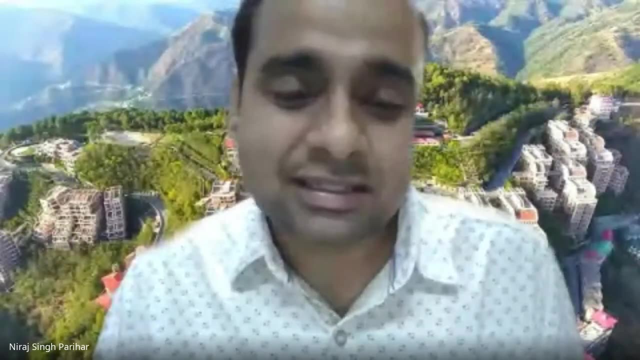 Okay, Sir. with this, I would like to thank you once again for your kind gesture, sir, and with all your support, it has been possible to organize this entire lecture series, And we are also grateful to you that we'll be meeting you once again. 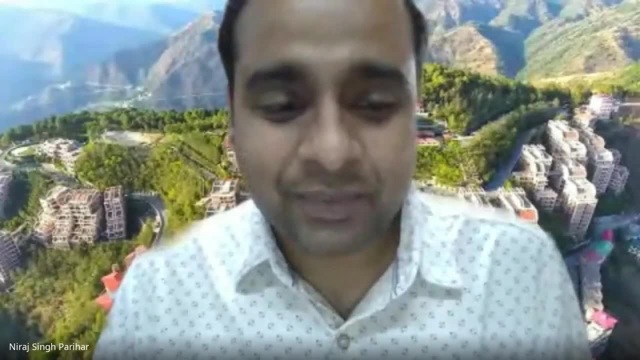 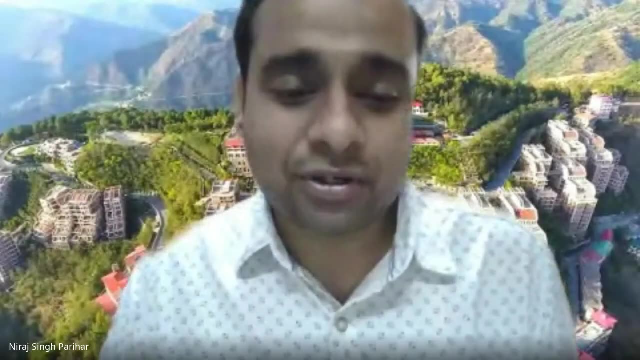 on 10th of October, 3.30 pm, And we'll be continuing with this lecture series, So next lecture will be on next Saturday, given by Mr Saurav Gupta, Managing Director of Singers Geotechnical Limited, on 25 September, from 3.30 pm onwards. 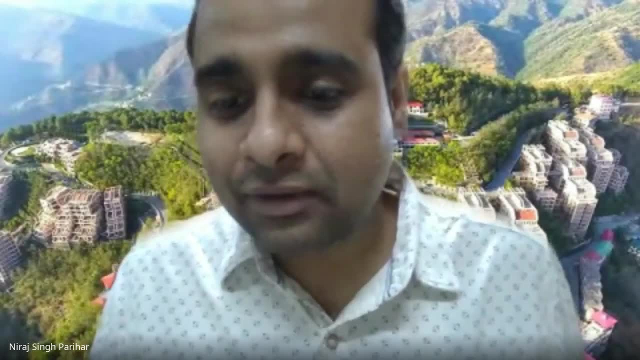 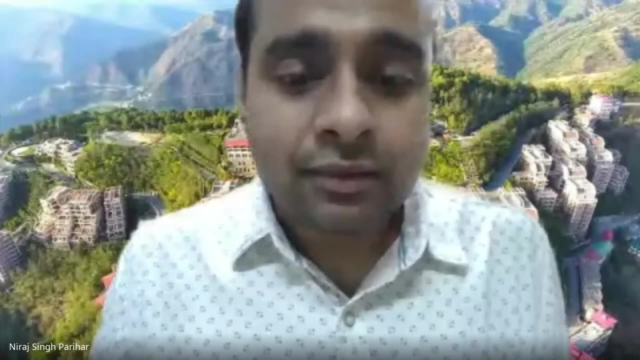 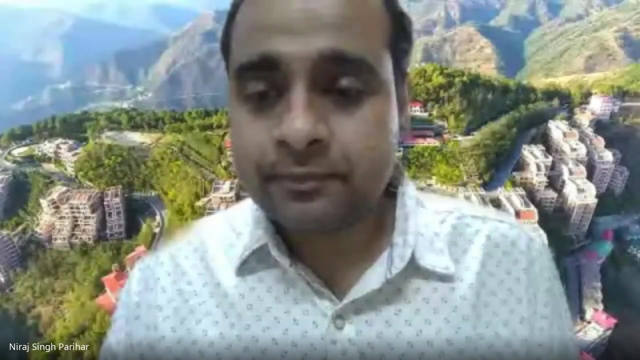 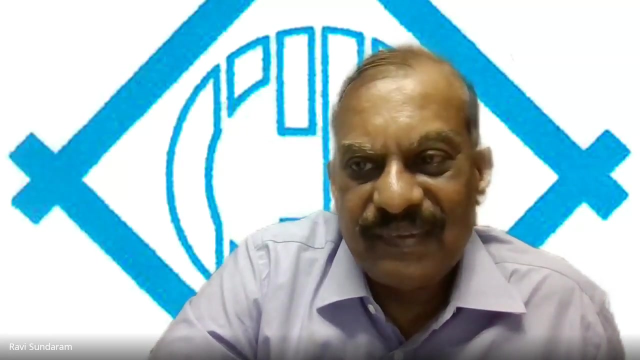 And I would also request all the participants to please fill out the feedback form before leaving. So thank you to all the participants. Thank you, sir, And thank you sir. Thank you, sir, Really very grateful for all the this great gesture. 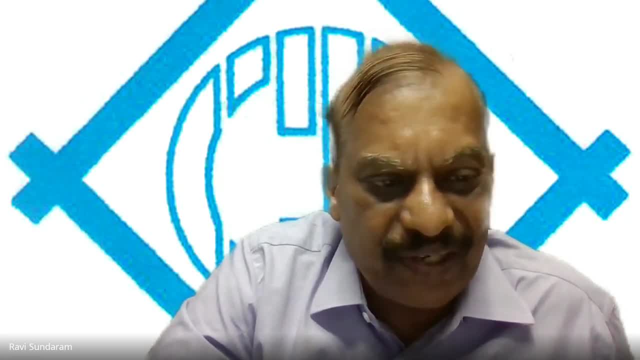 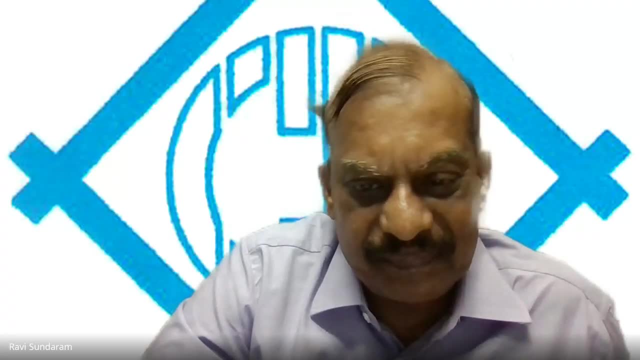 With your permission, now I would like to leave the call. Yes, sir, surely? Thank you, Thank you very much. Thank you, sir, Thank you very much. So thank you to all the participants. We hope we'll be joining again with us. 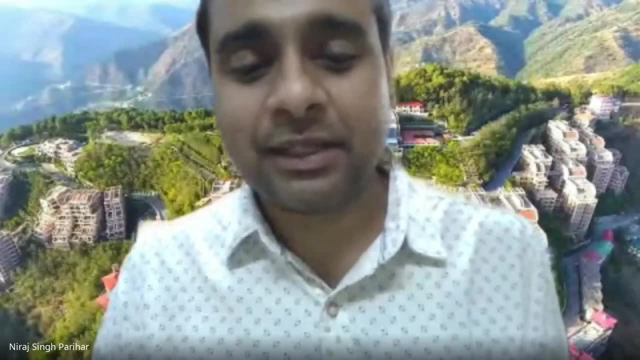 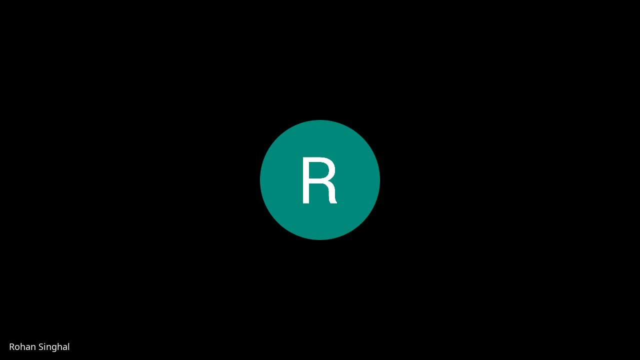 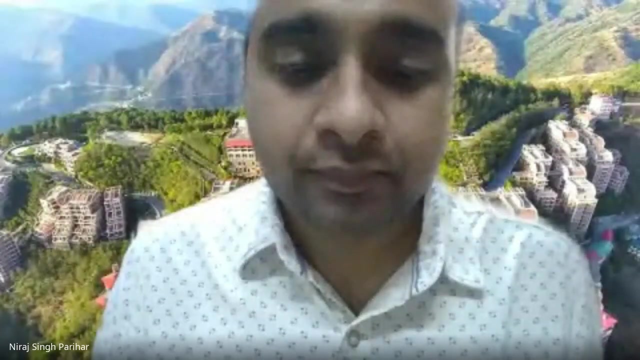 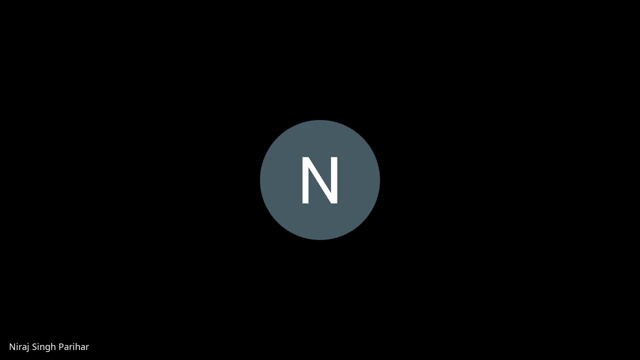 on the very next Saturday at 3.30 pm. Please feel free to contact us in case of any query. We will be happy to help you. Thank you, Thank you everyone. Thank you. We have more questions for Alan. 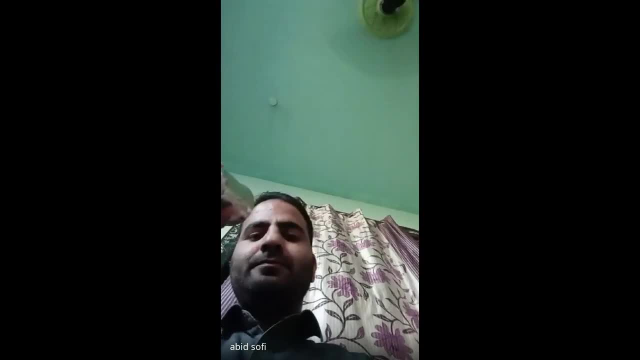 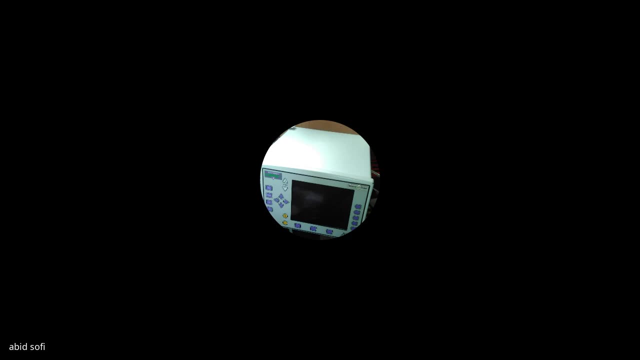 Alan Alan Alan. We have more questions for Alan Alan Alan Alan. I'm sorry, I can't. I'm sorry, I can't. Alan Alan Alan.